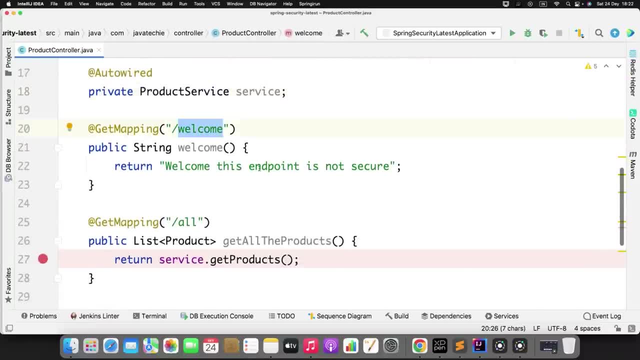 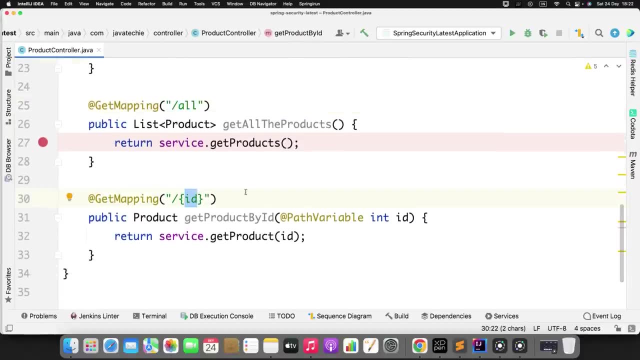 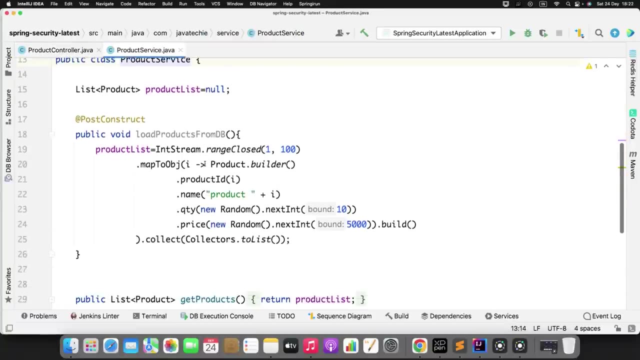 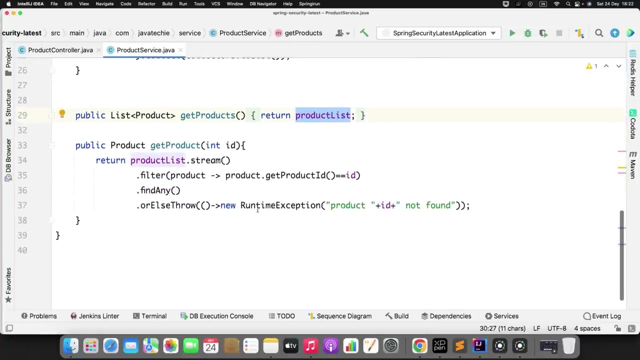 I have defined this for you. I have defined three: rest endpoint. One will print some string message and one will fetch all the product from the service. One will filter the product by ID. Okay, Now, if you go and set the service class, I am just generating hundred of product object using this int stream. Okay, So when I will call the serviceget products, I will return the list, And when I will call get product by ID, I will filter from the list and I will return the product object. 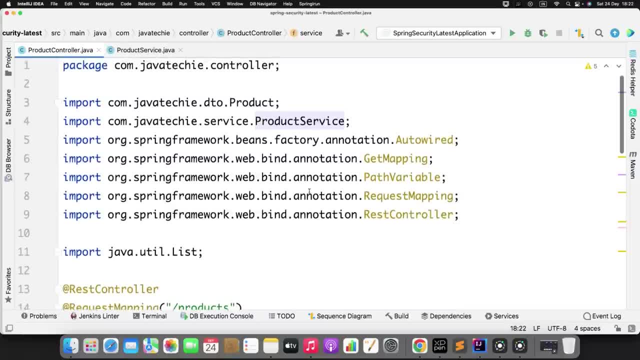 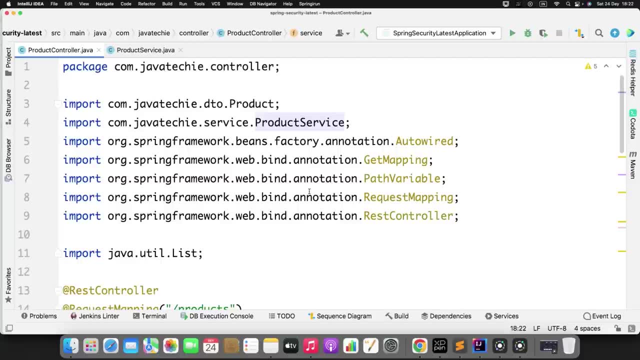 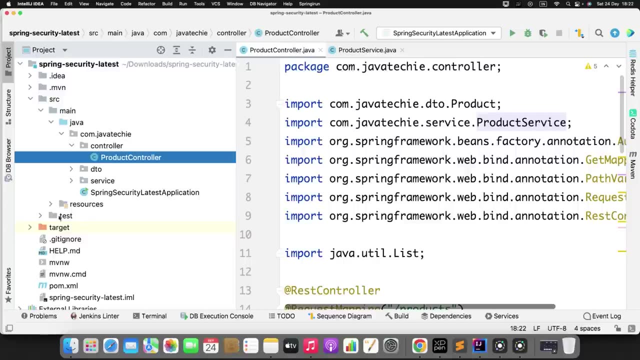 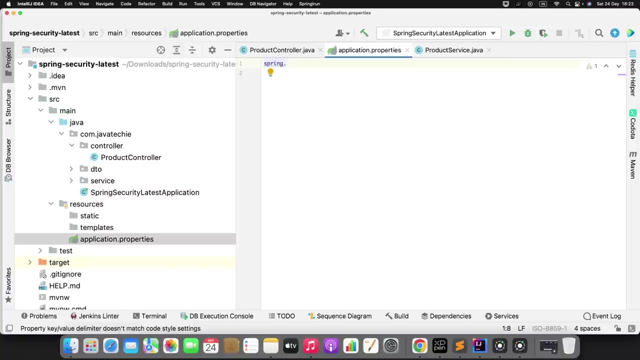 This is what the endpoint I have defined, but I didn't write single logic for security. Since we added the spring security dependency, by default in Spring Boot, security will be enabled. But if you want to configure your username and password for your testing what you can do, you can go to your resource application or properties file. Here you can define springsecurityusername. You can type security, Okay. So let me just 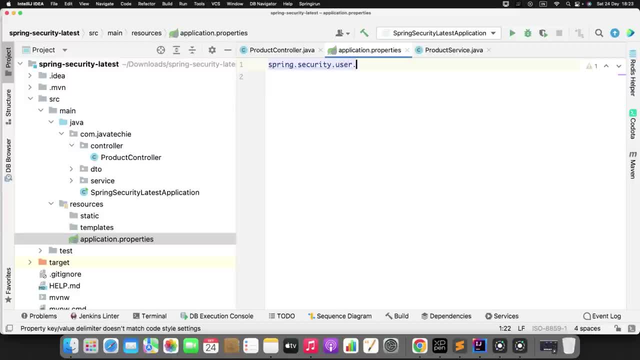 assume thisusername and then you can give your name. Similarly you can give the password. But this is not the recommended approach, since we don't want to hard code it and also we don't want to restrict with the one user. So here you can only define one username and password. So let's say username is basant and password is, let's say, pwd1.. Okay, This is the username and password. 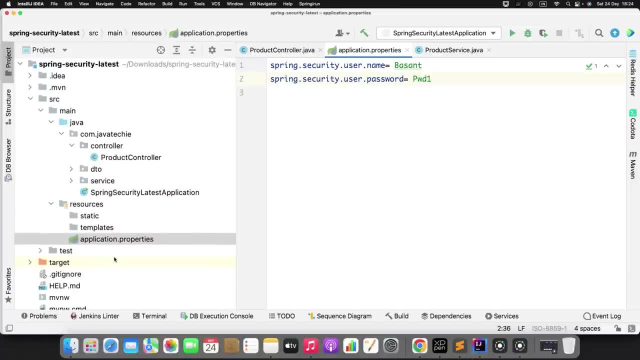 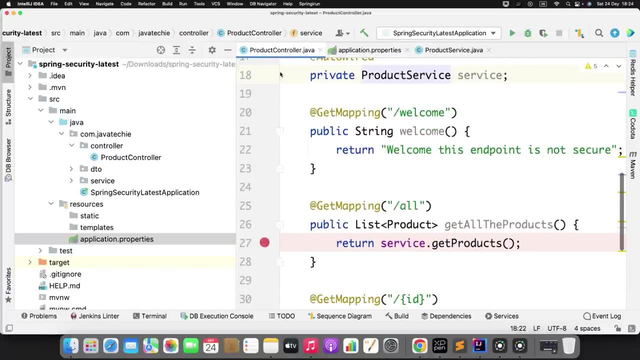 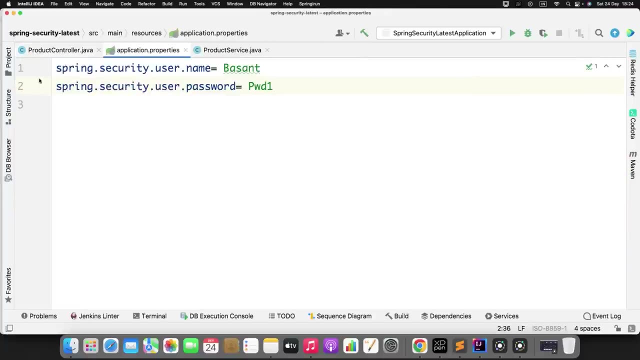 Since I added the spring security dependency, by default, security will be enabled for me. Now I can access all these three endpoint slash, welcome slash, get all the products and filter product by ID with this credential. Okay, So let me start the app, Then we'll verify. So let me run this. 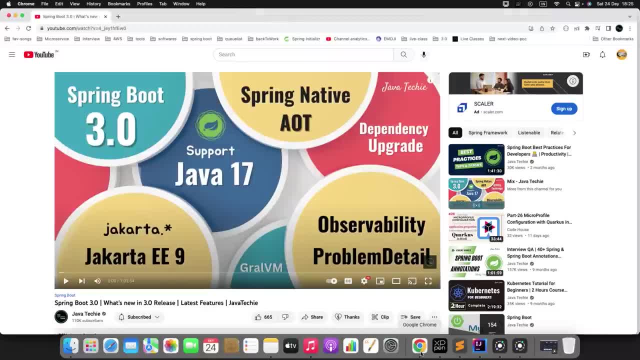 So application started on port 8080.. Now, if I'll go to the browser, If I'll go to the browser, I'll get theation. If I'll go to the browser, I'll get theation. So let's go to the browser. 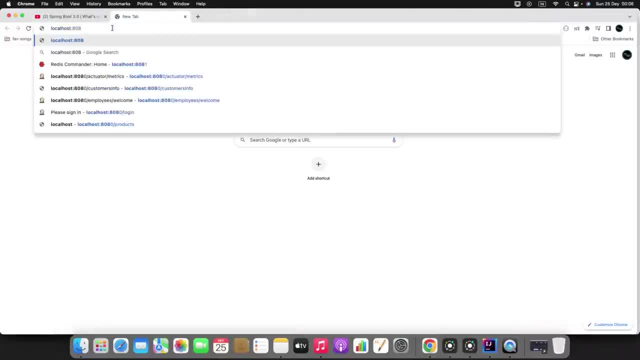 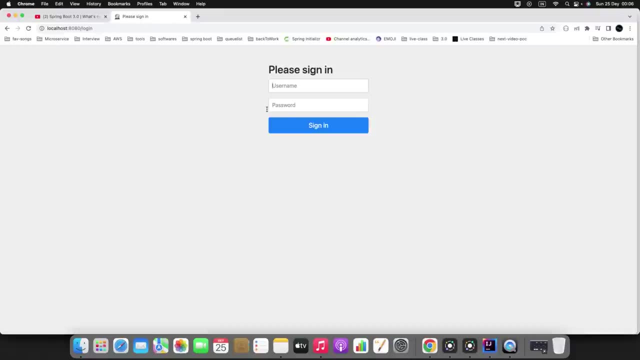 If I'll go to the browser. If I'll go to the browser. If I'll go to the browser, hit the endpoint: localhost 8080. slash products- slash- welcome. I need to pass the username and password which I have configured in my application, or. 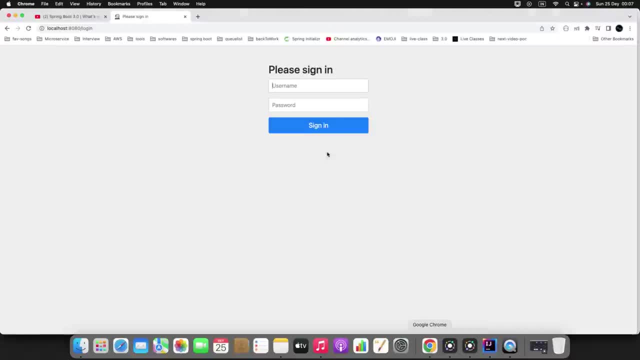 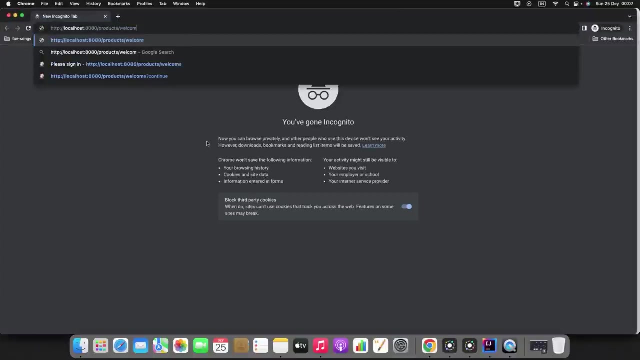 properties file. so if you will go to the browser, I configured Basant as a username and password as a PWD one. so if I will send the request, I can see the response. okay, similarly, if I will try to access other endpoint to get all the products and to filter product by ID, I will just open a new tab. I will just. 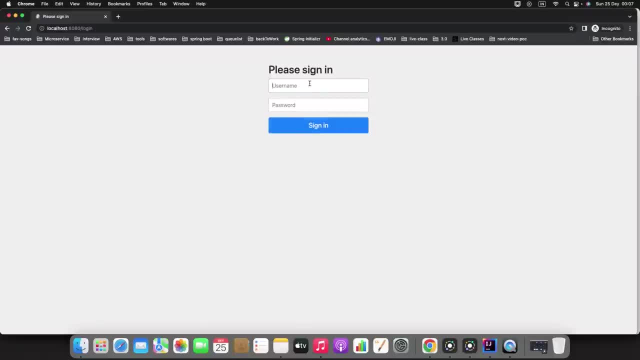 change here. all it will ask me credential, since I configured username and password as a Basant and PWD one I can able to access with that. only let's say I will give something PWD or I will give some random password. so it will fail bad credence in. okay, if I'll give Basant and if I'll give the PWD one, I 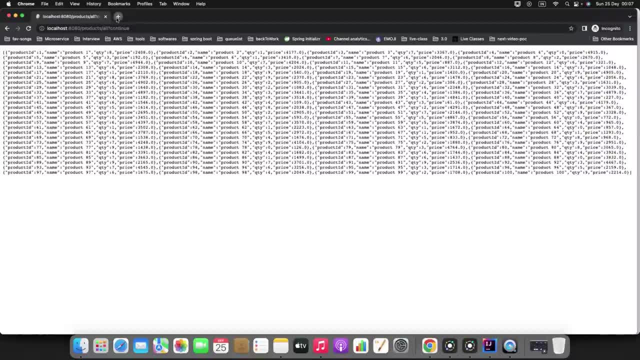 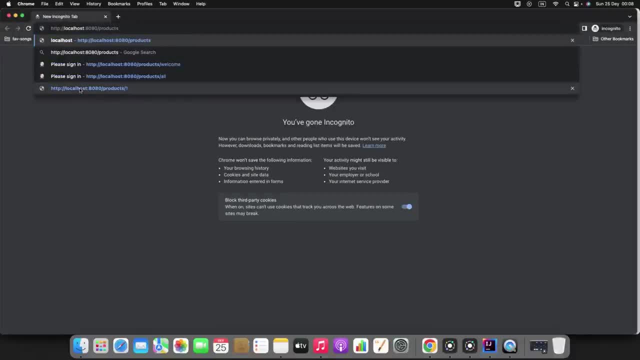 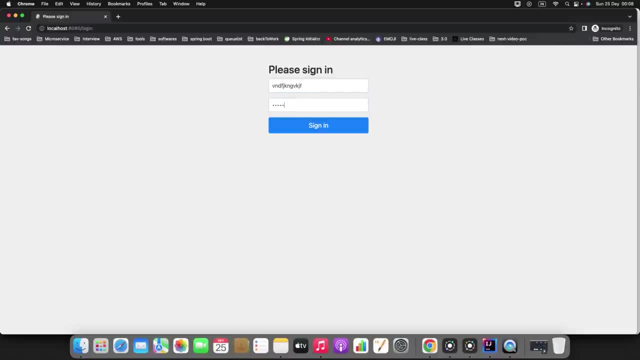 can able to see the response. similarly, if I'll try for other endpoint command, shift n, which is get the product by, I derive one. so it will ask me the credentials. if I'll give something wrong I will get the bad credential right. so I must need to, given what I gave, as it will give the credential for a particular, I will just open that so I will feel that bad credential so i must. 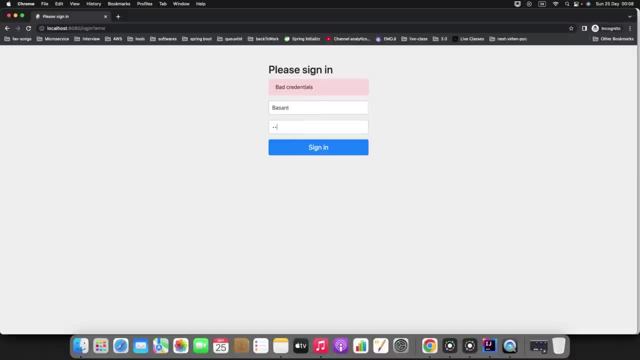 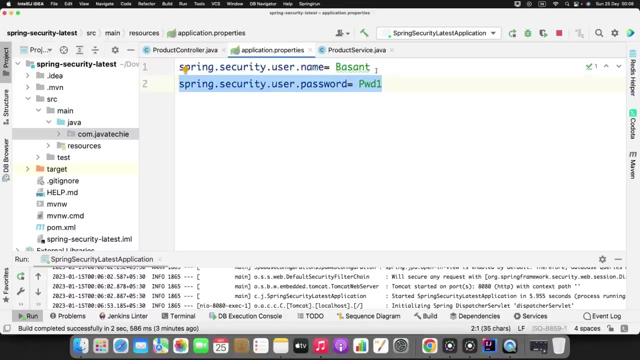 net to, given what i have defined in my properties file, pwd one. i got the response back. okay, so this is how you can use the uh credential or you can hard code the credential. this is for testing purpose in real time. we cannot hard code more than one user in application or properties file. 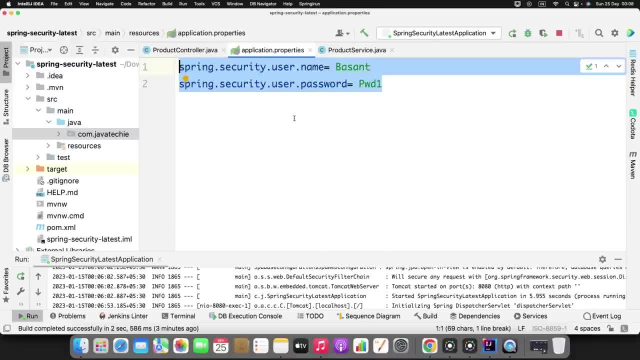 for quick testing. this approach is good. but what if i want to configure multiple user with different kind of role? where do i need to configure that? so, for that, you need to create a config class and you need to define your user detail service. so, for that, go to this package. 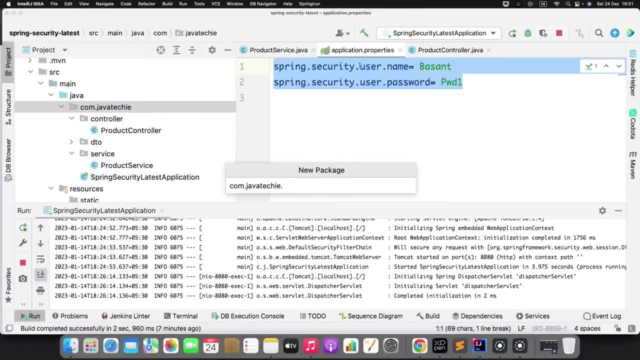 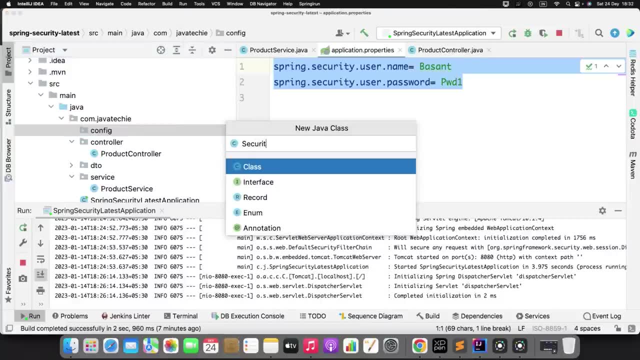 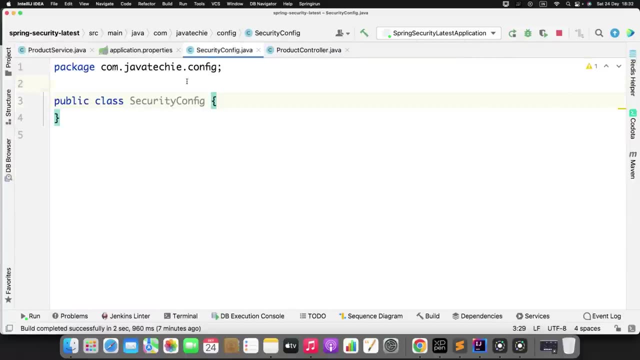 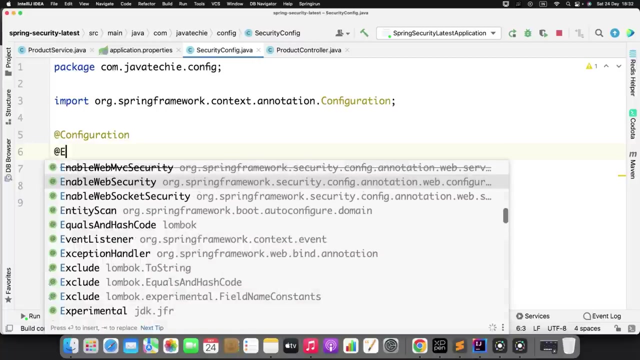 right click, then new packages, then i will just name it config. okay, so i'll just create a class, let's say security config. let me zoom this fine, so i need to annotate here at the rate configuration and since i am using web security, i need to enable that. 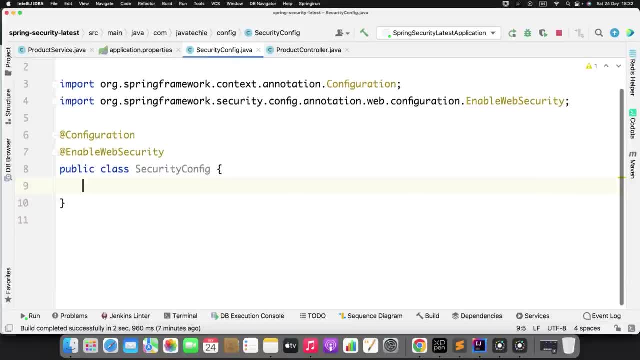 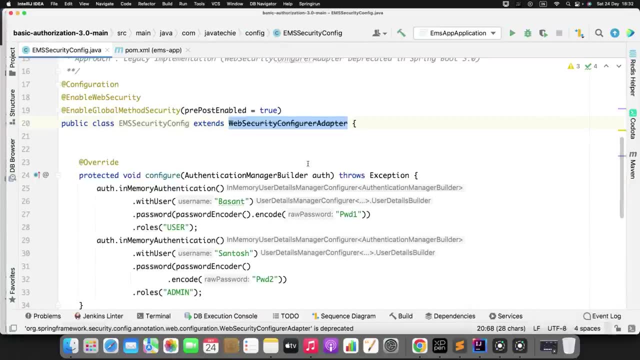 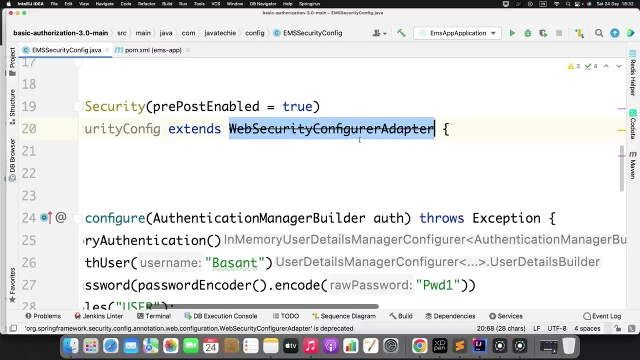 fine, okay now, if you remember, before springboot 3.0, usually we have something called spring security configure adapter. right, this is what the class web security configure adapter. this class is even deprecated in 2.7.x. okay, but what happened? what is the benefit we are getting from this web? 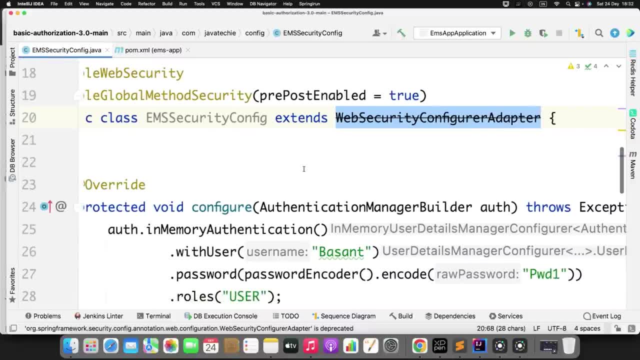 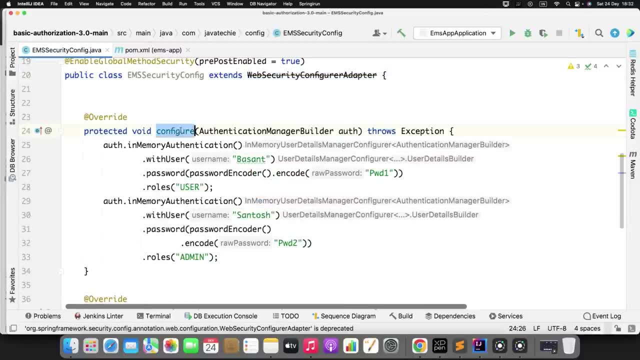 security configure adapter. usually it provides the three overloaded configure method. let me minimize bit so that it will be clearly visible for all it, given three overloaded configure method. first, configure method: you can have the argument authentication manager builder and you can provide your user details, user password and role right and 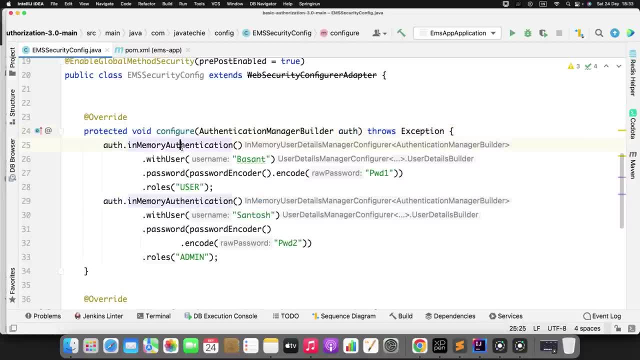 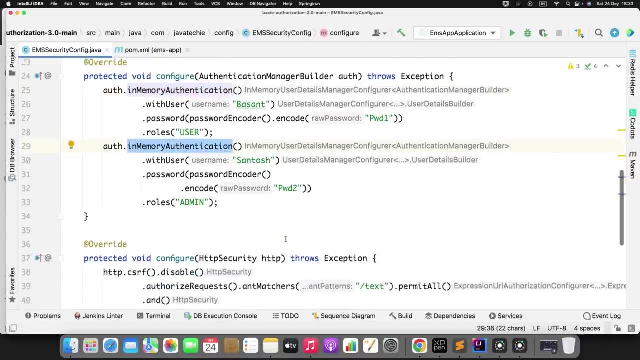 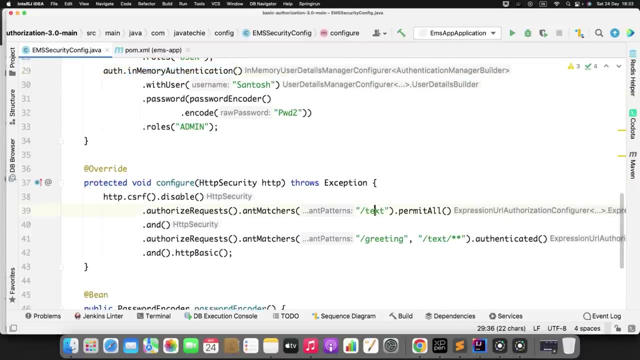 if you observe here you can configure n number of user, user 1, similarly user 2, with the having different role and different credential. and if you check the second configure method, you can have all your authorization related configuration here. what all endpoint you want to enable security or what all an endpoint you want to bypass without implementing. 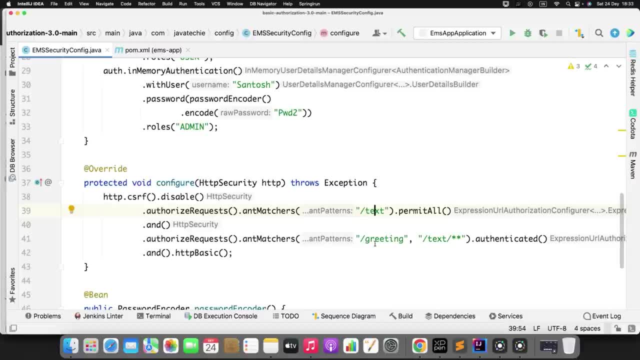 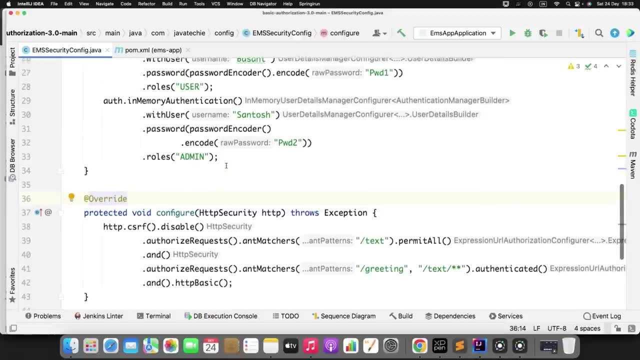 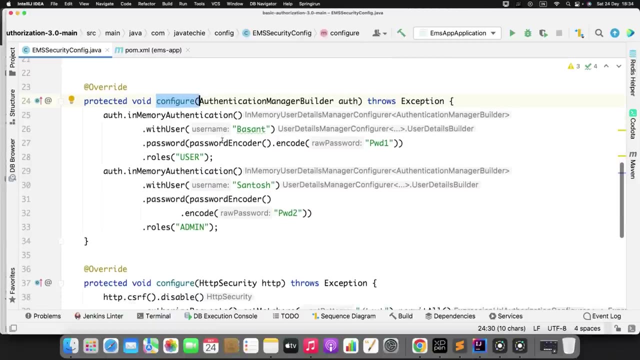 the security or you can define the ant matches for what all endpoint you want to authenticate that request. okay, so this part is nothing about the authorization and the first part- configure method- is nothing the authentication. okay, so these authentication and authorization to perform using web security configure adapter. it already given us the configure method, but now 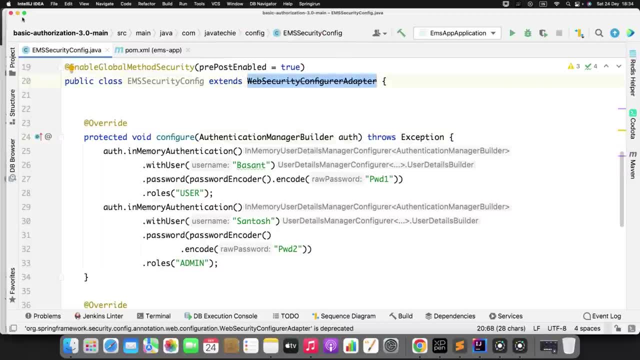 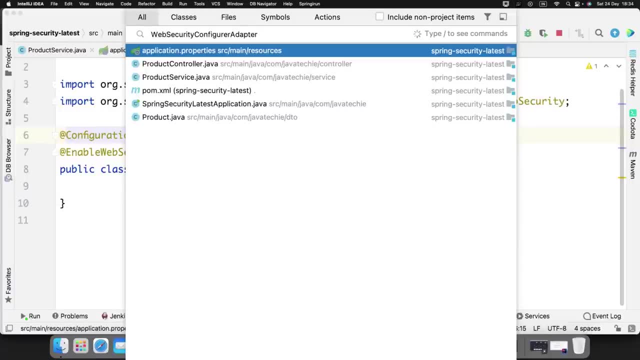 if you search this class, web security configure adapter- in your springboot 3.0 code base- let me click on double shift. if i'll just enter this configuration and you can, you can see that this configuration is not present. so you can see that we are not able to find this class in springboot 3.0. so they completely removed. 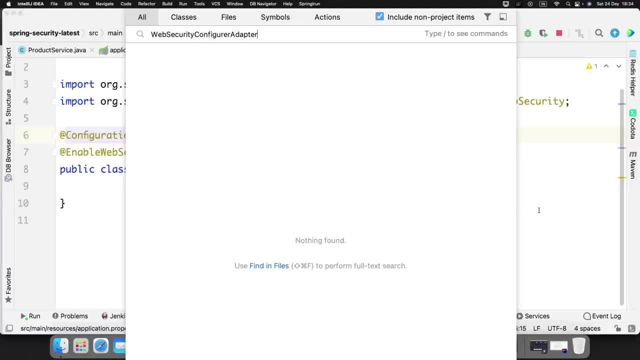 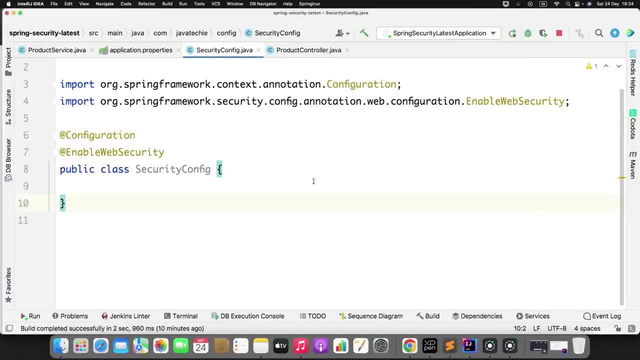 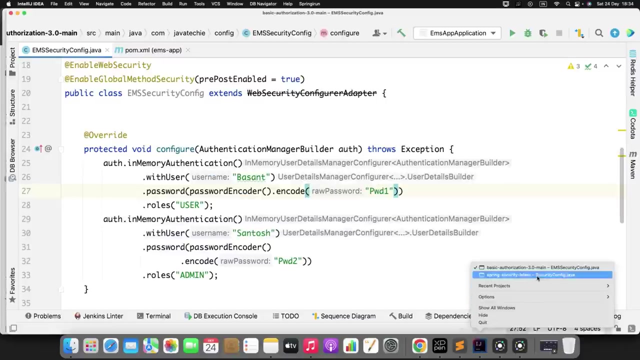 it. okay. so now, then, how can i configure the authentication and authorization without using this web security configure adapter? so for that, there are couple of new class introduced and the way we have configured before. i mean when i say before, this approach is completely changed. no overloaded configure method. now what you need to do? you need to create a bin of user detail. 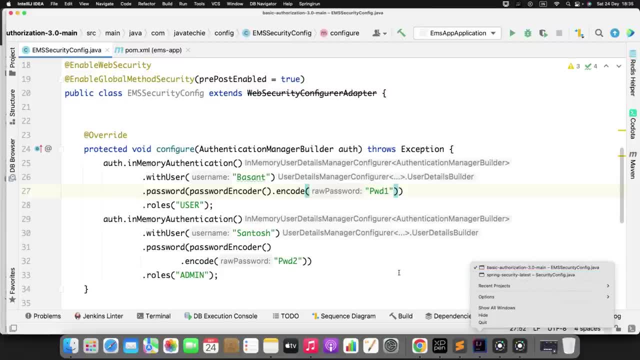 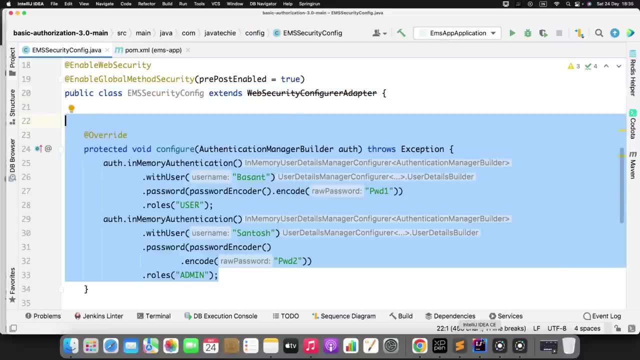 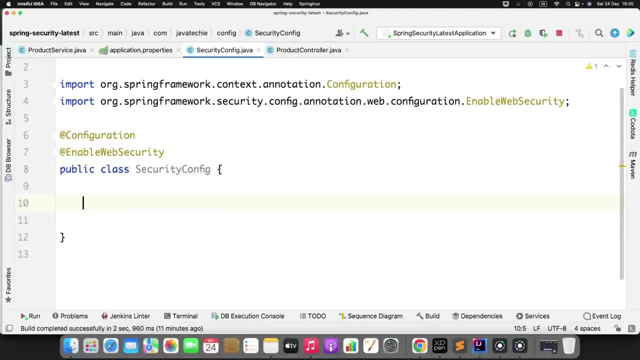 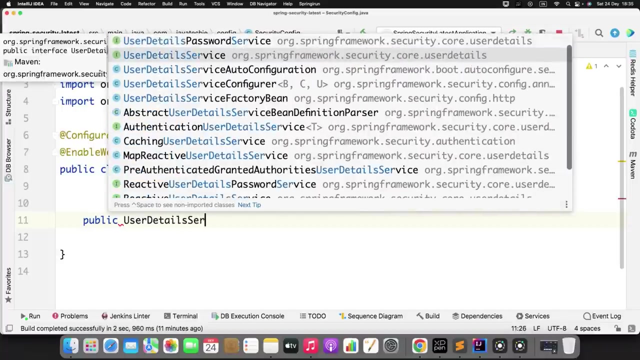 service to define the authentication related stuff. i mean these user details you can define by creating a bin of user detail service. so just go to the package. i mean go to the correct folder. now, here what you need to do: create a bin public user details service. okay, if you observe this, 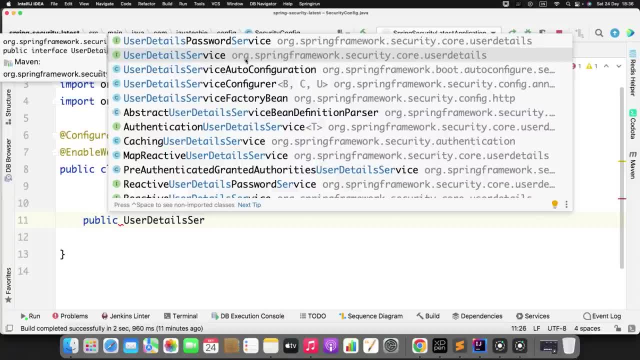 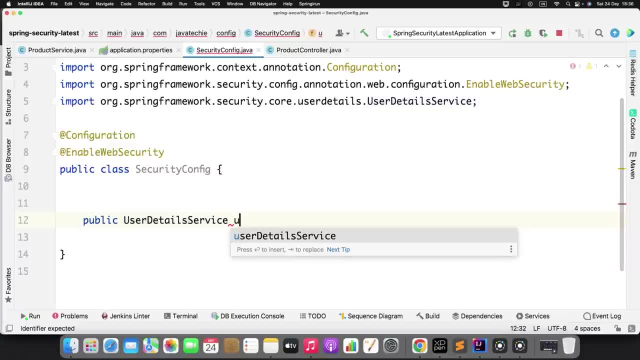 user detail service. it came from orgspringframeworksecuritycore user details. okay, so just use this service and you can name it user detail service, because, anyway, we are going to create a bin of it. okay, so i will just annotate here at the right bin now, here you can define as many as user details you want. you can define the same approach. 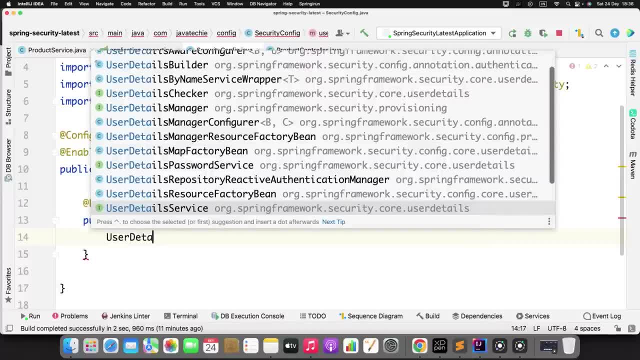 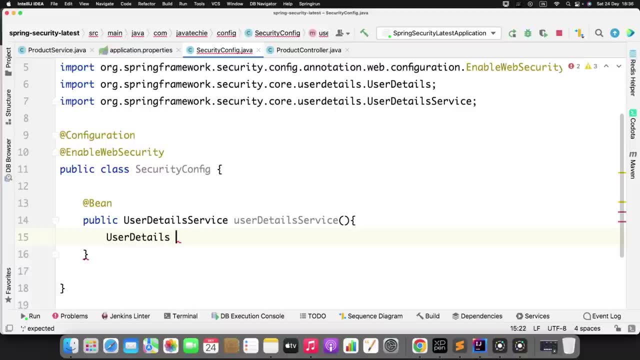 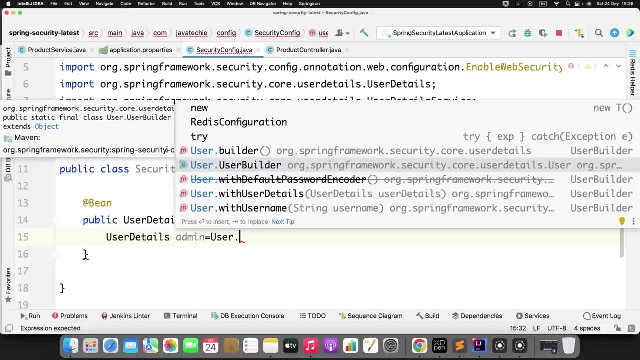 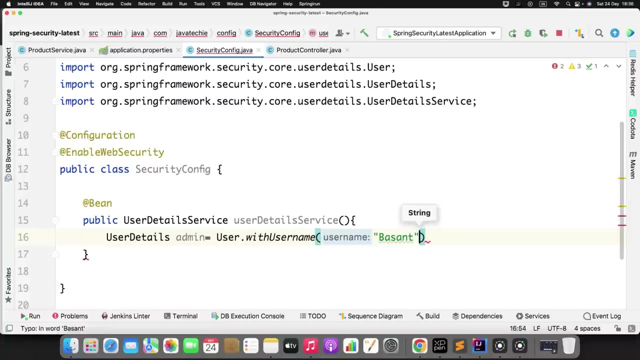 user details. let's say admin: okay, admin, equal to user dot. again, you can directly use with username what is the username you want to give. let's say dot dot, and i will also configure his password. let's say for now pwd1: okay, similarly, i can configure his role. 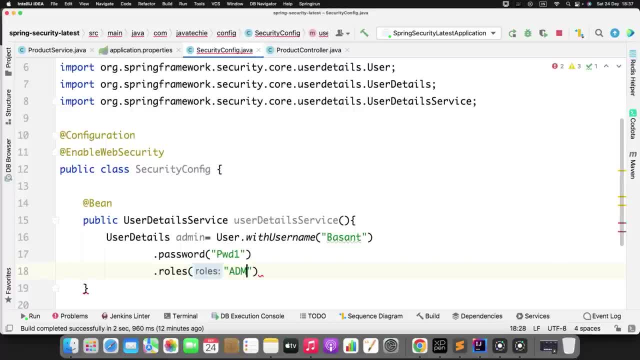 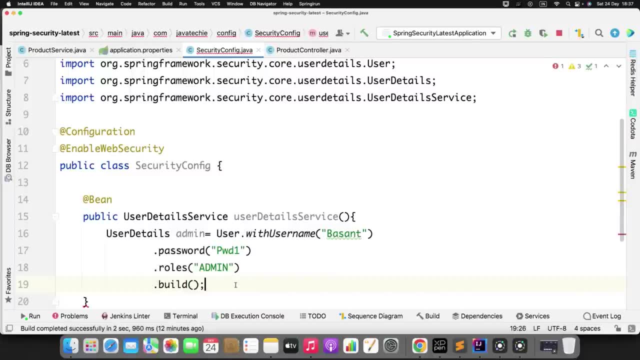 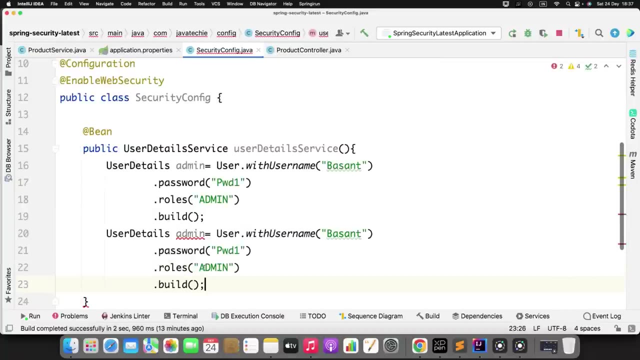 he is a admin. you can define multiple role for a single user and what else? just build that object, okay. similarly, i can define another user. let me copy this, so i will change the user to: let's say he is a simple user, okay, and i will give some name. let's say john. 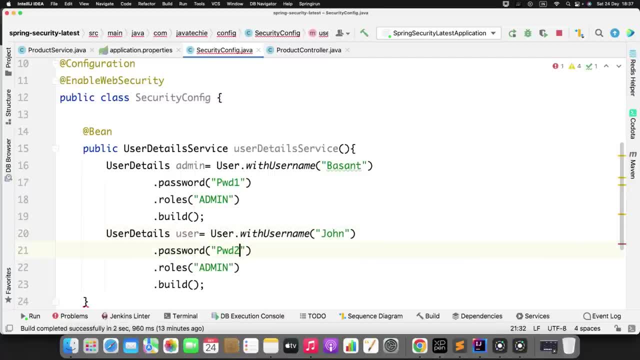 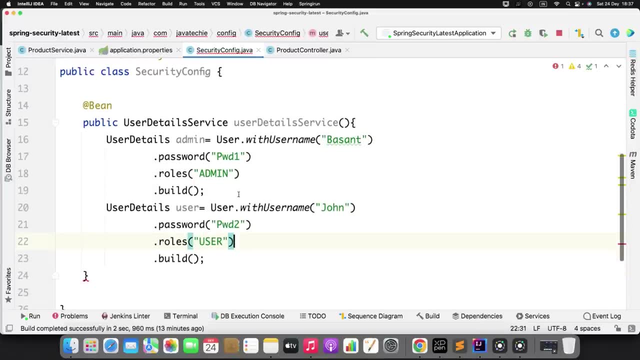 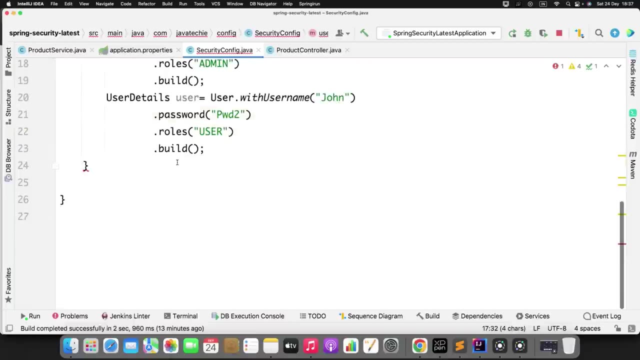 his password is pwd2. he is a simple user, fine, but it's not a good practice to keep the password in plain text, so i need to encrypt it. so for that, what i need to do i'll just create another user, another bin of password encoder. okay, that is also given by spring security: public password encoder. 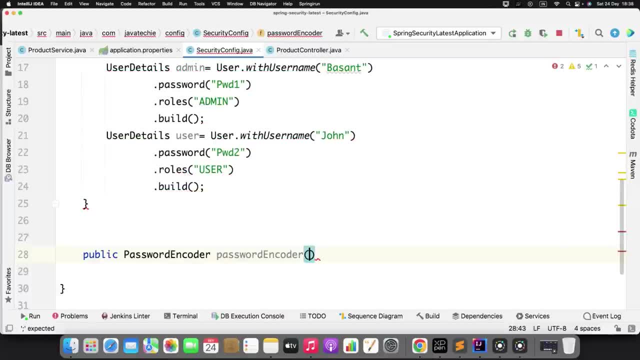 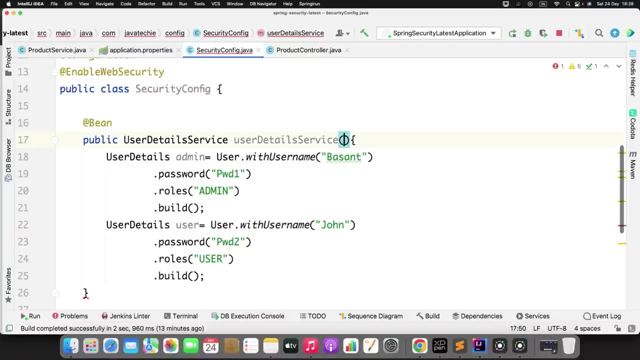 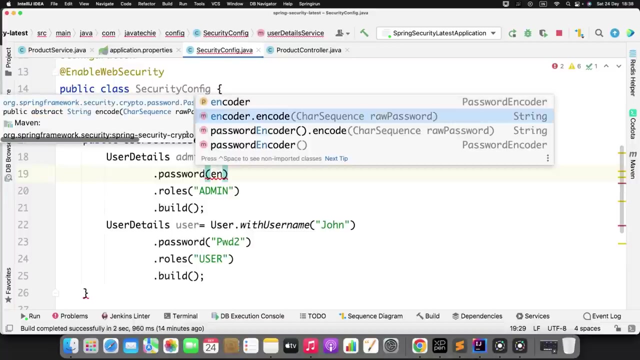 okay, password encoder, then i'll just use return new bcrypt password encoder. okay, i will also create a bin of it. then i can pass this password encoder here. i can define encoder now here, before i store the plain string as a password. what i can do, i will just remove this encoder dot encode the password. i mean just encrypt it. 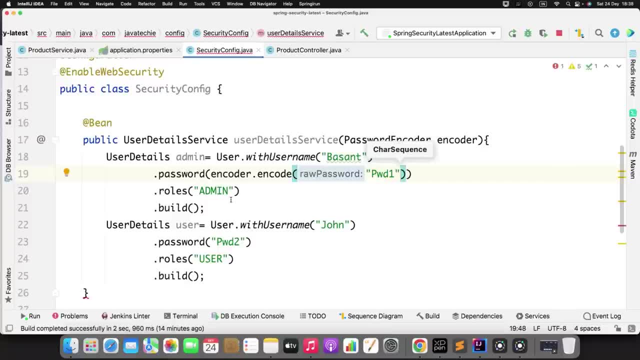 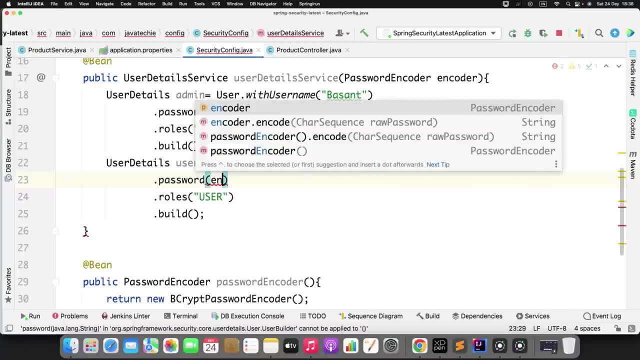 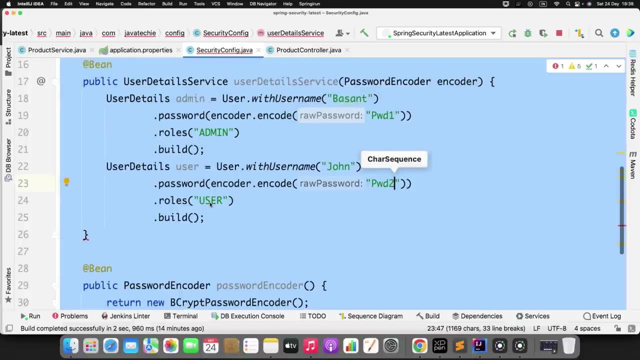 okay, similarly here also, before i store it, i can encrypt it, encoder dot, encode the password and give the password. that's it. okay, now, since you have two user, and currently we are hard coding- we are not connecting to our db to load the user i need to. 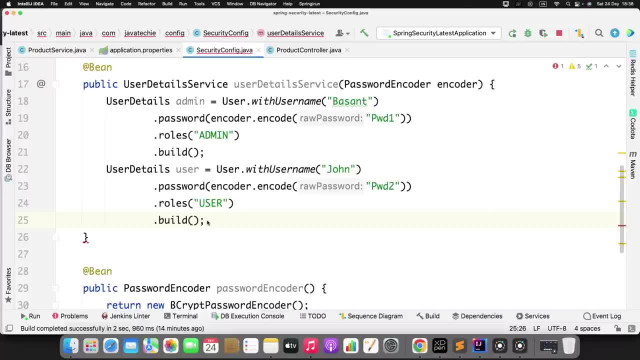 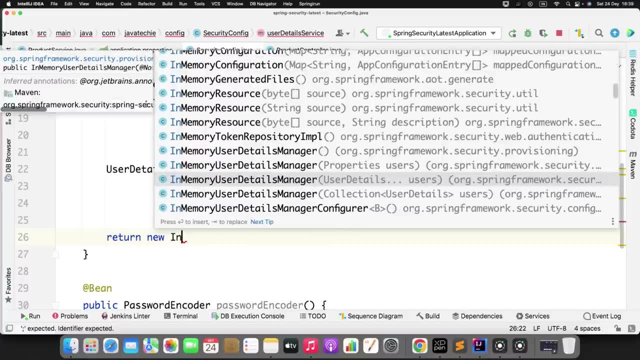 store these two user with in memory. okay, so what i can do i will just use return new in memory user details or something like that, in memory user details manager. okay, so what i can do, i will just use return new in memory user details or something like that. 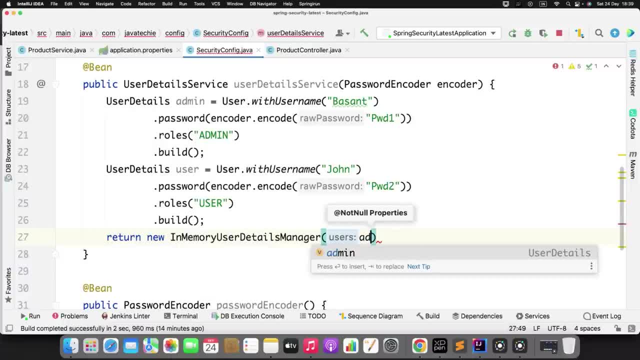 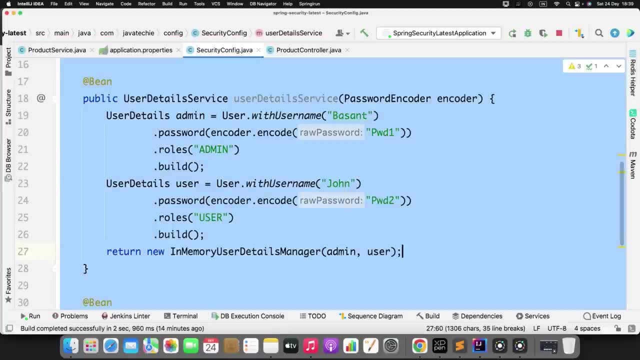 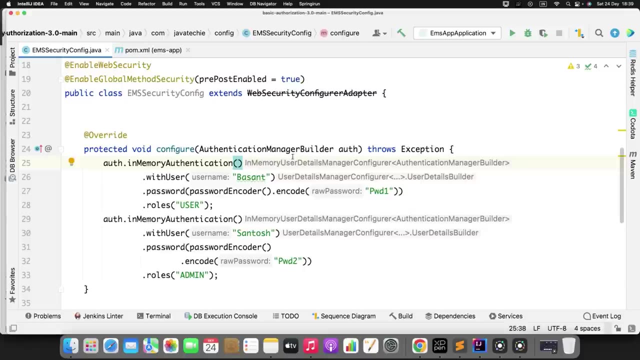 and give all the user details you have. i have admin and i have user. these are the two user i have. fine, now see if you will compare here earlier we have the overloaded configure method right, and inside that configure overloaded method- i mean this particular method- we have something called. 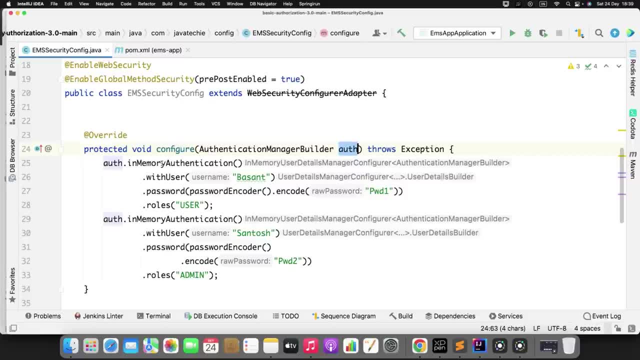 authentication manager builder. to this authentication manager builder, we are just building the user details and we are storing it now, since this configure method is not working. we are just building the user details and we are storing it now. method is not with us with the springboard 3.0 version. we are just creating the user detail. 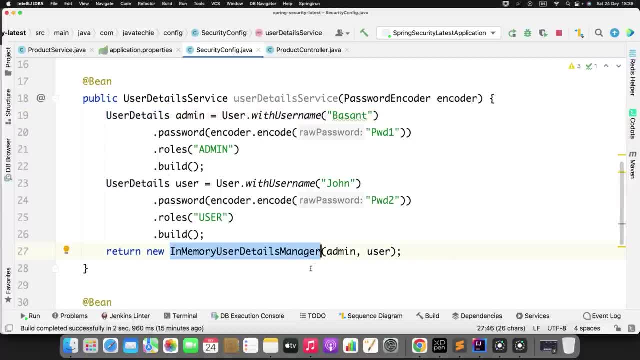 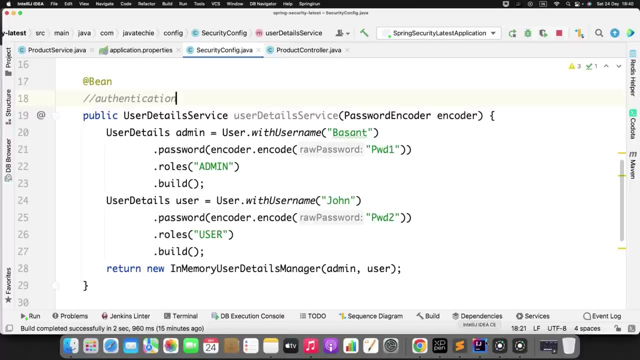 object manually and at the end we are giving it to the user details manager to tell that these are the two user details i have. okay, and we have exposed it as a bin. this is what we have done about our authentication. but if you compare the old approach, we have configured the. 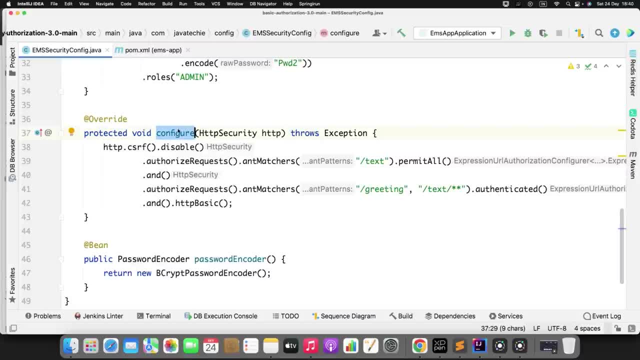 authorization related. stop in the second configure method. who takes the argument as http security? right, but again, we don't have this configure method with us. how we can do that? so that is the reason: springboard 3.0, given a new class called spring security filter chain. so we 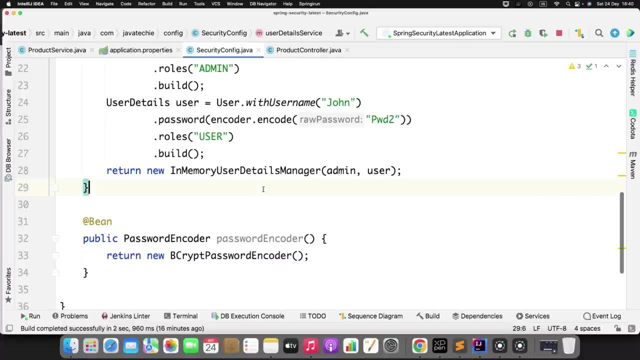 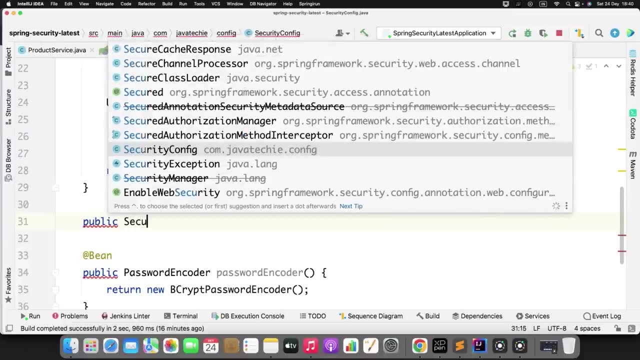 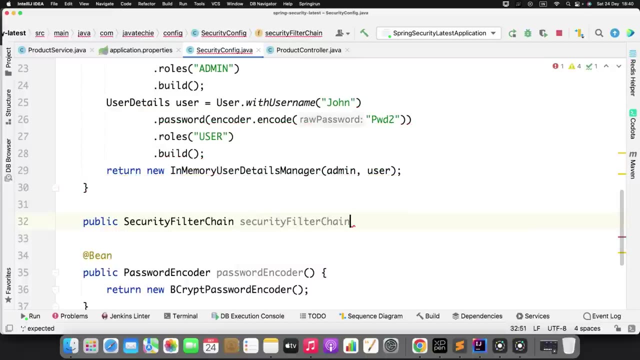 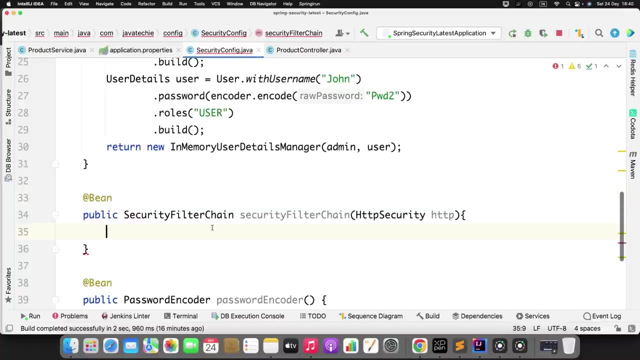 can use that class, we can expose it as a bin and we can configure our authorization related. stop how we can do that. so just do public security filter chain. yeah, security filter chain, security filter chain. then i need to pass here http, security http. i need to expose this as a bin. fine, now, here you have http with you now, the way we have. 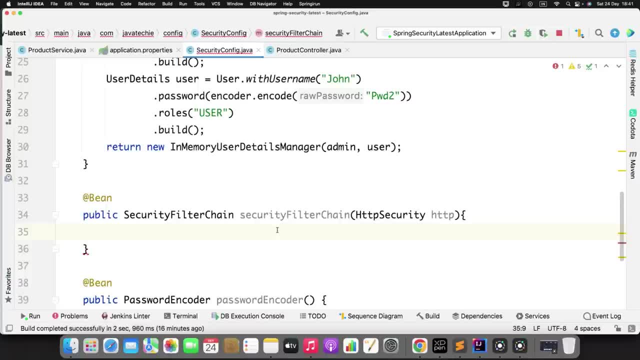 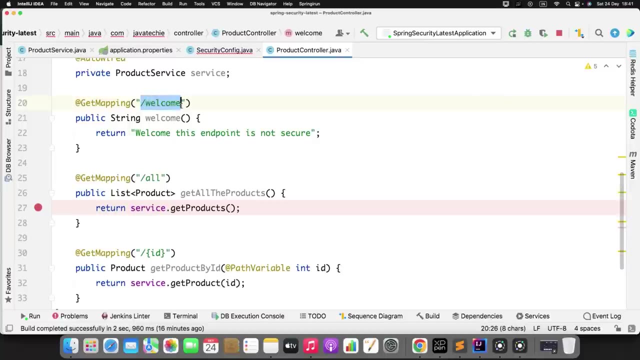 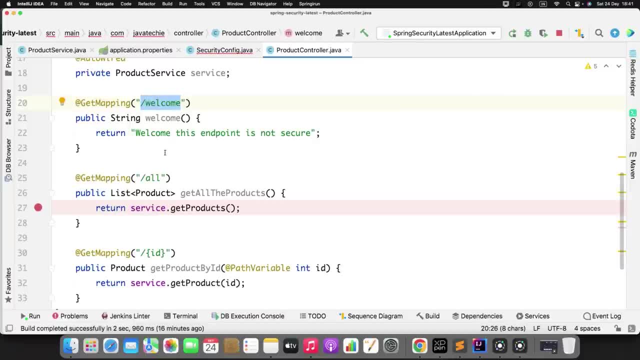 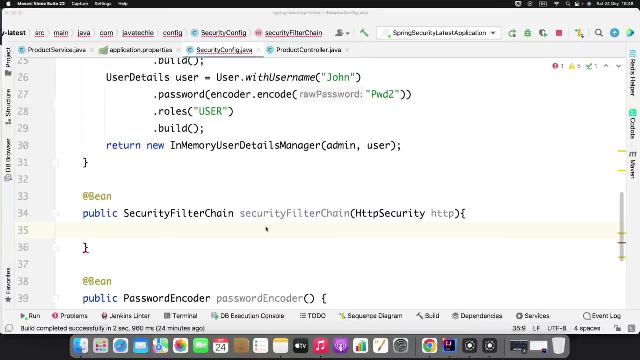 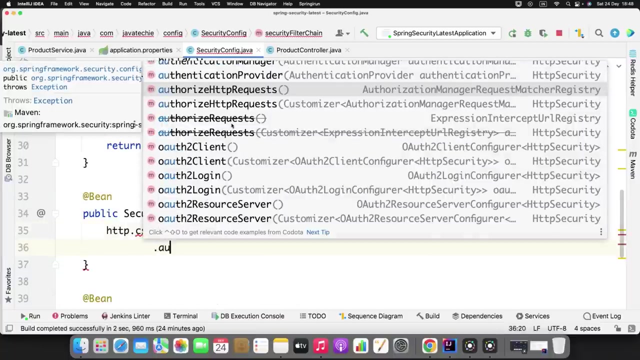 welcome, without any authentication. okay. and i want other two endpoints: slash all and get the product by id. these two endpoint i want to authenticate how i can do that. simply, you can go to the config and you can define something like this http, so you can type here: dot, csrf, dot, disable it. fine, then authorize all the request, okay, so you. 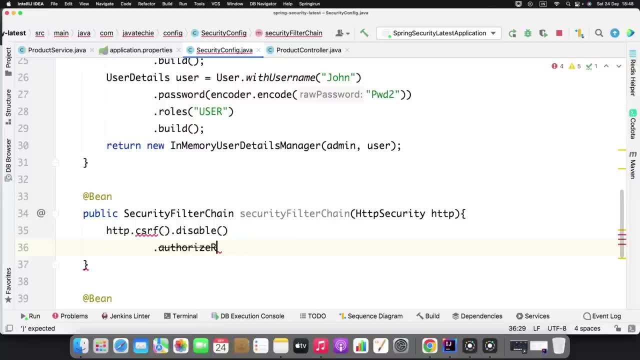 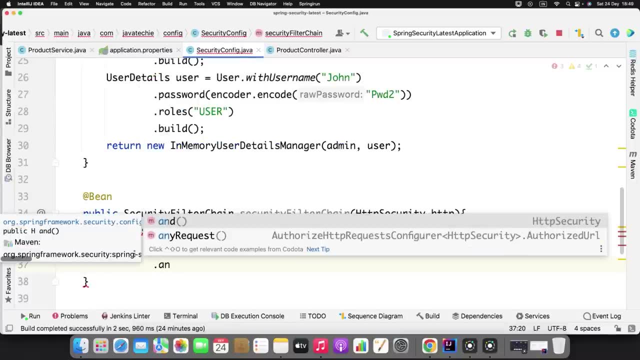 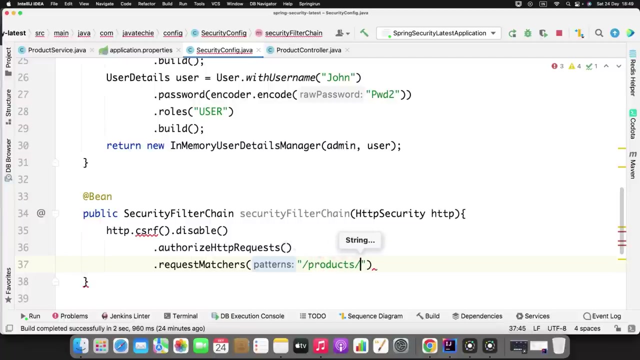 can see here, authorized request is deprecated, so you can use authorized http request. okay, and then dot aren't matchers. so that is also not available. now the aren't matchers method is changed to request matchers. okay, here you can define if the url is coming with slash products, slash- welcome. 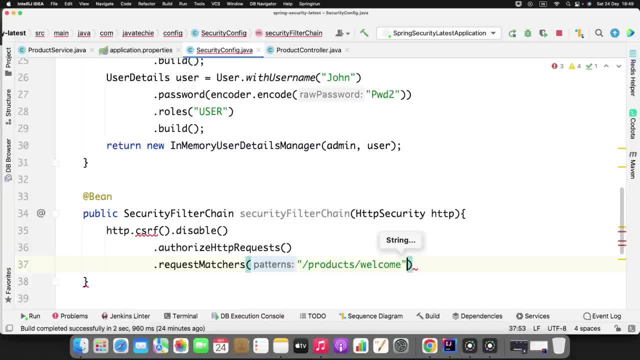 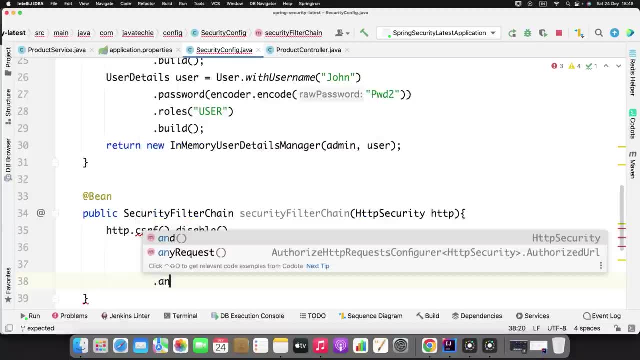 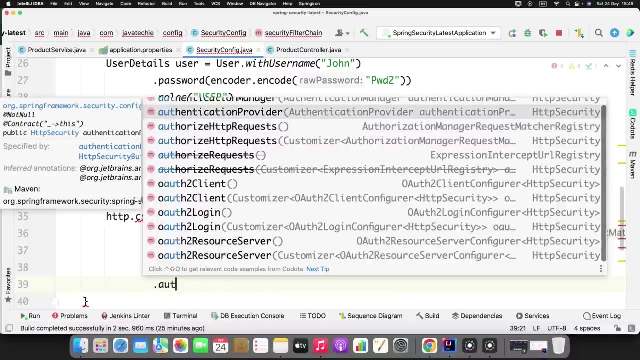 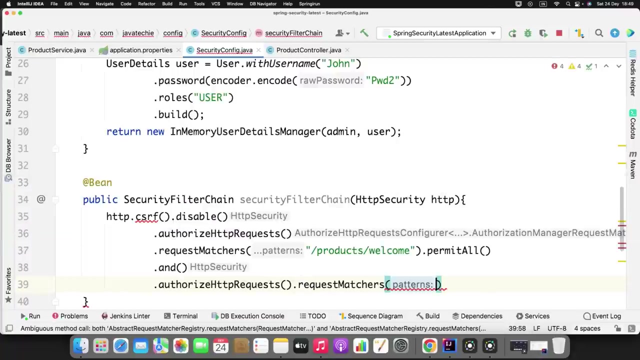 then bypass it. i mean don't authenticate it, just simply permit all the request, fine. and if request is coming with, i mean you can also authenticate using authorized http request. if it is coming with the url slash products, slash, all okay. or you can simply define: slash products, slash, star star. apart from slash products, slash, welcome. if any url is coming. 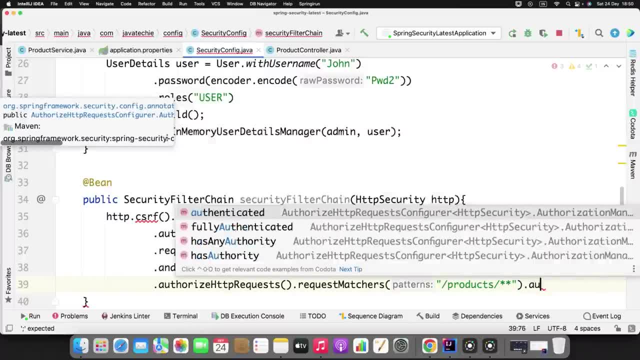 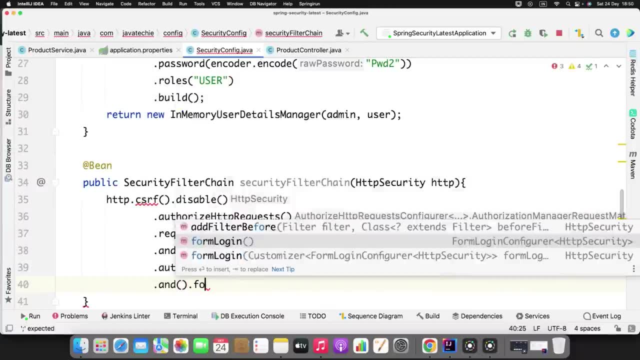 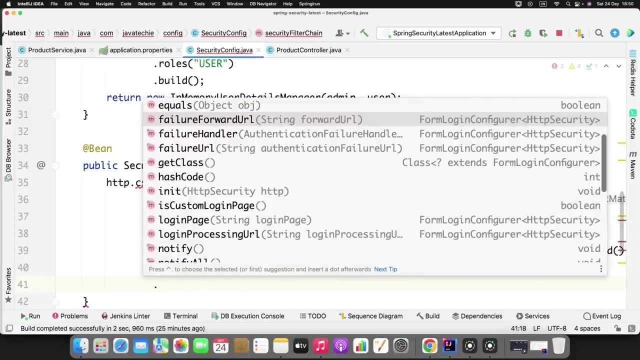 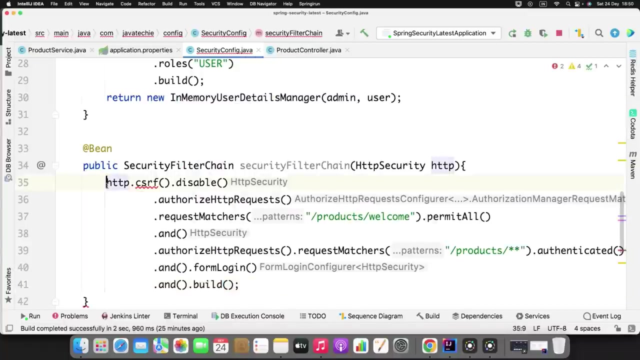 with slash products, then authenticate them. okay, and how you want to authenticate. let's say you want to authenticate based on the form login or http basic, it is up to you. so let me use form login, okay, and then simply build it. now i can return it, fine, so just handle the exception. 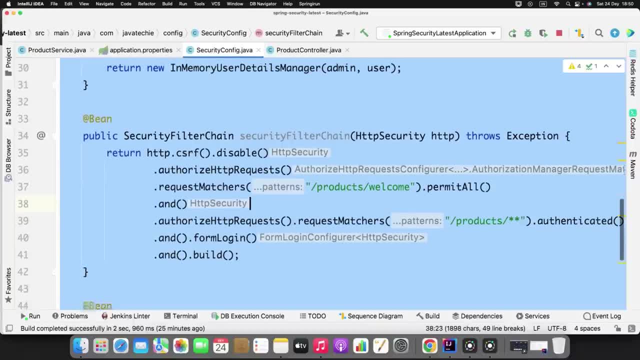 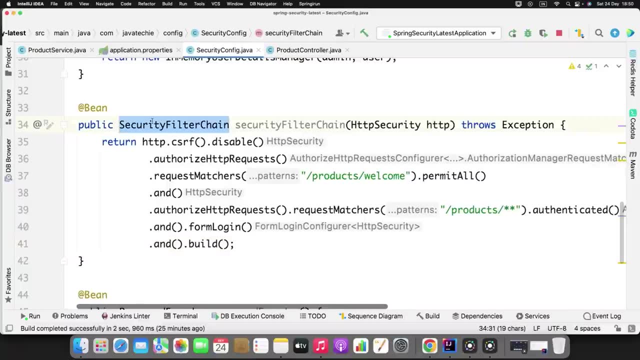 this is how you can define the authorization in lattice springboard version. you need to create a security filter chain and you need to tell what all url you want to permit all and at what url you want to authenticate them. so i can break down here. okay, so you can do like this. this makes sense. 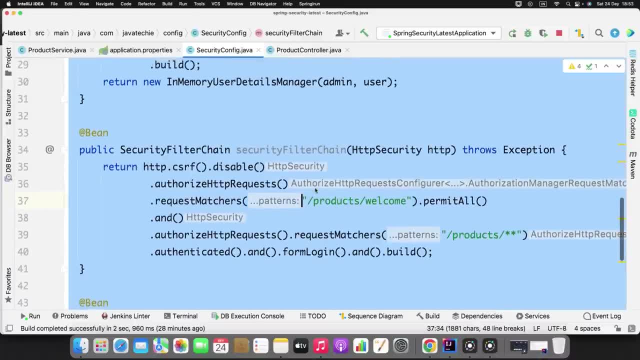 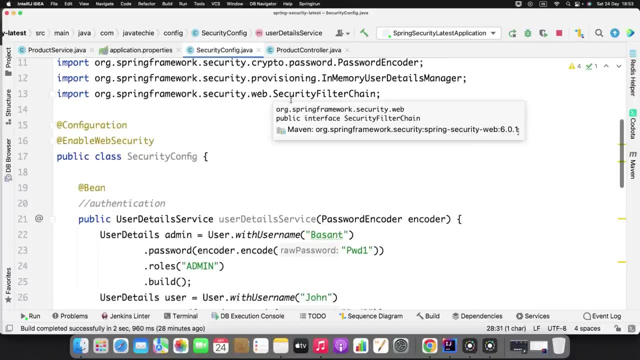 right. so this is how you can define the authorization and you can define the authentication here, okay. so now let's quickly test this endpoint. i mean, you can define the authentication here, okay, it's task. please mein with this credential whether you are able to access or not. before that, let me 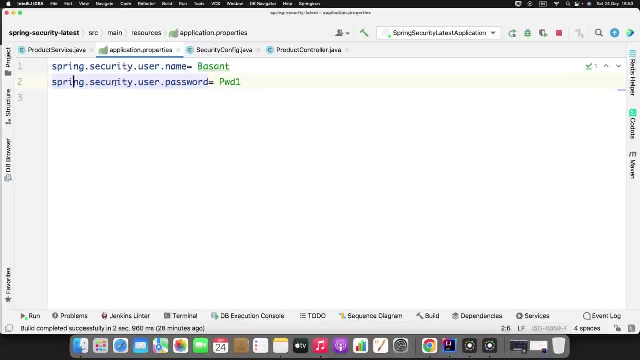 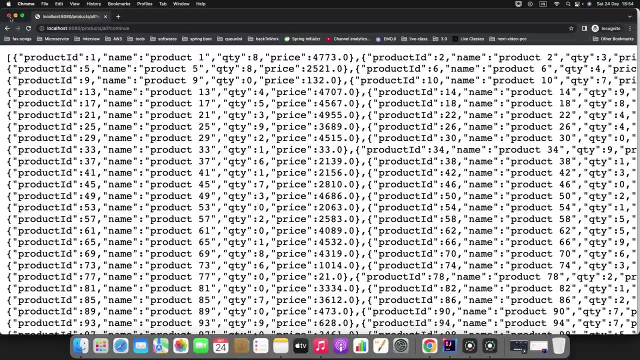 comment these two in my properties file. okay, so i can comment this. let's run it now. so it started on. put 8080. now let me go to the browser. okay, so, since you know we bypassed the url slash, welcome. okay. so if you go to the controller, i can specifically this method: red continuously. okay, and when we retail it does it will access the site as well on this network. so i'll add this. but when you do, then let's see if you'll see the earth will access the benchmark. it always has a special feature next to it to add each of the container. okay, i'll add each. 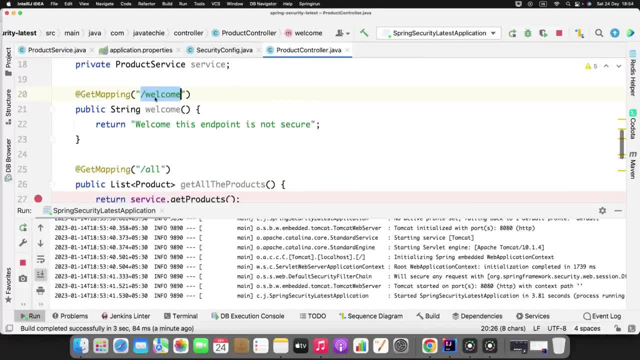 check out also with a save and console. i'll add: i just entered jeszcze that WITH. we only follow the wealth. after this error we'll wait for the solution. it'll bringing my update of the principalmente if i'll hit the slash. welcome. it should not force me to authenticate because we have just configured. 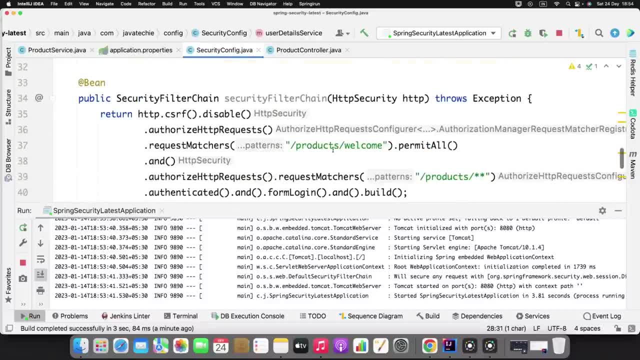 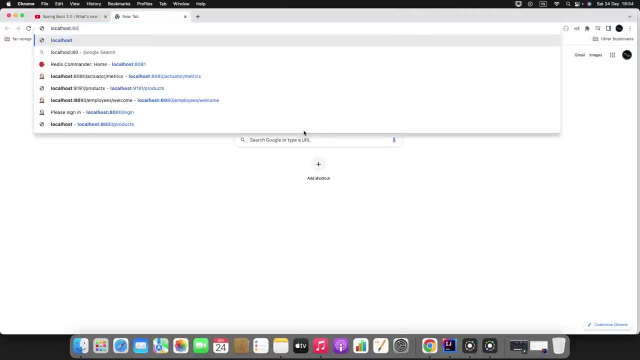 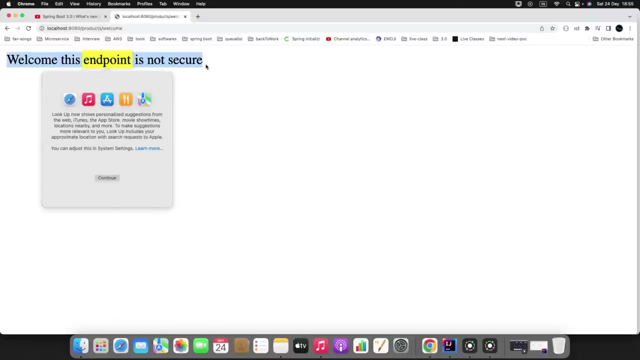 here, right? if url is coming with slash product- slash- welcome. then permit all the request. just go to the browser. i'll type localhost 8080, slash products, slash- welcome. i'm getting the response here. can you see here: welcome. this endpoint is not secure. this is what i'm bypassing: this particular url. if url is coming with. 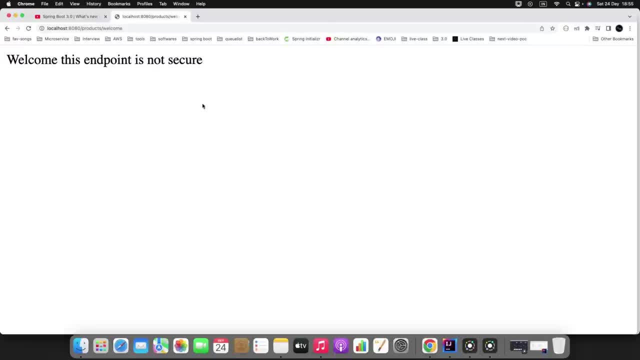 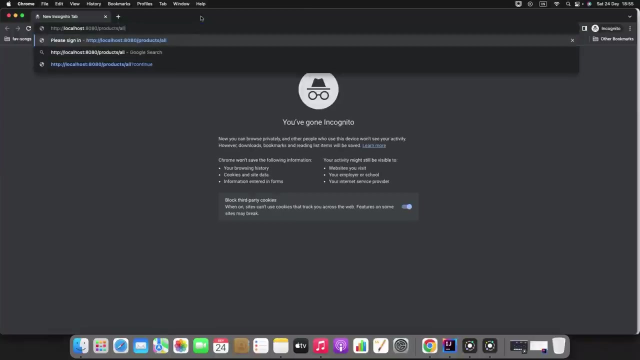 slash product slash. welcome, please don't authenticate it. okay, now let's verify the other url. so let me copy this and then i'll open a new mode, incognito mode. okay, i want to fetch all the products. can you see here when i try that particular endpoint? 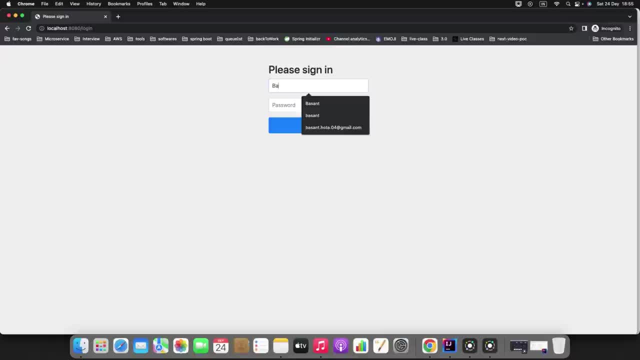 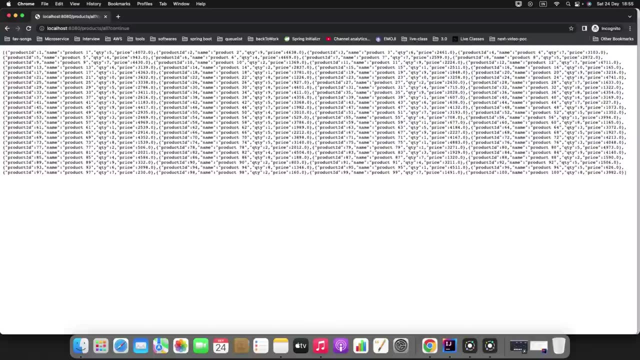 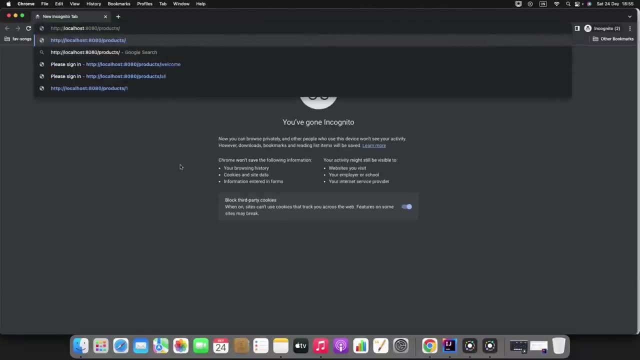 it is asking me to give the credential, so i will give basant pwd1. i will sign in. i can able to see the response, so i'll open a new tab. i will hit the same endpoint: get all the products. okay, i need to close it, then i need to. 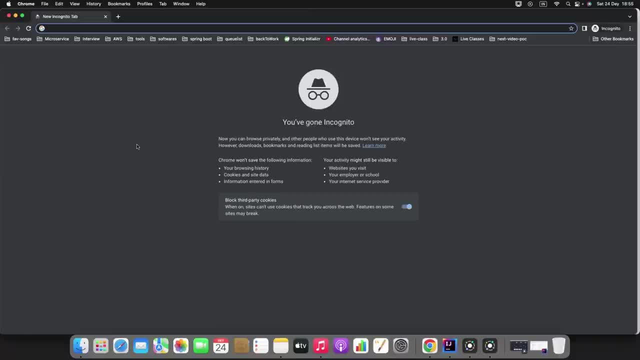 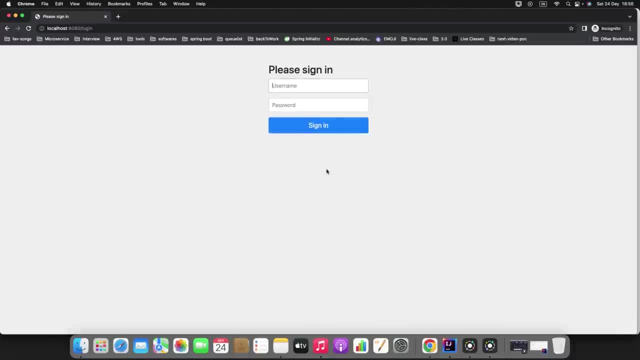 retract it, and then i need to close it, and then i need to retract it and then i need to write with the different user command, shift n, localhost. i mean i have the url copy, just change it to the all. it's asking again username and password. second user is john right john and pwd2. 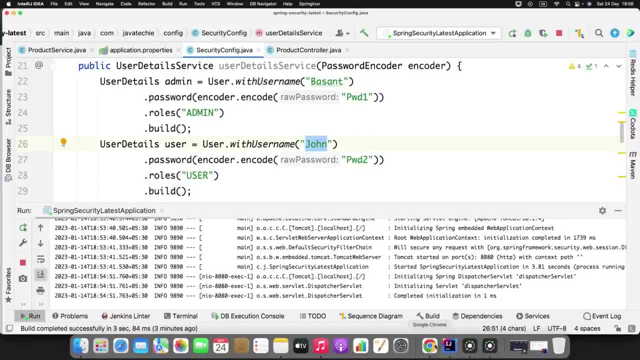 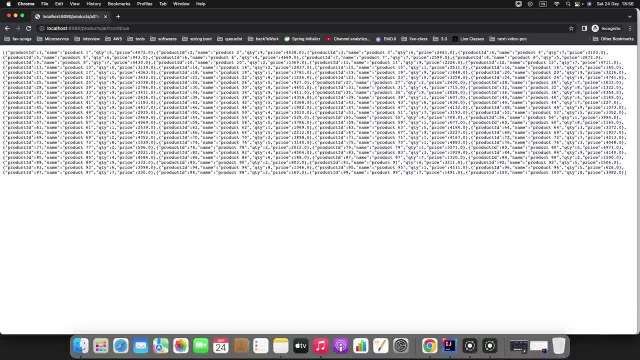 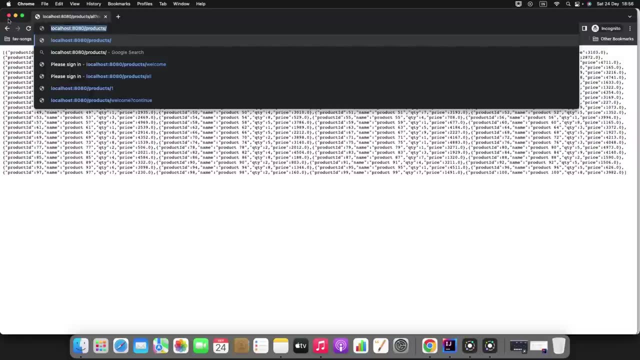 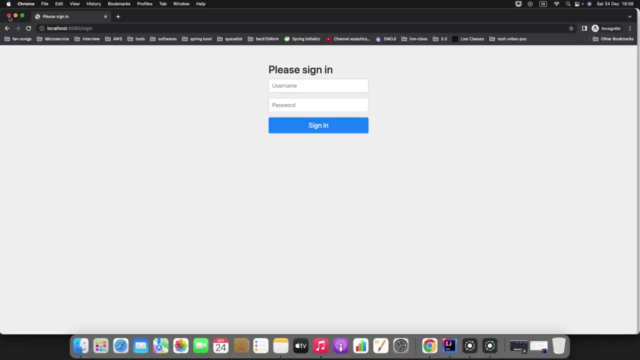 so i'll just copy his name. i'll go to the browser. username is john, password is pwd2, so he's able to access. similarly, we can try for the endpoint products by id. right, so let me copy this. i will open a new incognito mode. id is one. it's asking username now: basant and john. both can access. okay, because even though we have 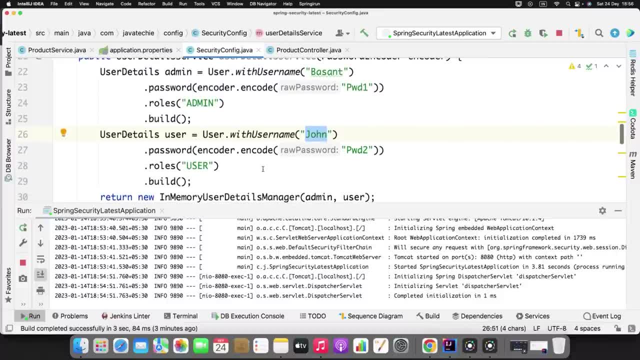 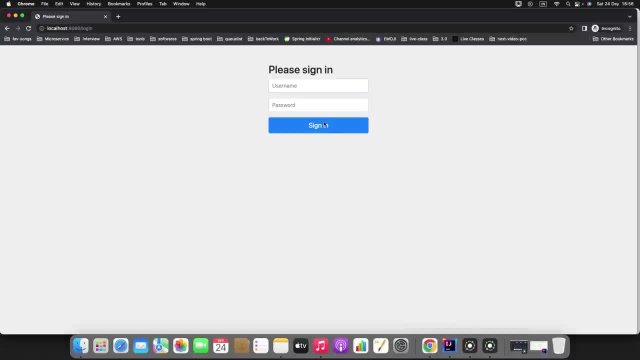 defined the role here. we didn't specify to the method which method can be accessed by which user. that we have not configured yet right. so if i'll try here with john and pwd2, he's able to access. we got the json response right, so this is what we understand about. 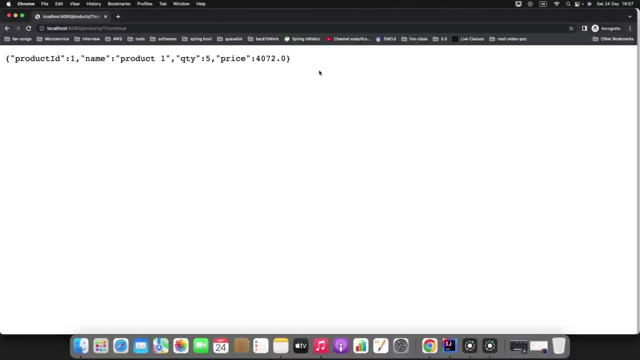 the authentication we give the username and password. it validate whether the given input or username and password is correct or not. this is what authentication. now we need to understand authorization, how we can perform authorization in this spring security 3.0. so when i say authorization now, let's say: 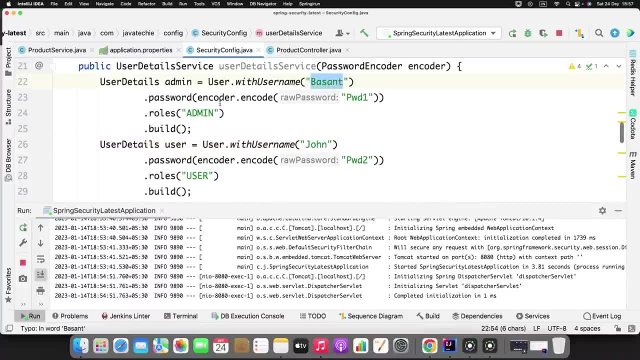 this guy, basant, is the admin right now. as a admin, what all feature basant can access as a user, what all feature john can access, that is what i am authorizing him to access. these are the endpoint. i am authorizing, authorizing him to access. these are the features. so this is how we 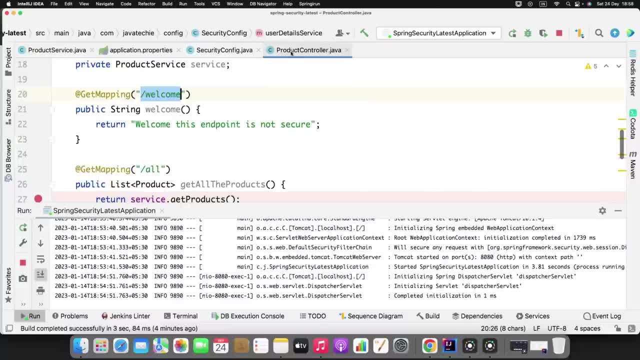 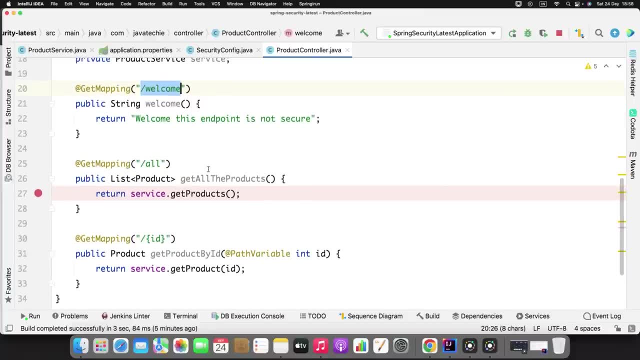 can authorize them. now, for example, let's say in our product controller we have three endpoint. right, we bypass it, but i want only who is the admin. he can view all the products present in my warehouse, okay, but only the user can view a product by id. i mean, i just want to specify this particular endpoint. 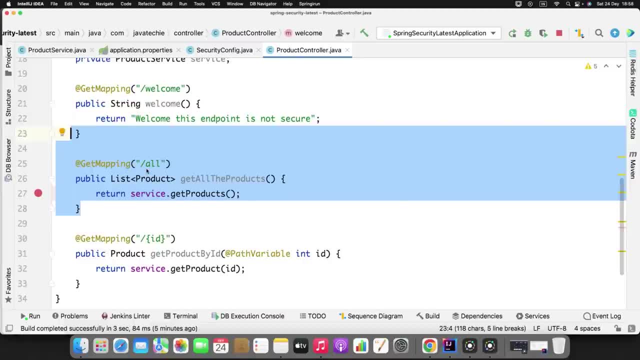 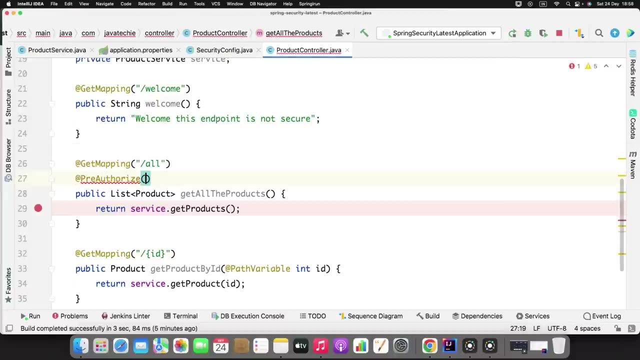 can be accessed by the admin, not by any user, but this particular endpoint can be accessed by only user, not by admin. okay, so how i can do that? simply, you can have a annotation here pre-authorized, okay, and you can define here. you can define here: has authority, okay, what is the authority? 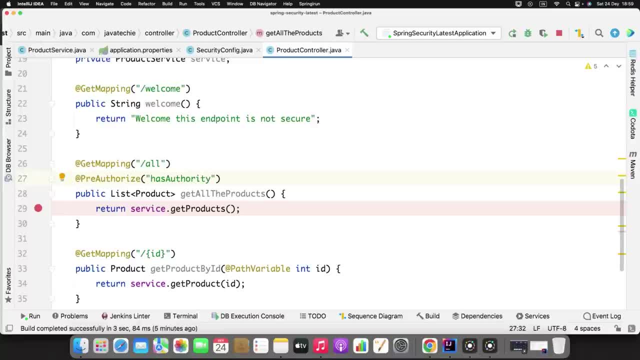 who can access it? admin right. if that user is having the admin access, he can access it. even like if you have some different KP farm or you have some different verification system had to do separate authentication. we go to get share inside viruses server. you can see within the directory. okay, you should. want to check between little master or in some language, if you are creating. your app is working. v้et also asked you to tell him a little secret. Cam крюк, it only fingers crossed. those are here. dvrW-R. sincerity word. sorry if you are using an advisory. 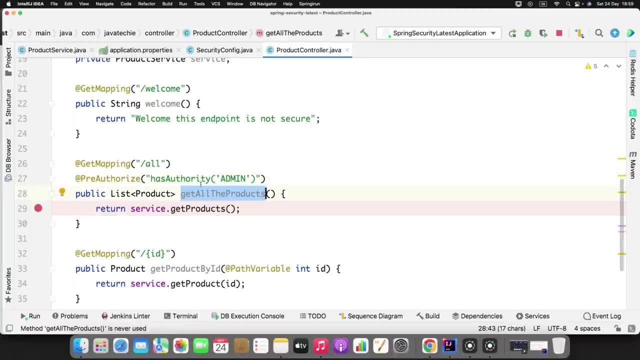 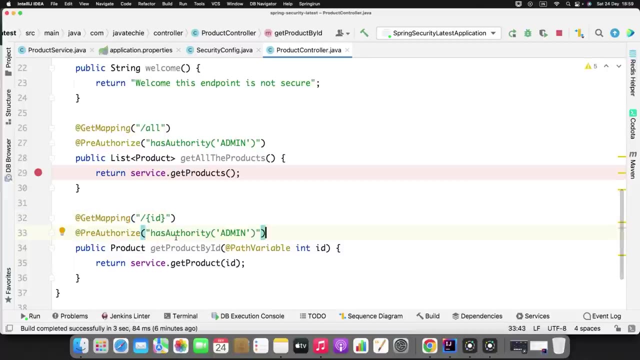 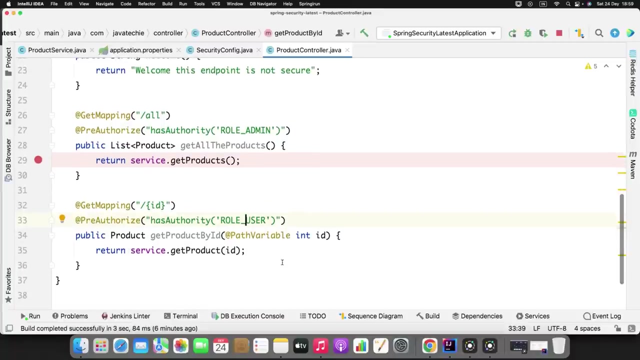 able to access this particular endpoint has authority admin. okay, similarly, i can define for second endpoint. let me copy this properly. i can define here: if the user has authority user, he can able to access it. so i believe we need to add the role underscore admin and role underscore user: okay. but by defining this annotation we cannot achieve the authorization. 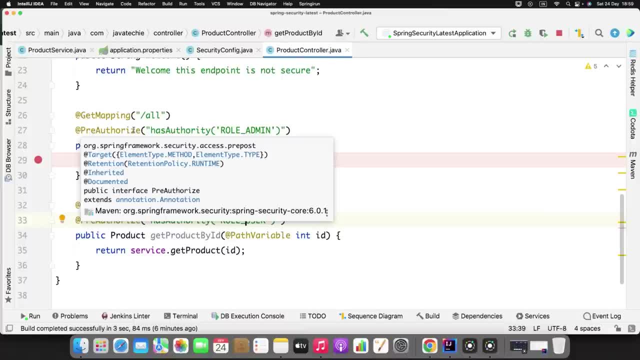 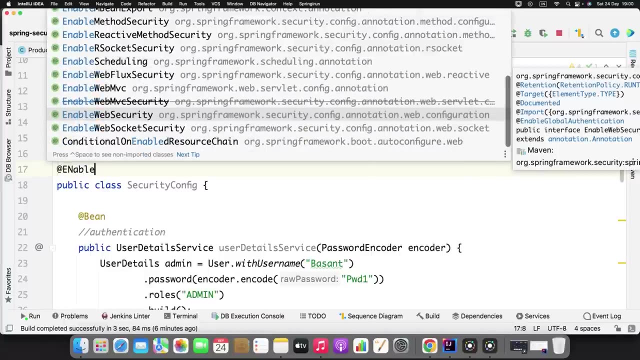 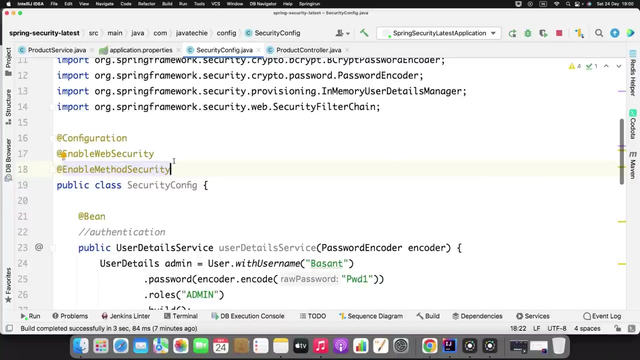 so we need to tell to the spring security: hey, i have implemented method label authorization. okay, how we can do that? just go to the config and you need to play with another annotation called enable. uh, what is that? let me type enable method, method, method security. okay, but not that. before that we are using someone, some, some different annotation. 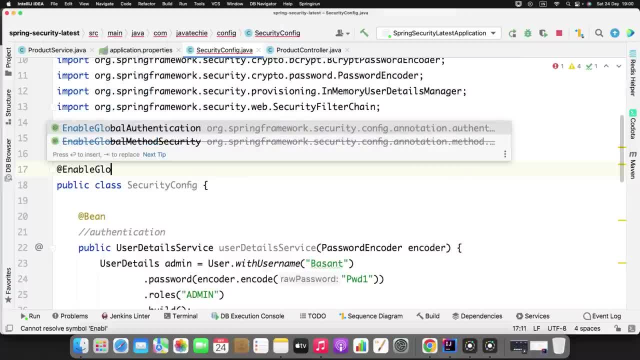 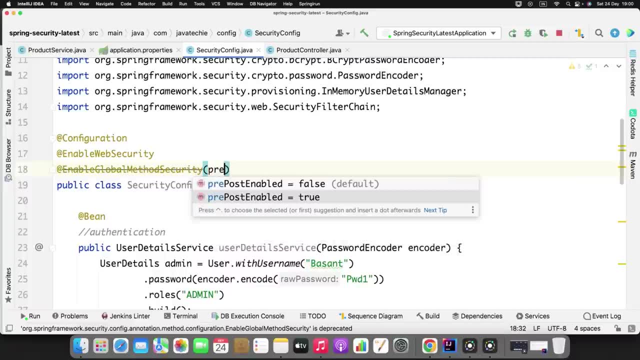 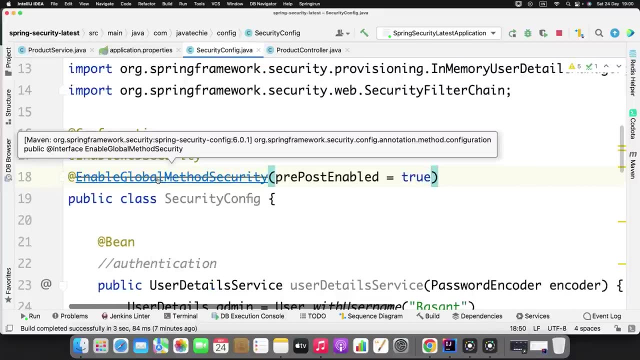 something. if you type enable- yeah, can you see here: enable global method security, and we are just specifying here: pre post enabled. true, right, but if you observe, this particular annotation is also deprecated now. if you open the source code of it, it will suggest you what annotation you need. 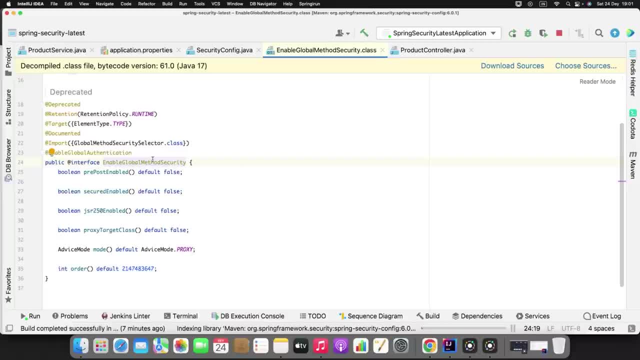 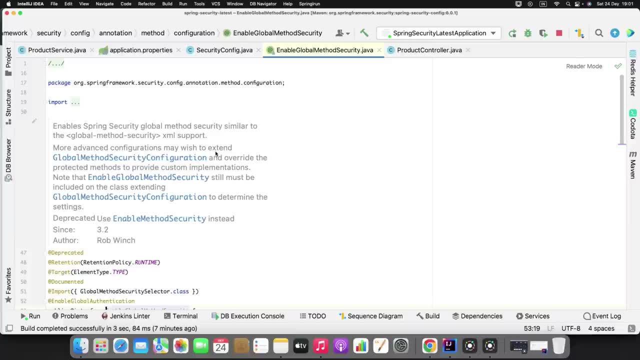 to use rather than this deprecated annotation. okay, so it is downloading the source code. if you will scroll up more advanced configuration, may wish to extend global method security configuration. note that enable global method security still must be include on the class extending this configuration. deprecated use: enable method security. now the annotation is this: okay, you can. 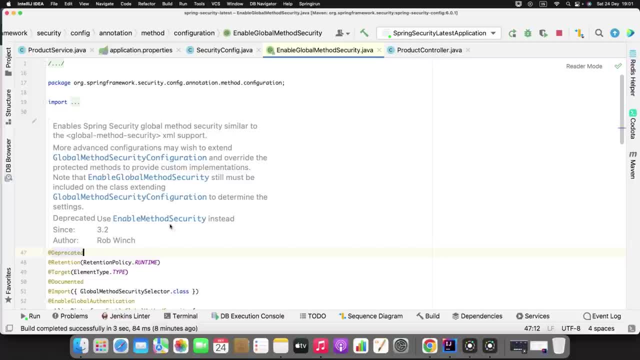 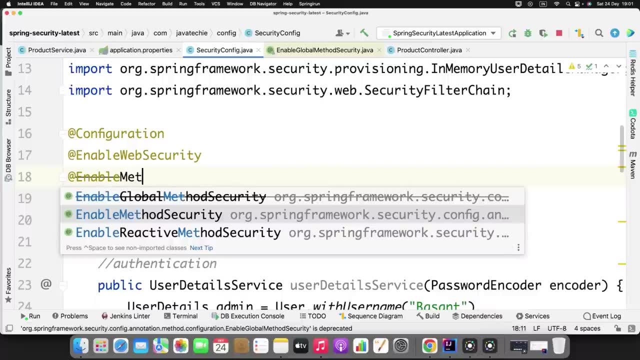 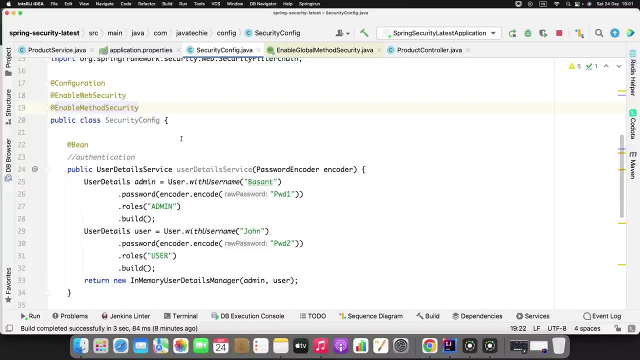 use this annotation. what is that annotation? in my end point, controller class basant can only view all the products because he is the admin access and john can only view the product and i have breaking access all over again so i can start adding or Questo this location things. now, this is all i did not know and i 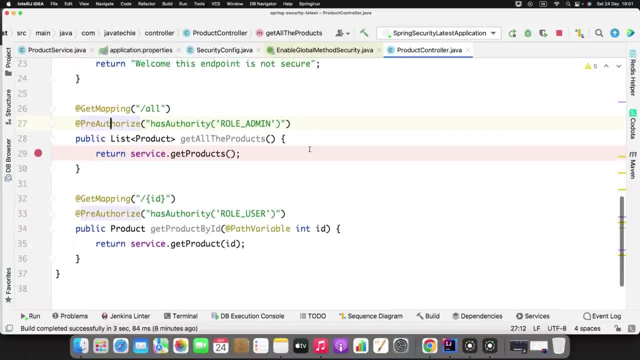 will need to navigate the menu ver for now. okay, now you can see that snel event contents you just need through the fringe of이야, victory and better, which serves as an option. so by default I wanted to save for something else- other functions- because it will work on the channel. 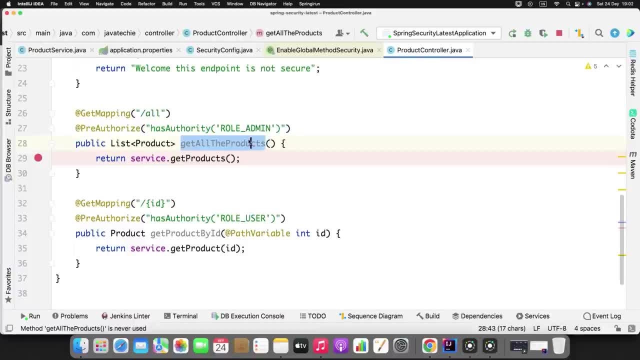 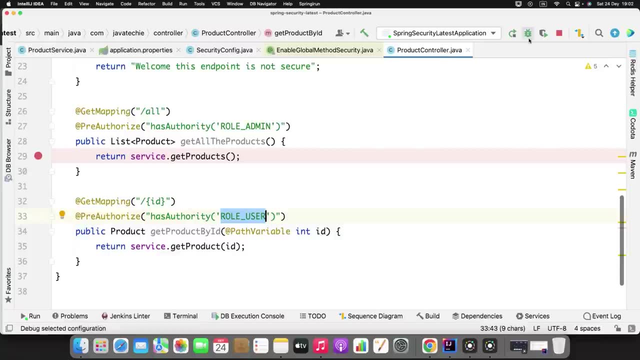 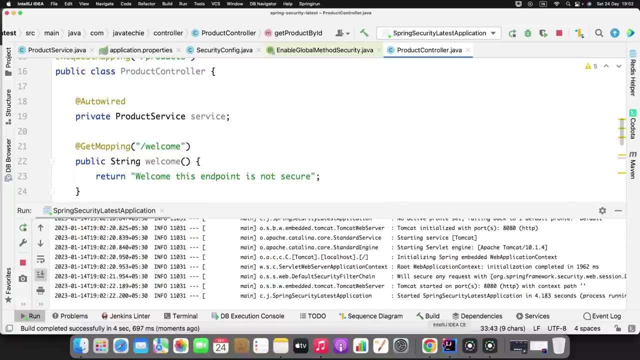 the specific product by id. okay, this particular method can't be accessed by the user and this particular method can't be accessed by the admin. fine, let me restart the code and we'll verify now. so application started. you can go to the browser. let me close this. let me open a new browser. 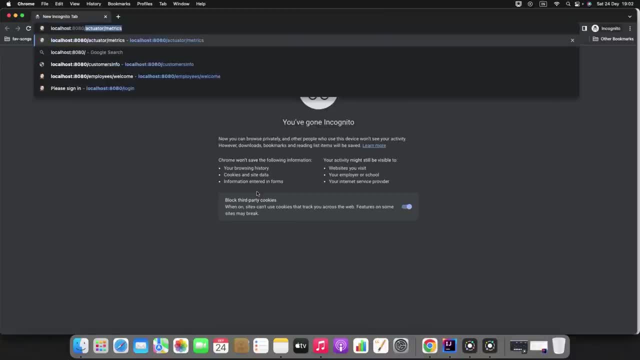 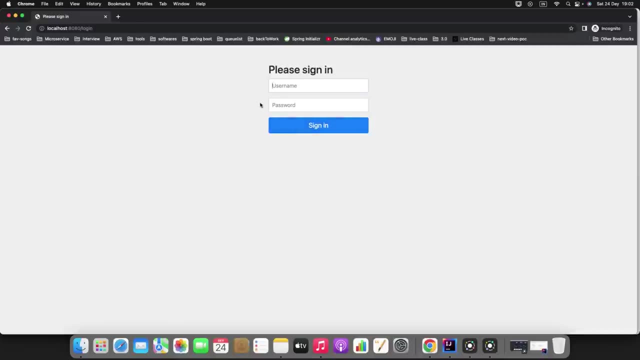 localhost 8080, slash products, slash, all. now this all endpoint can be accessed by only admin. basant is the admins, but let me try with the john. okay, john pwd2. it will give the error. access to localhost was denied. he is getting the 403. 403 means forbidden access. he don't have, he is the. 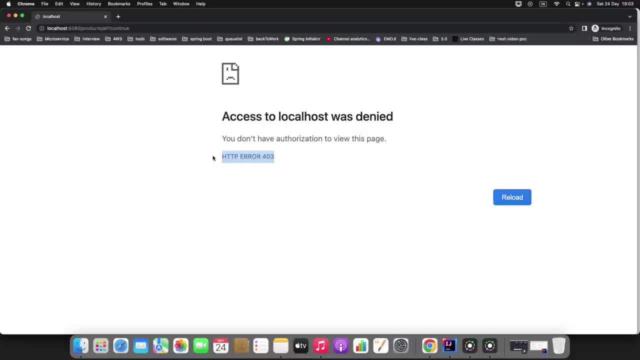 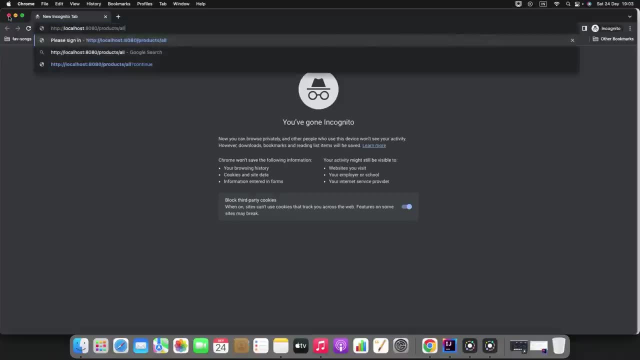 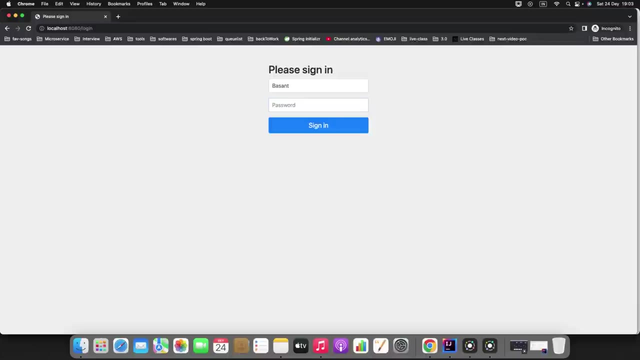 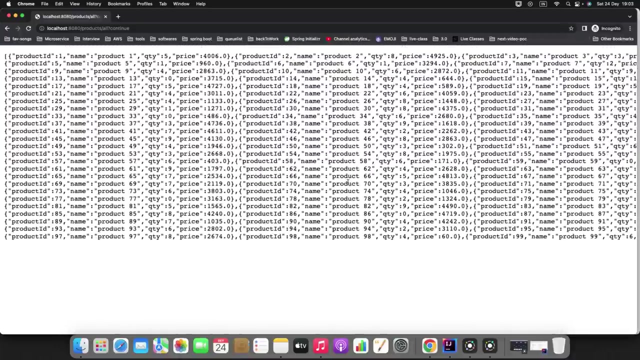 correct guy. he is able to authenticate, but he is not able to authorize to access that particular endpoint. okay, so what i will do? i will close this again, i will open and i will now give the basant, because he is the admin he can access. slash all endpoint. password is pwd1. can you see here the authorization is also working, only you. 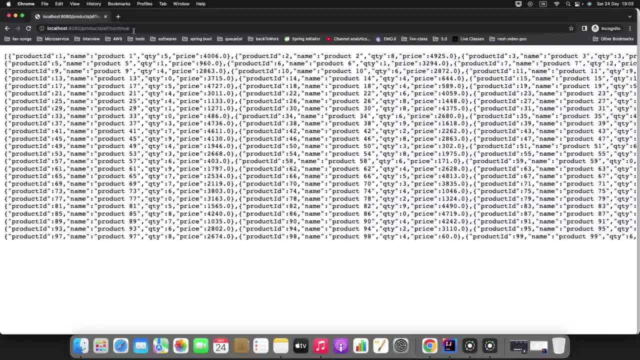 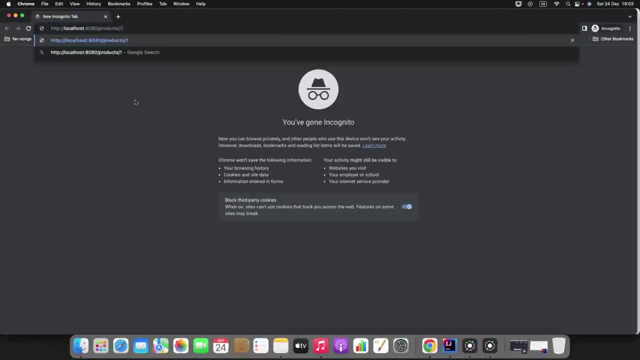 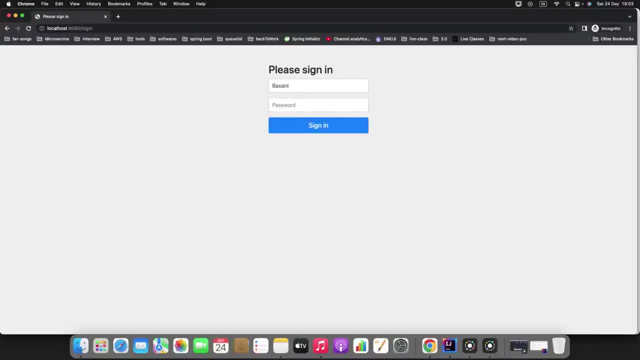 need to change the annotation introducing the springboard 3.0 now. similarly, if i will try with the get get, get a product by id id1 who can access this only user. okay, but let me try accessing by admin, because basant is admin, right? so, pwd1, if i will send the request it should fail. can you see, here we are. 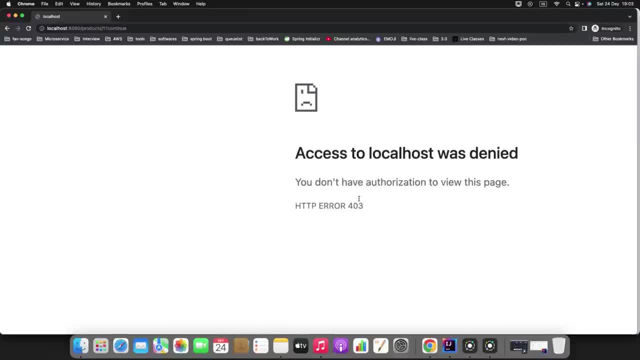 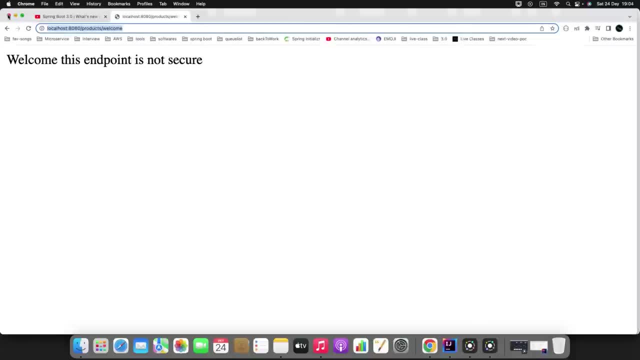 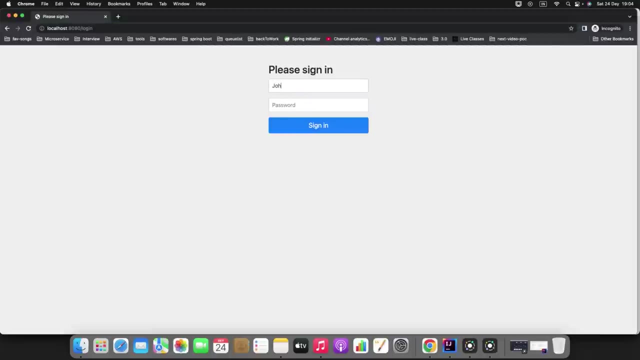 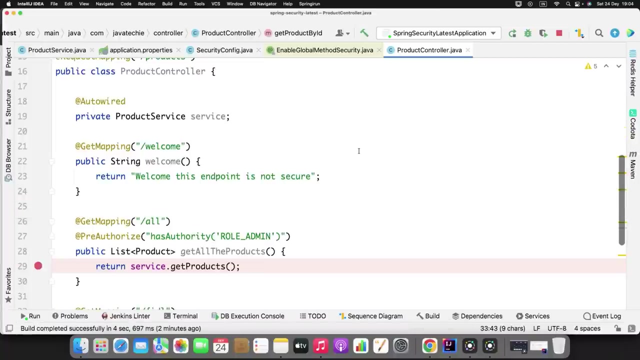 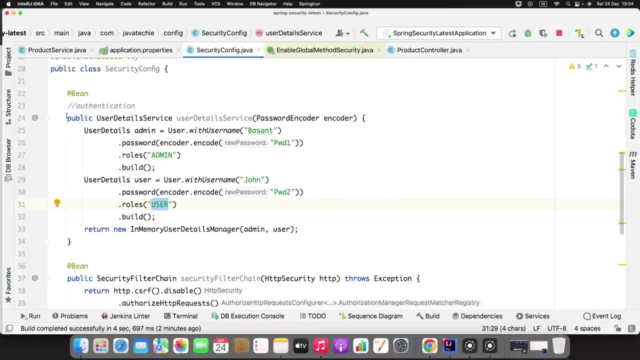 getting 403, which is nothing forbidden. okay, basant is not authorized to access this particular endpoint. again, close this. open a new- now, if i will try with john, and password is pwd2 he is able to access. okay, so the authentication and authorization- both are working in our case. but if you observe what we, what we have done here in this security config, we hard coded the username and password, but that is what, not something we have to do. we need to fetch it from our db. 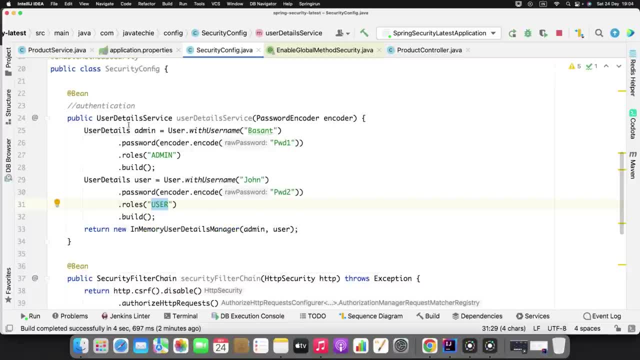 db, db. right, so how we can do that. since you said user details service you need to create as a bin, but i don't want to hard code this user details. i want to load it from the db. how can we do that simple step? okay, so what i can do. first i will 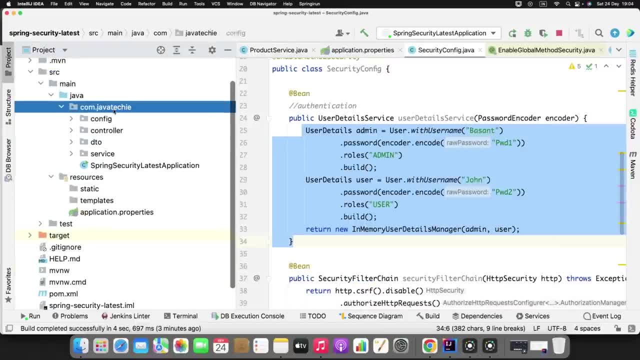 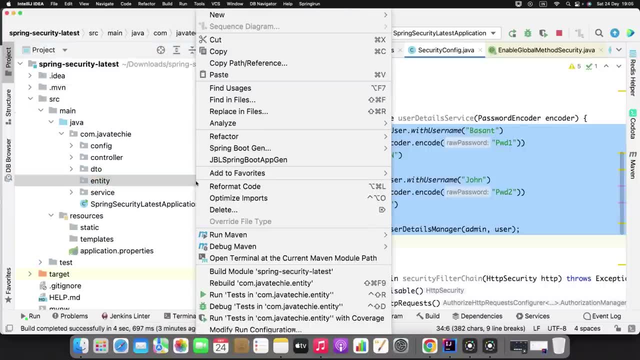 create an entity to store the username and password related stuff. i will quickly create a package, let's say entity. then i will just create a java class batch, let's say, every morning i will create a java class, let's say u2. so, because this is a brief, 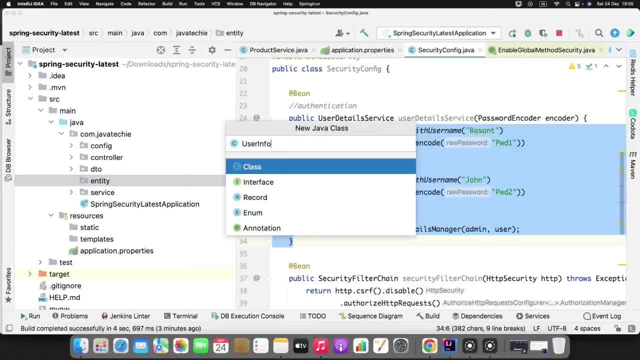 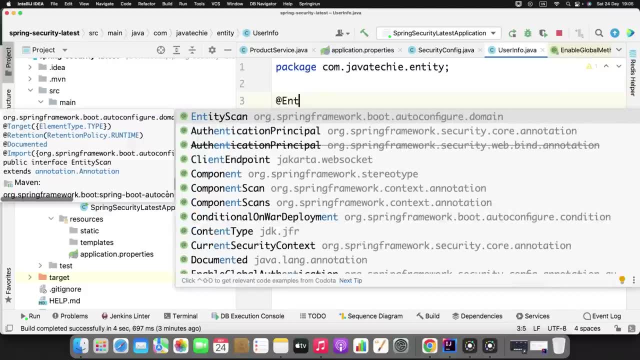 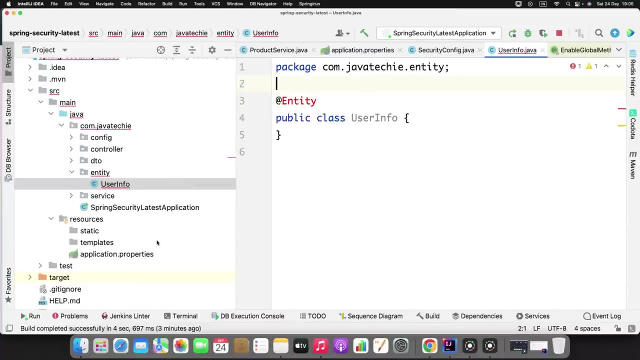 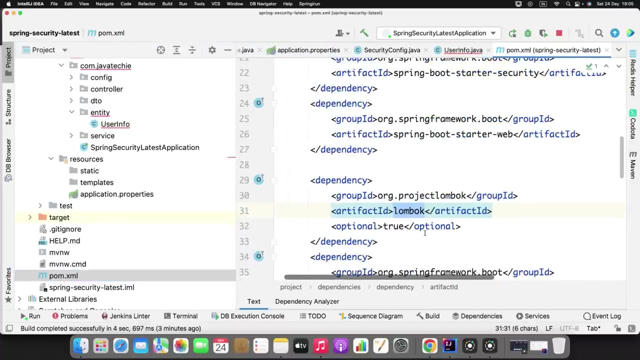 say user entity or user info, something like that i need to annotate here at the rate entity. i didn't add the jpa dependency. let me verify. okay, i didn't add the jpa dependency, so i need to add it, otherwise i cannot interact to my dv. 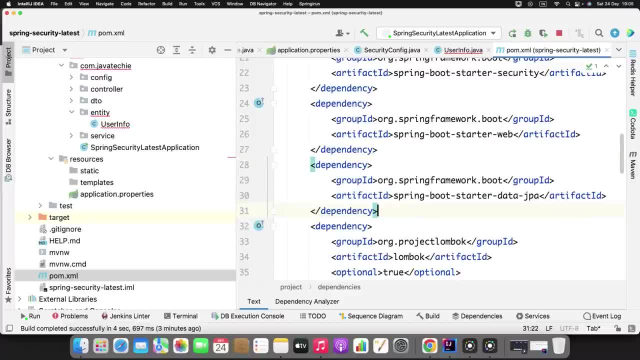 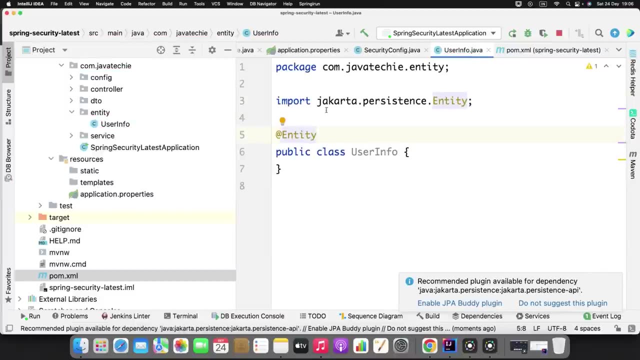 right, let me paste it down. just hit this maven update now i need to annotate this at the rate entity. fine, if you observe, the input statement is changed right: jakartapersistenceentity. this was recent change on spring boot 3.0. before that it was javaxpersistence. now this javax is changed to jakarta. 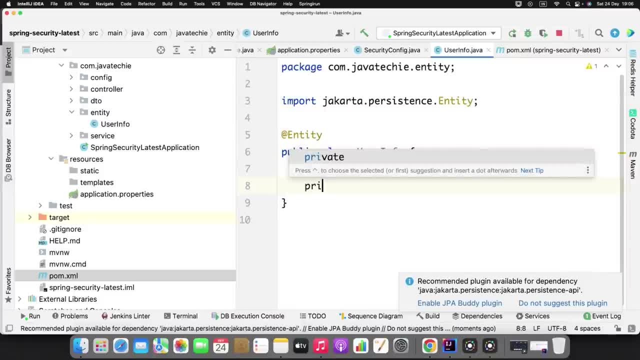 okay, and i need to define few field here. okay, let me quickly define private int id. private. what happened? i missed the semicolon. okay, private string name of the user. private, um, anything like id name is there. i'll just store the password. private string email: also. i'll keep okay, private string email, then private string. 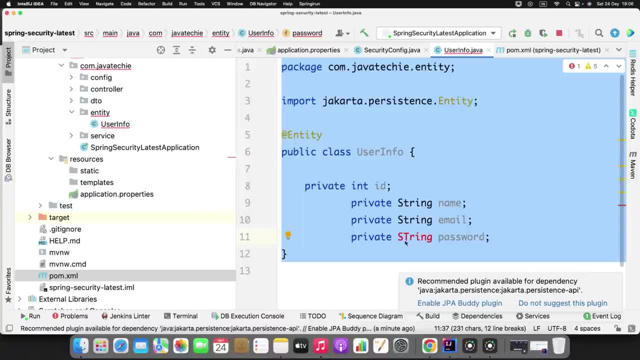 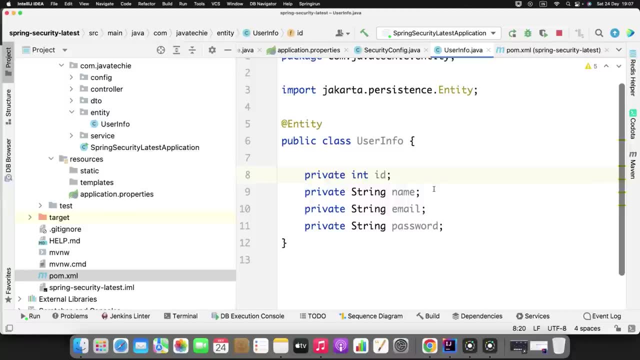 password. fine, i have defined four field: id name, email and password. and since i use the lombok, i can just use at the rate data at the rate, all argument constructor. at the rate, no argument constructor. and also i can define this as a primary key and i want it to be auto generated. generated value. 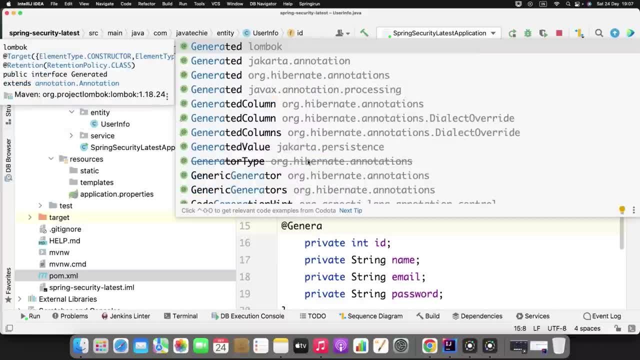 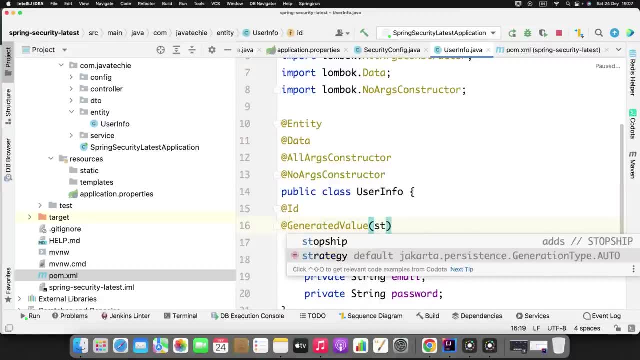 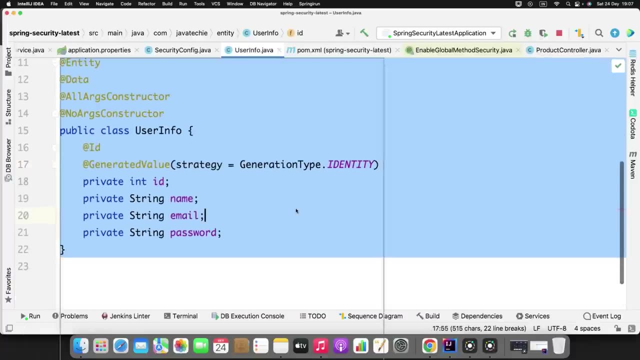 then what is that identity? i'll just use strategy find best started using an entity. fine, we have defined this entity, so i want to store the user information in there, dv, so that i want to load it from the dv for authentication and authorization. simple, just create the repository. i will just create a passesite, itlerpository, the enfim. known use thatHey guys help me enable strenuous mapping of files and it is șiśu's poison. allORD hari was 45 minutes, 2 Scholars City in hiv and he is fine after training- will get this c캰 ay the with entrepreneur to do it. I want to load this from the d movement Inversion from the form. I will just create this repository in the milyon marks membership folder. just create the repository in managing two rooms. we are going to call by ceremony. i'll just define this St am wanna to click on the dv. it is to form you the calm in the. 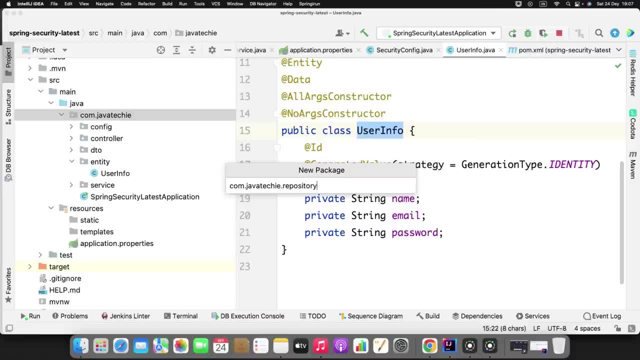 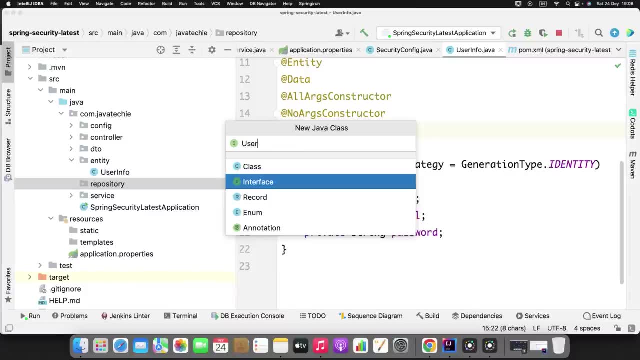 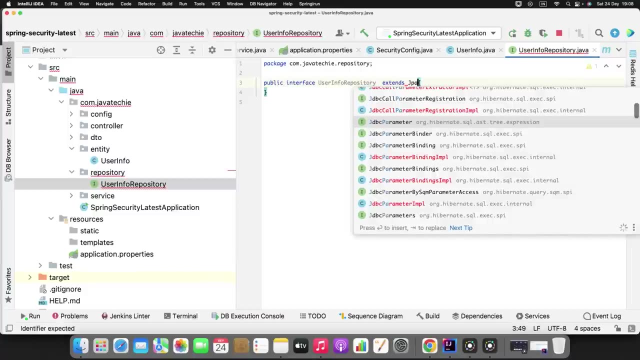 create a new package. i'll name it repository. i'll just create a interface java class. i'll change it to the interface. i'll just name it user info repository quickly extends it from jpa repo. first argument should be your model or entity, which is user info. 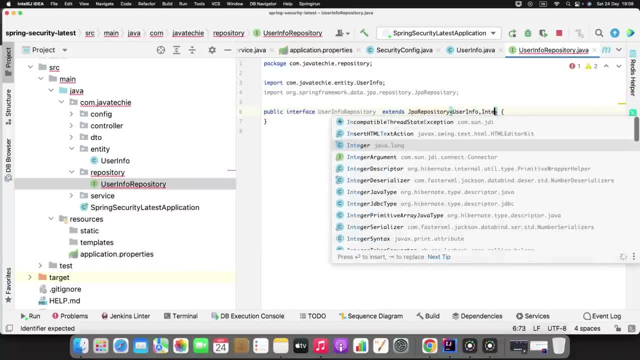 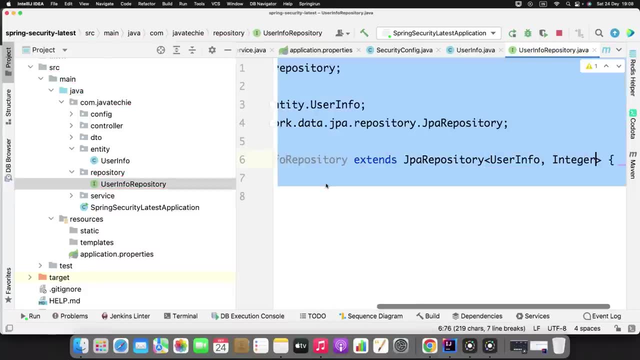 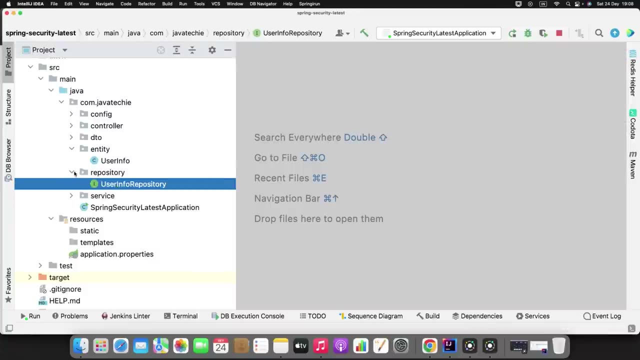 second is data type of your primary key integer. fine, user info repo, extend from jpa repo. that's it fine. i have created the entity and i have created the corresponding repository. that's fine, right next, we need to perform the authentication by fetching from the dv and, if you remember, we have configured the authentication related staff. 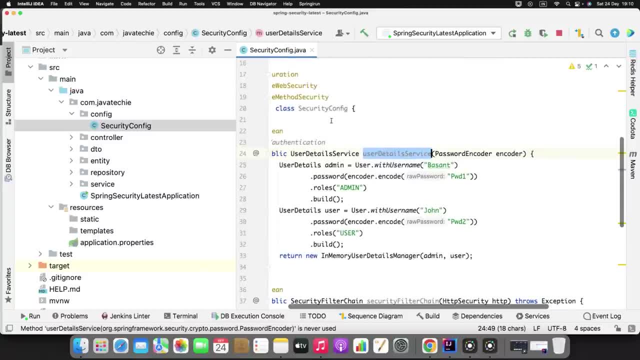 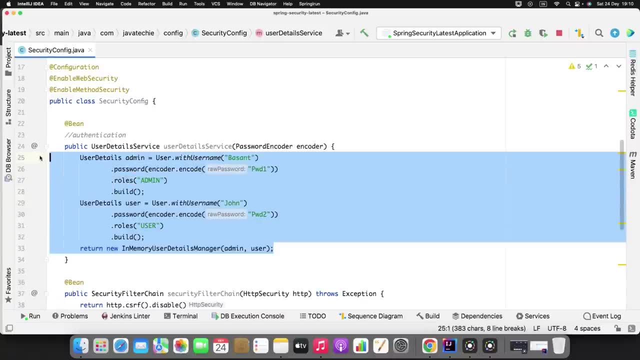 in the first bin, user detail service. right here we have hard coded the details, but that we don't want to do so for now. i'll just comment it. okay, and i want to create my own user detail service. who will talk to the db and will face the user details? okay, 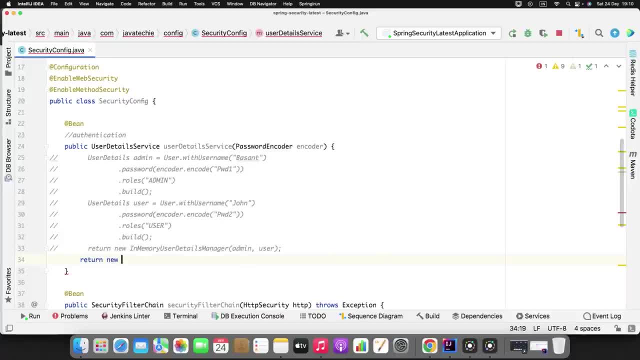 so for that, what i'll do, i'll just use return new user info user details service. okay, this is what the user info user detail service i want to create. okay, so i'll just create this class, create a class of this. i mean i'll create in the same package. it's fine, but better to move. 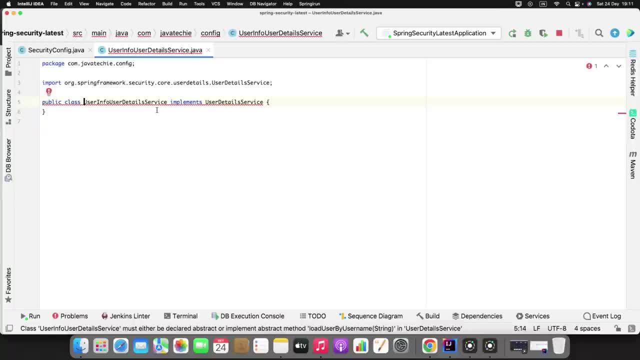 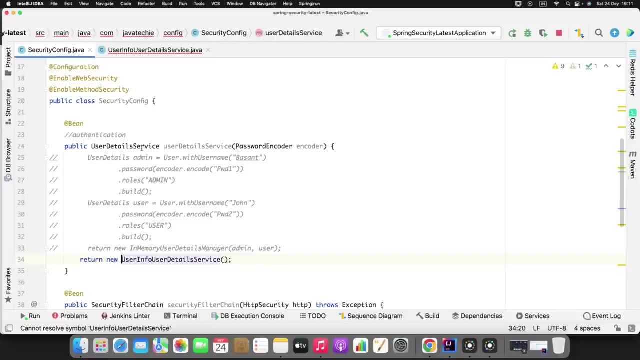 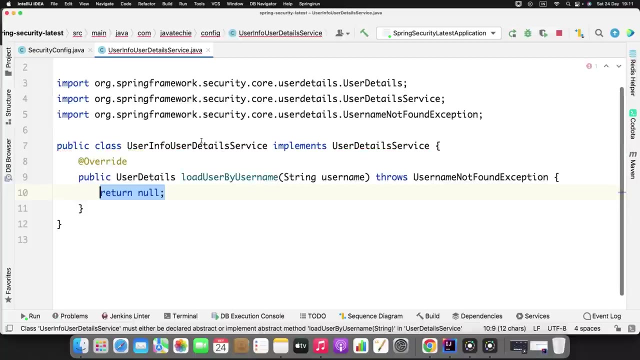 it to the service class service package. now can you see, here i have created a user info, user detail service by implementing from user detail service, because user detail service bin only. i'm creating right, so i will just override a method and i will define this at the rate. 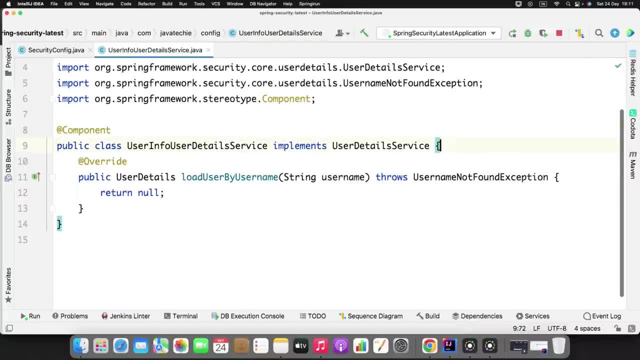 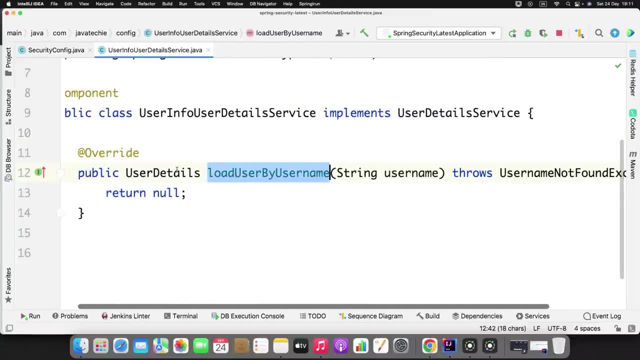 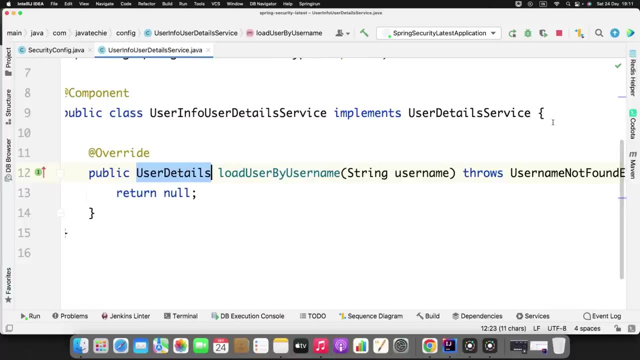 component. okay, so here, if you observe, this user detail service gave me a method to load user by username and give me the user details. but where can i get the user detail object or my user information object? i can get it from my repo, so simply. i need to inject my 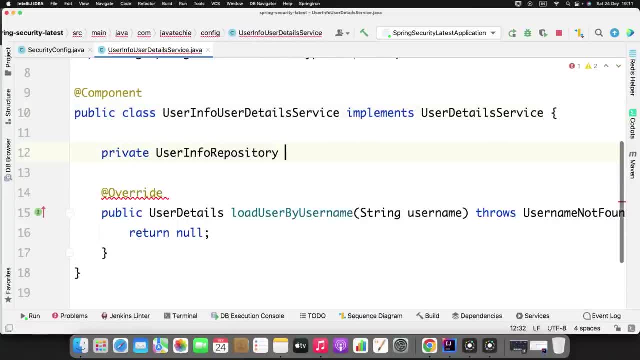 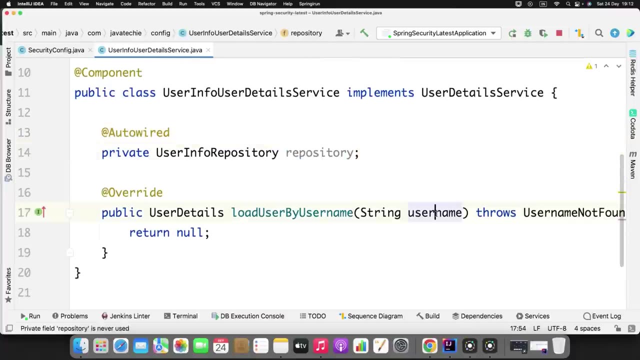 repository here, user info repository. um, i'll name it repo, that's it. okay, i just need to auto edit. fine, just format it now. here i have the repository with me. i will get the username. now i can load the user by username from my dv. so simply for that, what i can do i need to. 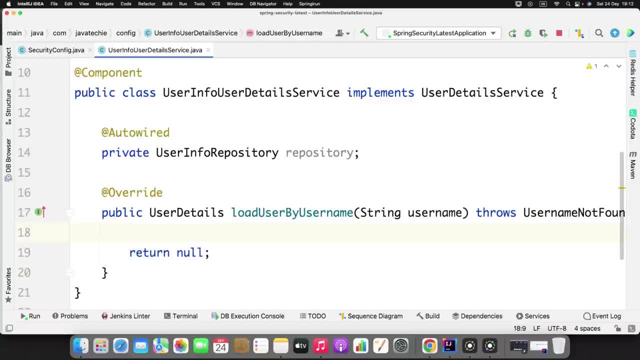 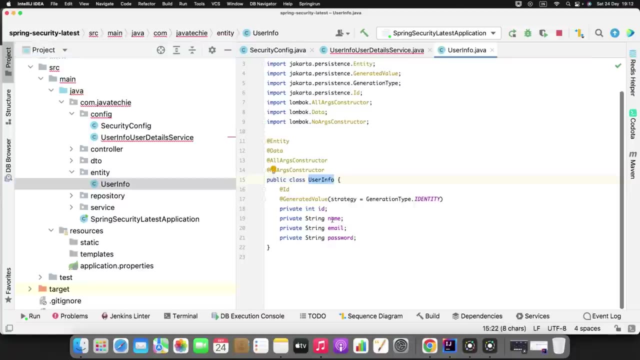 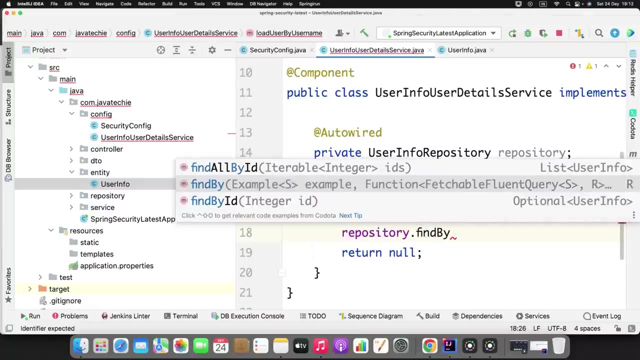 write a method in my jpa right, so i can write repository dot. first let me verify the field name in my entity, which is: uh, what is that user info? i have defined name, okay, not username. it's fine, i can go with that. i can write repository find by name. name is nothing my username. 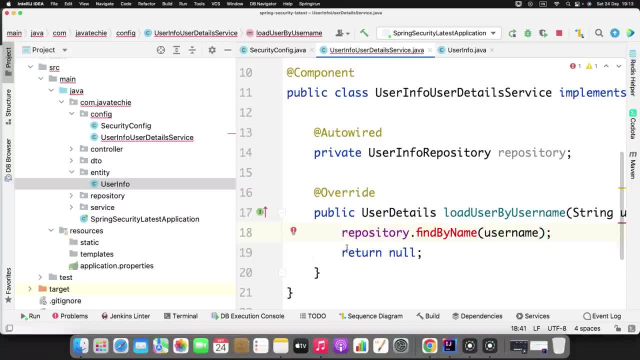 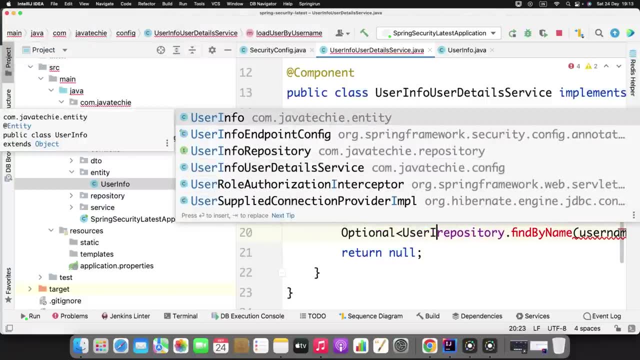 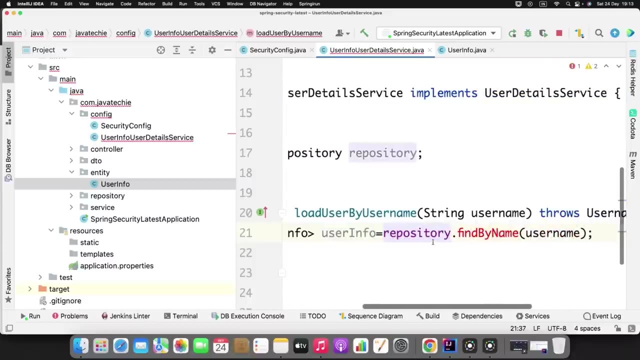 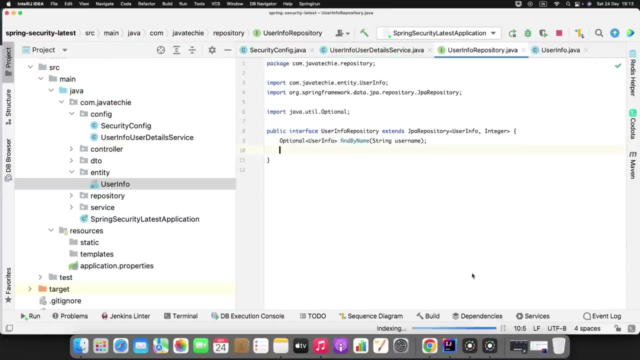 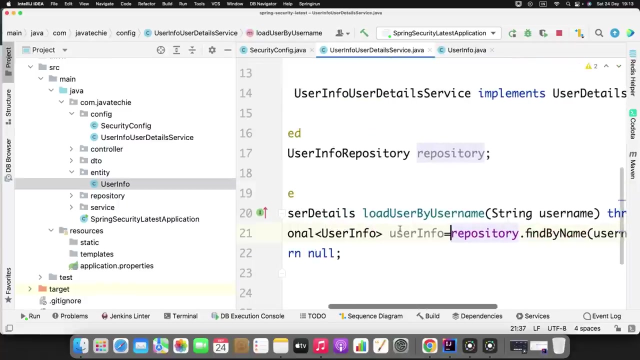 i will give the username and i will expect it to return the optional of user. okay, user info. so i need to create this method: find by name. fine, i have created this method in my repo. now i will pass the user name and i will get the user info object, which is nothing: my entity. 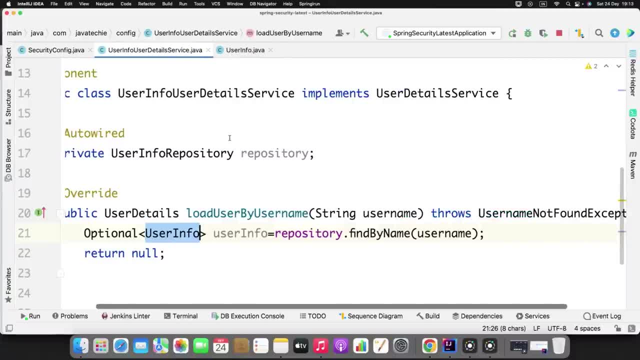 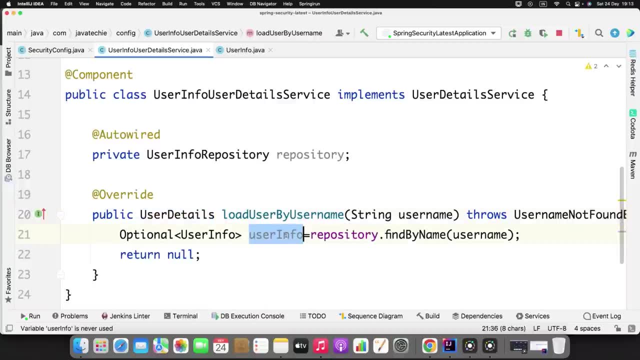 you. but if you observe- let me zoom this- what this method expect me to return: user details object. so it means what i am getting from my dv need to convert it to the user detail subject, then i can return it right. so for that, if you go and check in the user details, 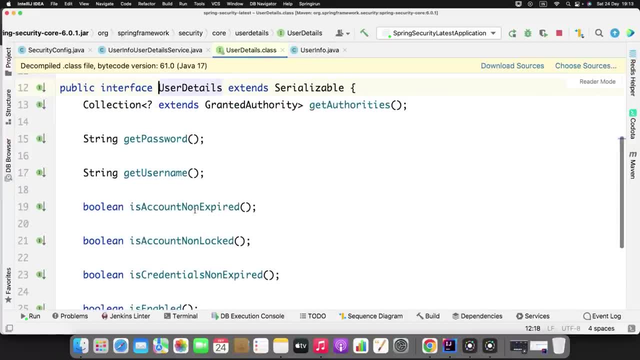 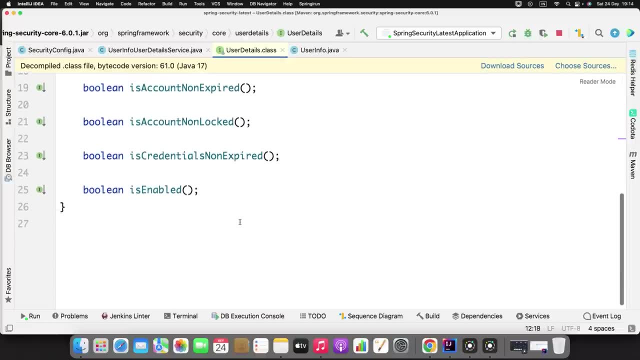 it contains the password. it contains the username when account is account not expired, is account not logged, is credential not expired? lot of things are not expired, so i can return it to the user details subject. so i can return it to of things. it. it is there, right, and also the roles and authority is there, so i need to get each and. 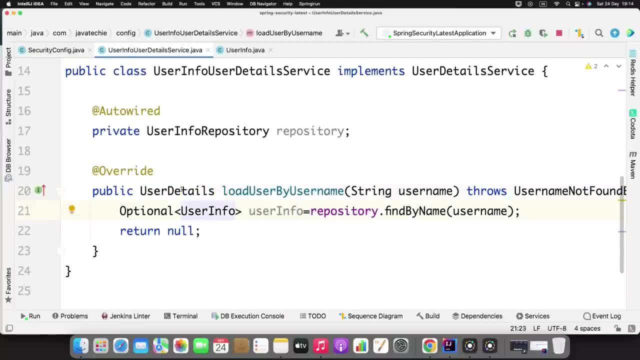 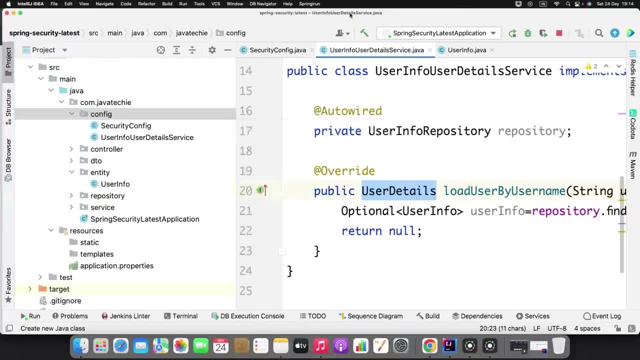 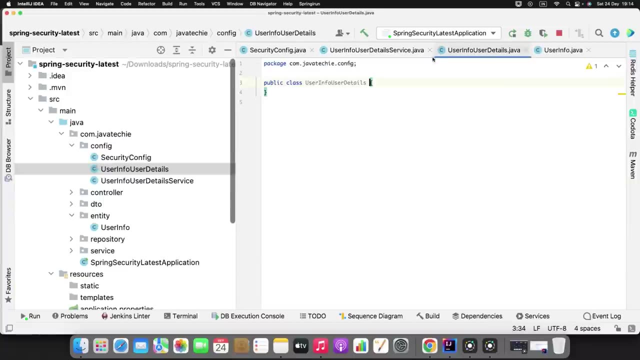 every info from my user info object and i need to convert it to the user details object. so for that i need to create another user details class. so i'll name it user info- user details, because i want to confirm my use. i just want to convert my user info object to this. 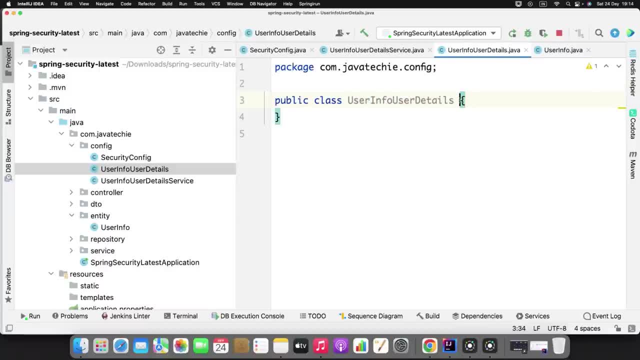 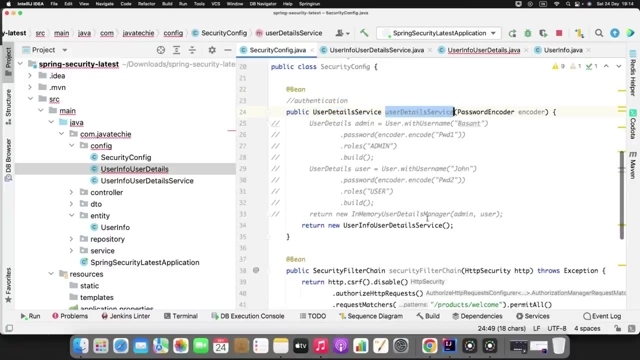 user details object. okay, so that is the reason. i just need to implements from user details. this is the simple as usual flow. it's not something we are doing new here and this is also not the enhancement in springboard 3.0, only the enhancement. we have these two way to define the bin, okay. 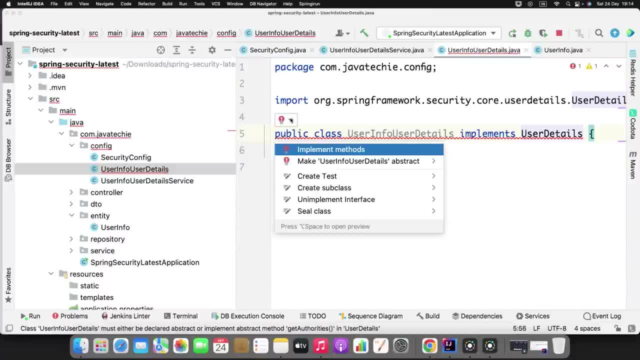 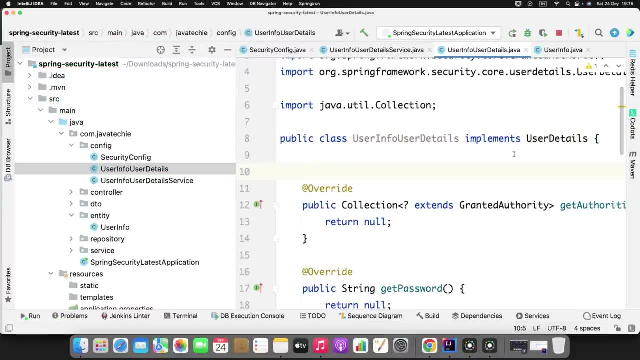 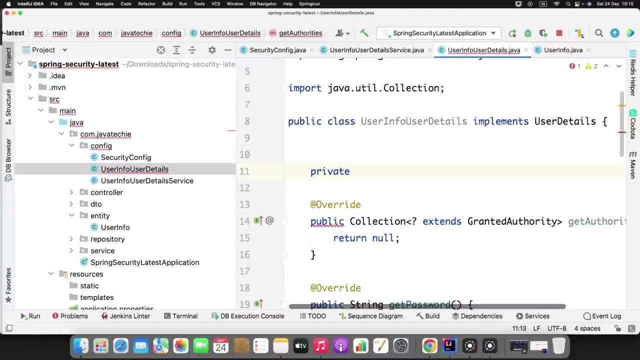 but this is the as usual flow usually we follow while implementing the security. okay, now overwrite all the method and just define all the field, what you want to apply to the user details object. okay, so that is the reason i just need to implement. want to convert to this user detail subject. so i'll just define private. i mean nothing else. 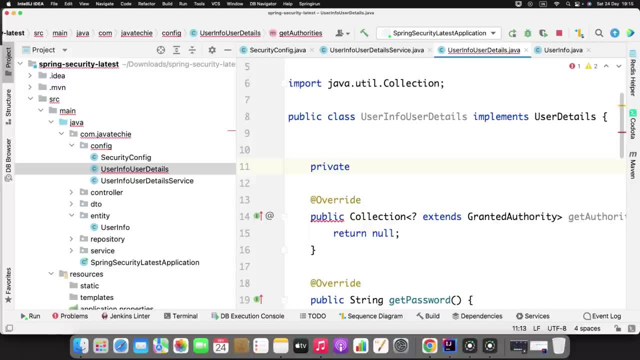 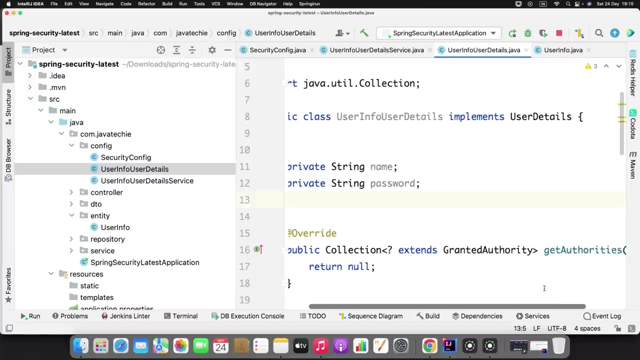 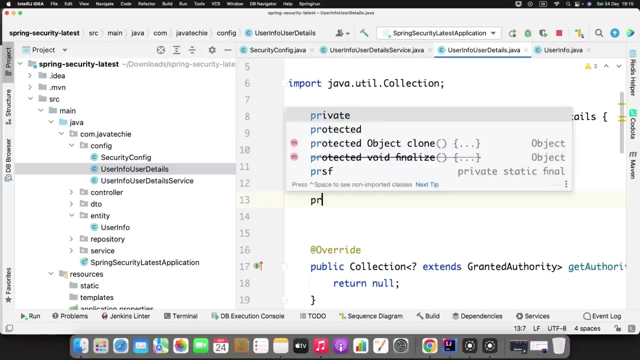 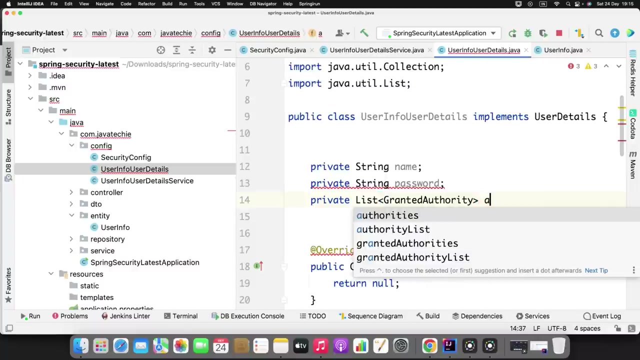 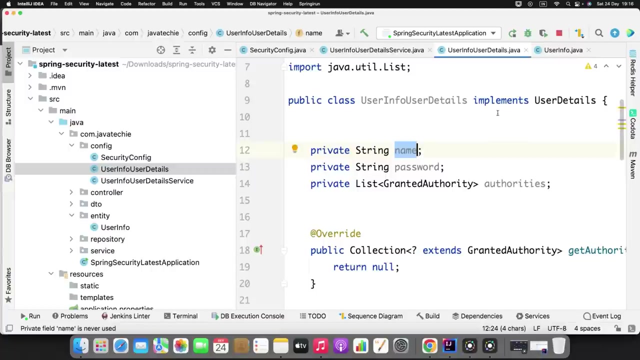 just username, password and your role. okay, i'll define private string. i mean for me name is fine, private string, pwd or password, whatever you are comfortable, fine, the next. i mean i can also define this: grant authorities right: copy this private list of. okay, that's it. now this. i i'll just map my own user info. object. 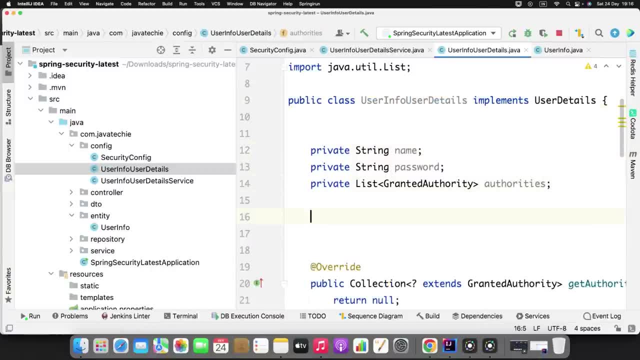 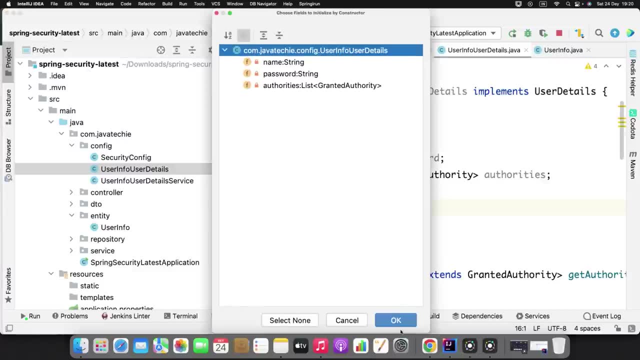 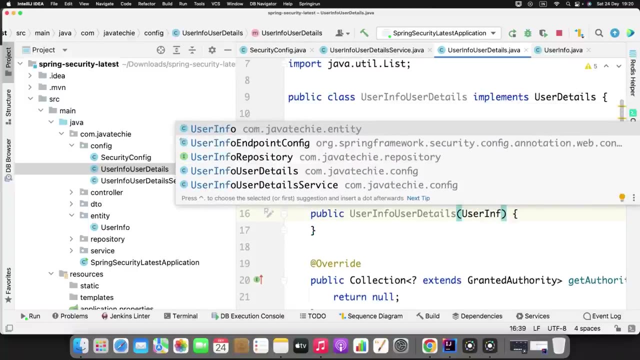 okay, that's it. now this: i i'll just map my own user info object, this particular user details object. so that is the reason i will just define the constructor here: type control, return again constructor. anyway, i don't want to give any attribute because i want to convert the user info to user details. so i'll pass the user info here, user info, and then i will. 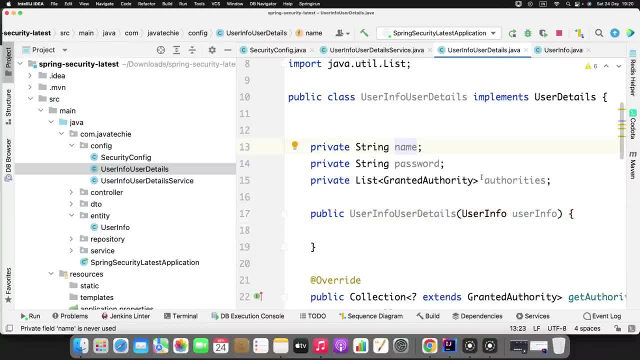 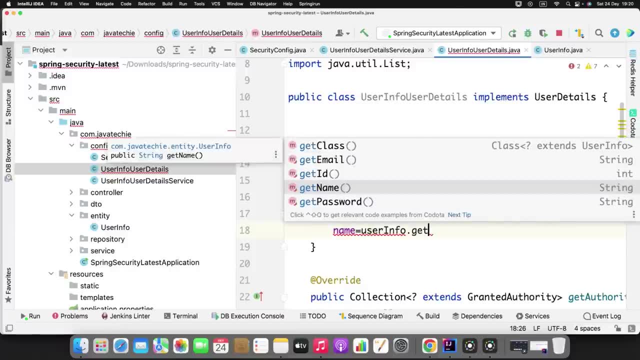 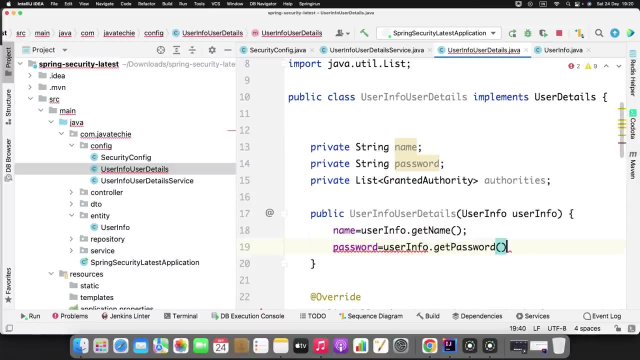 just convert this user info to the required field: name, password and authority. so name: equal to get the name from user info and map it. password: equal to get the password from user info and map it similarly. authorities, right, this is bit tricky part, i mean. anyway, since you can assign multiple. 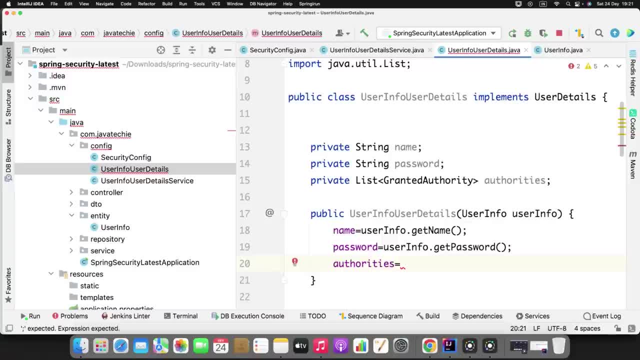 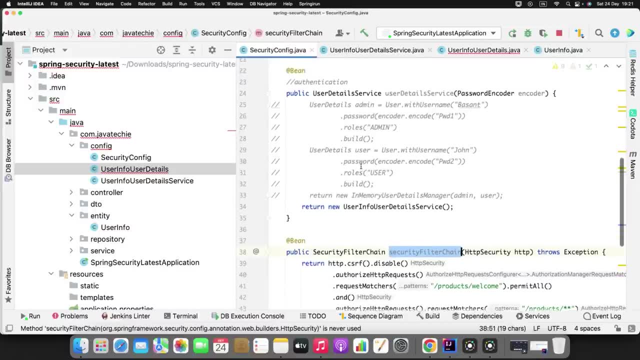 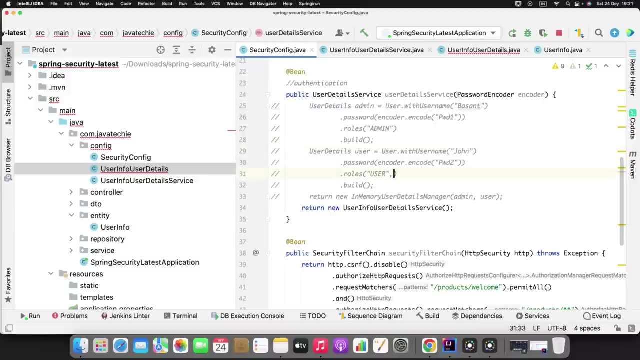 roles to a single user, so it's good to extract the individual role, okay. so let's say, for example, if you'll go and check in the security config, i can define: uh, this, this particular john can be a user and comma, he can be a admin or he can be a. 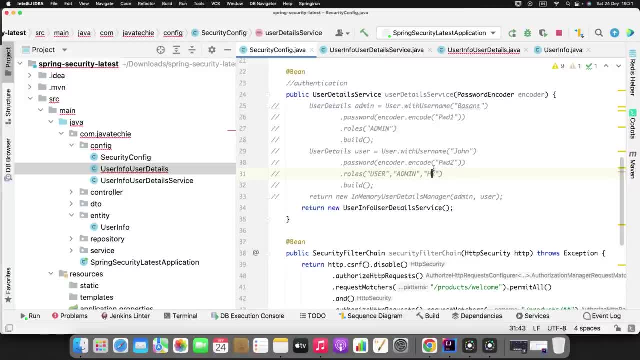 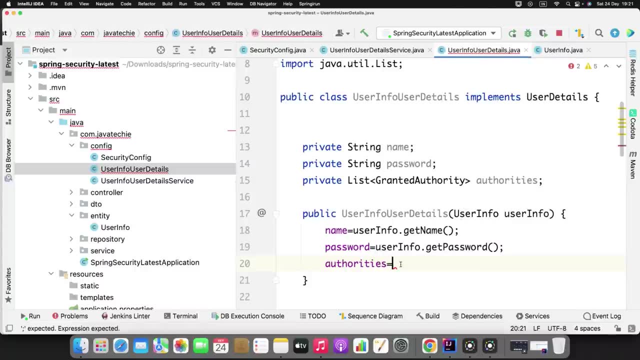 hr. right, i can define multiple role to that particular user. so for that case, what you can do, you need to extract. split them by comma and then extract it. okay, so how i can do that rs dot stream, i will split the roles, okay. um, what is that? 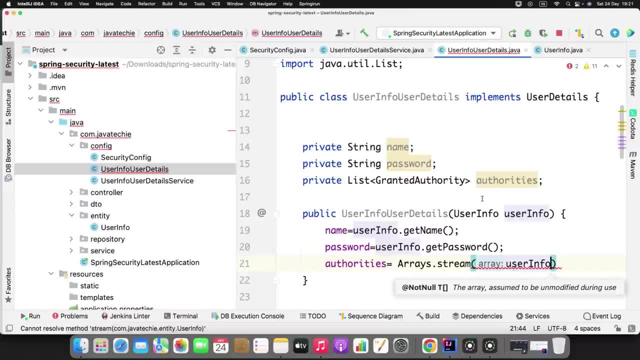 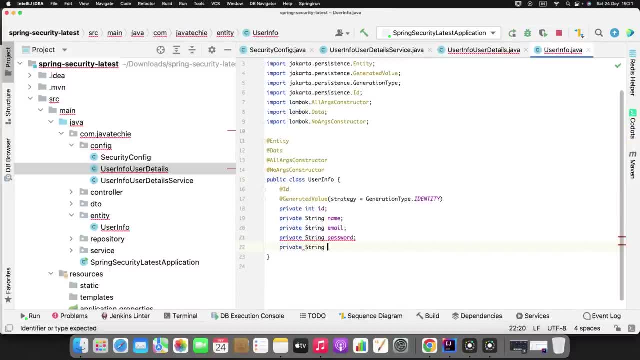 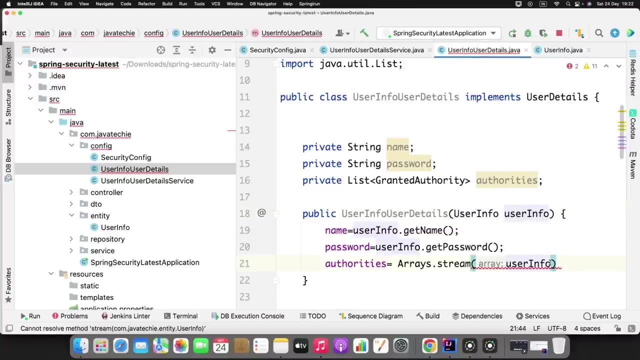 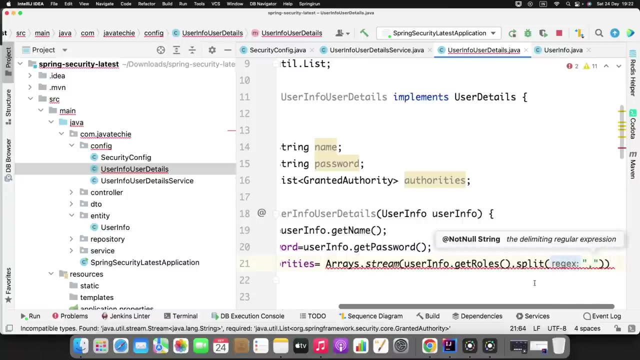 user info. i have not defined the role right, so go to user info. i'll just define the role here: private string rule or you can define rules that's fine. so now we can extract the role here: gate roles, split by comma. okay now, whatever the single roll you will get. 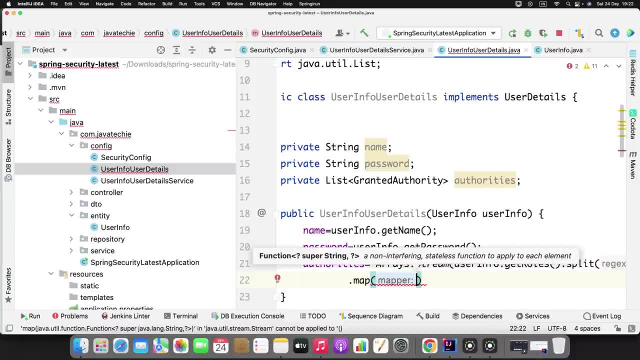 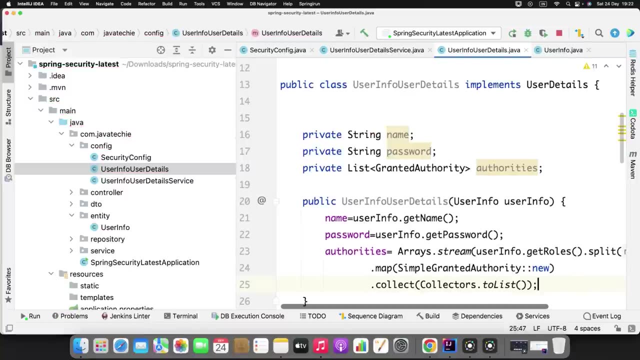 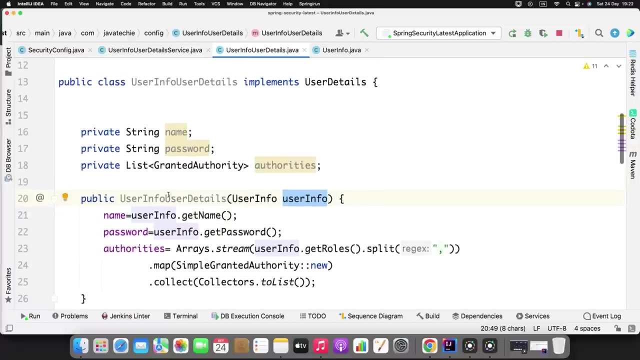 just map it to the simple granted authority- okay, simple granted authority- and create a new object of it and collect it as a list. fine, simple guys. i want to convert my user info to the user details understand by the spring security. so that is the reason i have define a constructor. 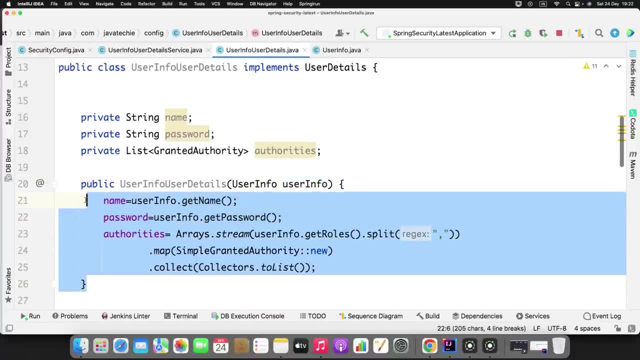 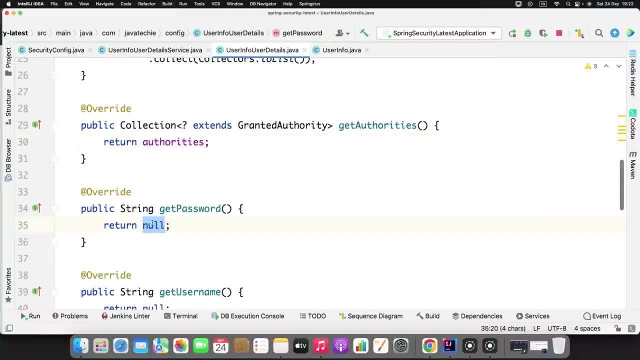 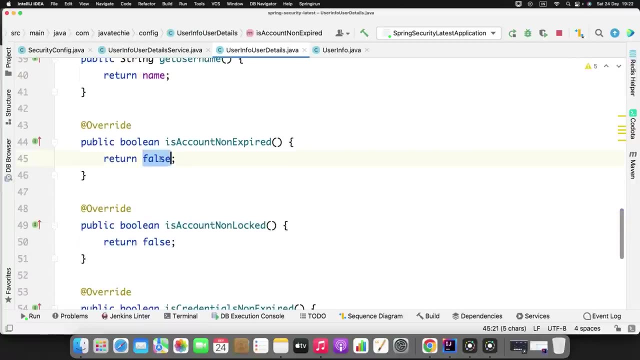 and i am giving my user info and i am converting that to the required field of user details. now i can return here authorities, i can return here password, i can return here what is the name, and i can make everything as it true here. let me copy paste: 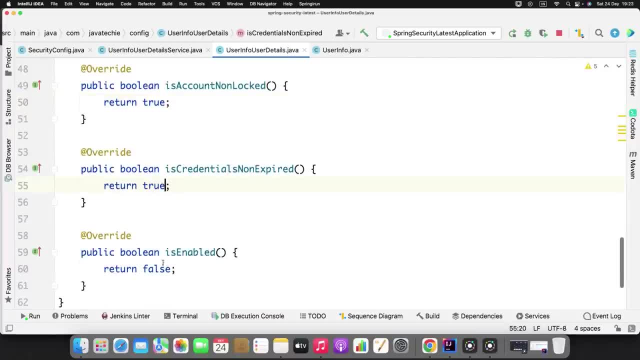 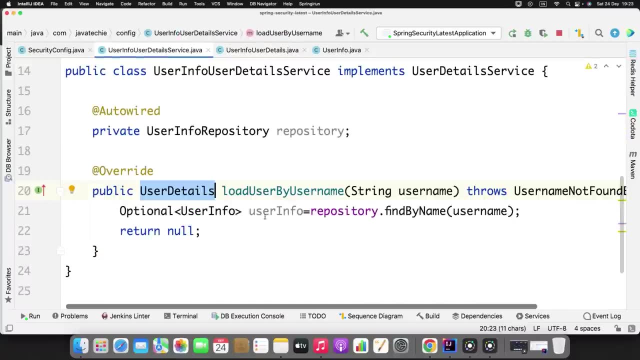 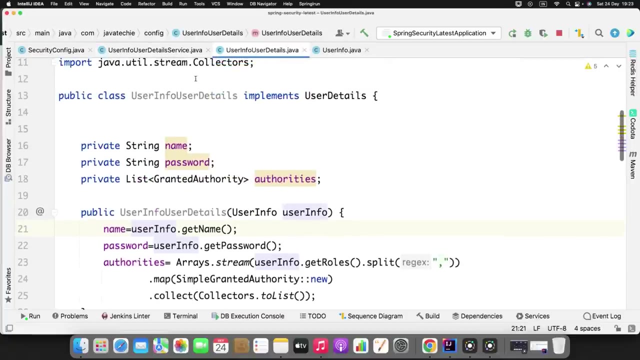 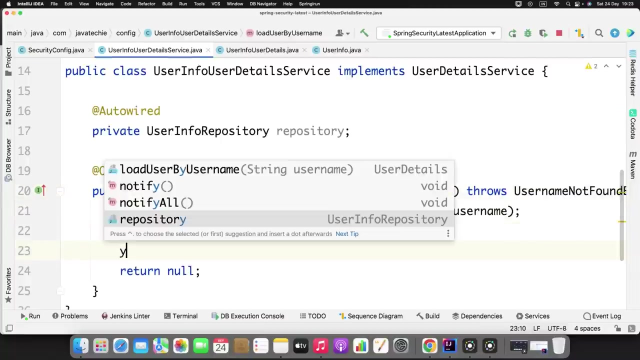 fine, now just go to your user detail service class, your custom user detail service class. now you have user info. just convert it to the user info user details. what you created, that is what the return type of this method: right, user details. so what you can do, simply, you can do user info dot map, since this will return the optional 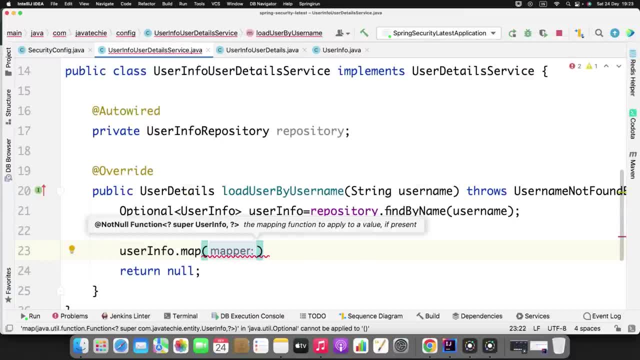 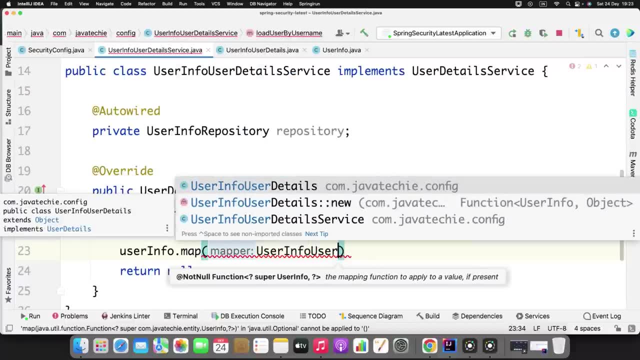 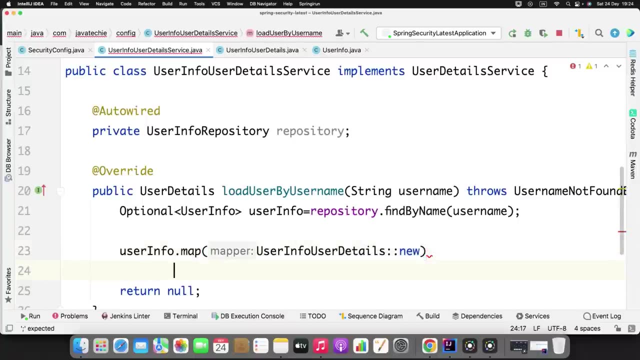 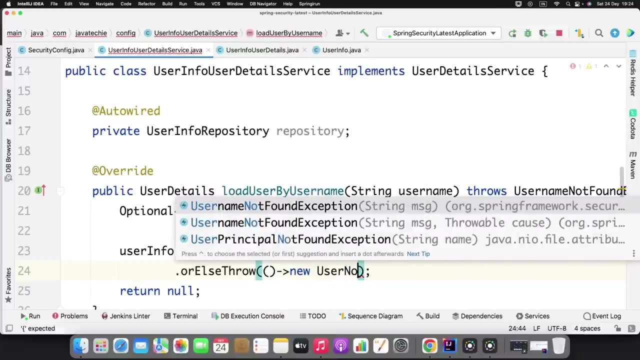 and you can just call the user info user details: user info- user details where it is. create a each object of user info user details. okay, and then i mean: anyway, i just want to validate it or else throw some exception. i can throw something like new user not found exception. 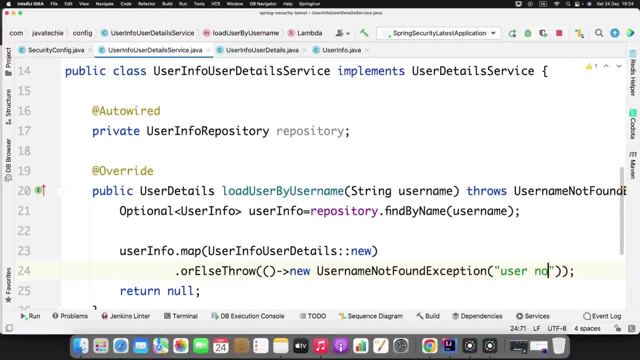 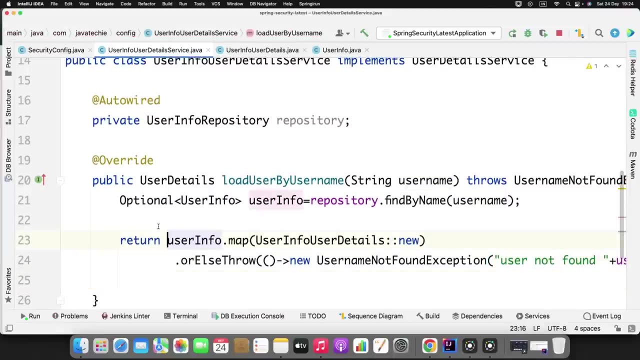 you can give some message- user not found- and you can give the username. that's it right, i can directly return this, just remove this. fine, so i will get the user info from the dv then, since i need to convert that user info which is there in my dv to the user detail subject by giving the username, password and roles and authority. 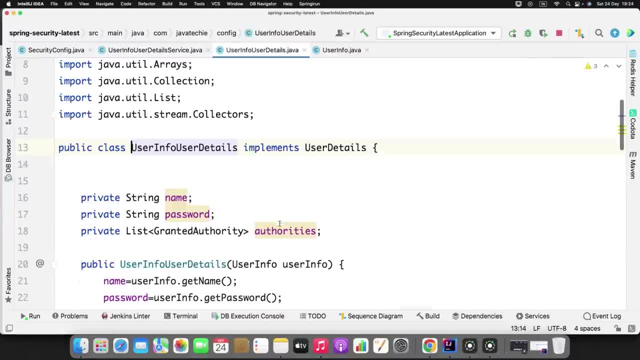 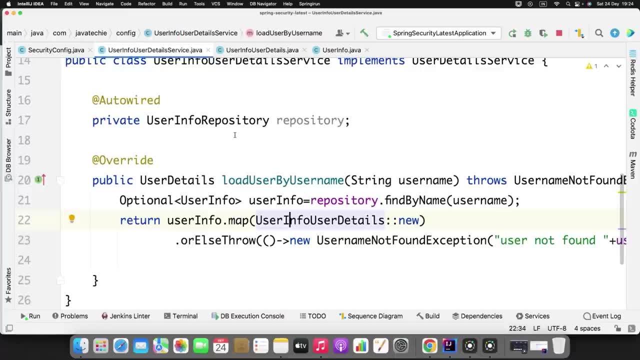 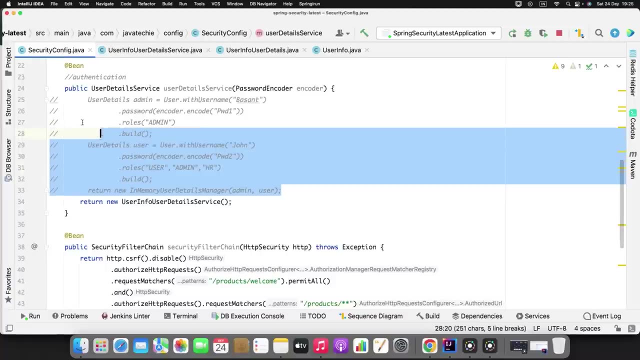 so i am just converting it here. okay, this is the constructor i am converting here. fine, all looks good. now i have given the user detail service in my security config. okay, we are not hard coding the username. now it will use the own user detail service which i have implemented by extending. 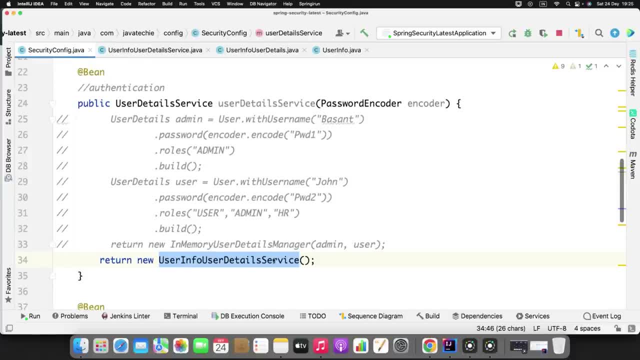 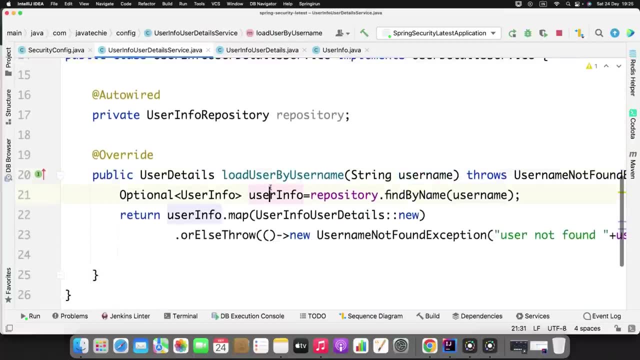 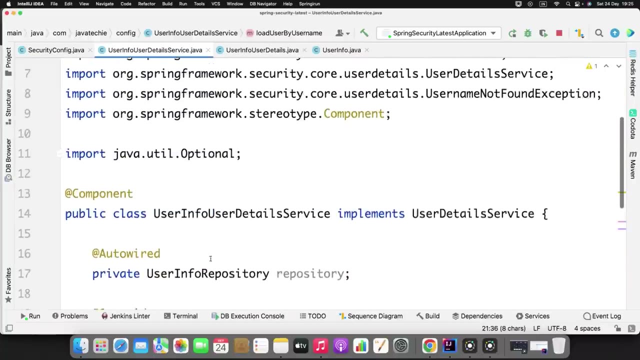 from user detail service. okay, now the request will go to this class and then it will face the user object from the dv by giving the username, and once it get the user from the dv it will just convert to the user info details and it will just do the authentication. okay, so that's it now what we can do for that. i want to store few user object. 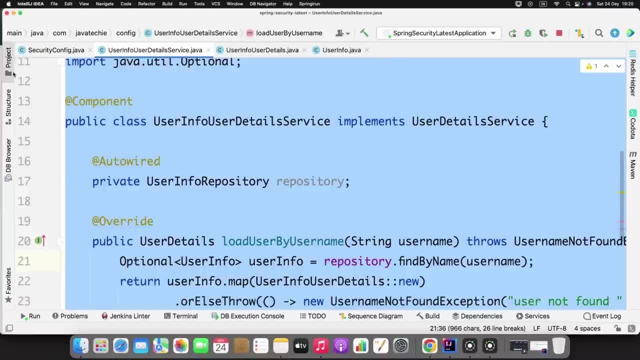 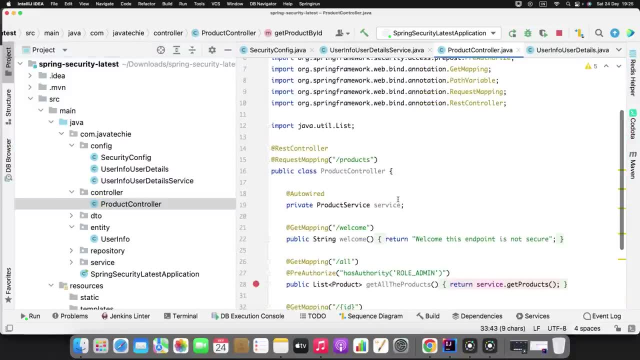 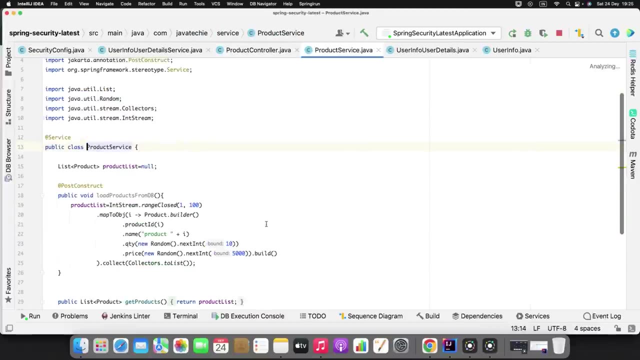 to the dv right, otherwise how i can validate? so for that what i can do, i will just go to the controller and then i will quickly create a new endpoint. let me zoom this anyway, i'll just. since i have the service, i will just go to the service and i will create a method here. 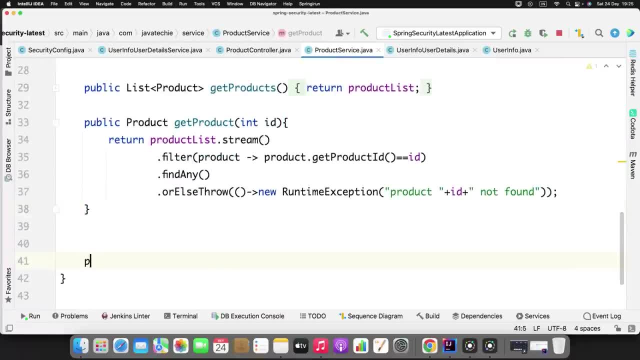 i'll write a method here and then i will just go to the service and i will create a method here. method public, let's say, will return string. ok, or better, i will create a new service. right, why? i will write this logic in the product service. it's fine, you can keep a separate. 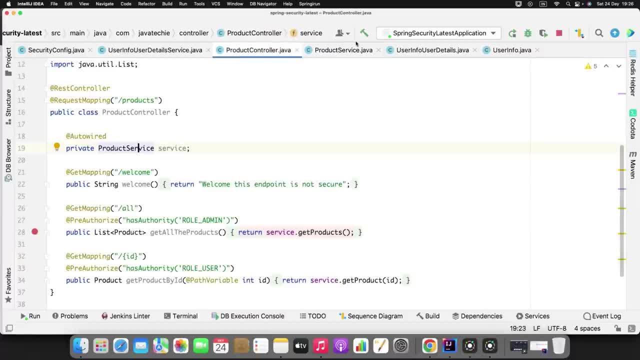 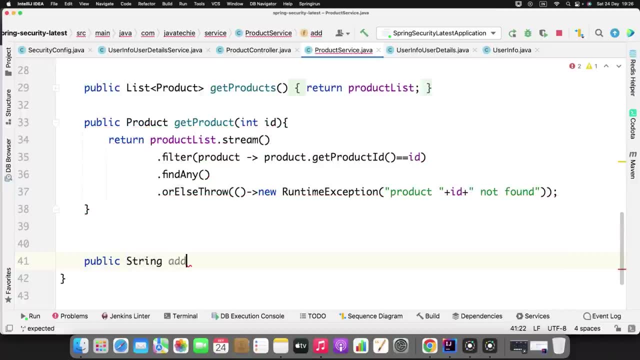 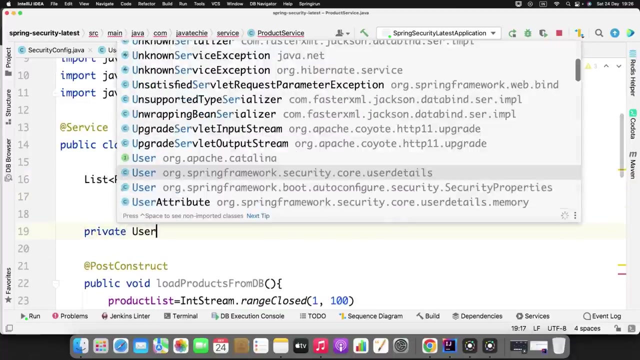 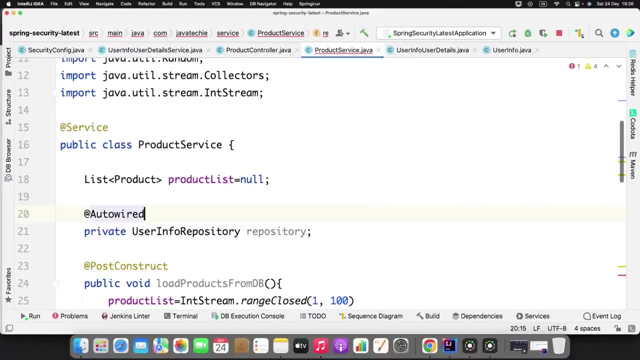 one. but what i am thinking? ok, let's do it here only public. return the string, add user. then give the user info as a request. then i need to inject the repository here, right? so i will just inject here private user info repository repository. i need to auto add it. 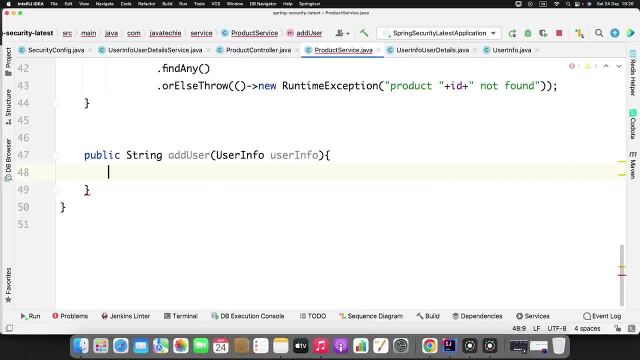 fine, so i just need to save it. i mean, anyway, i am not returning anything. repository dot save user info. but before or while persisting that to the dv, i must need to encrypt the password. so for that, since i have defined the bin of password encoder, i need to inject. 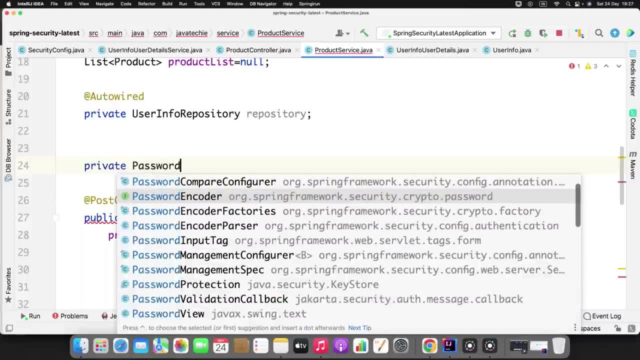 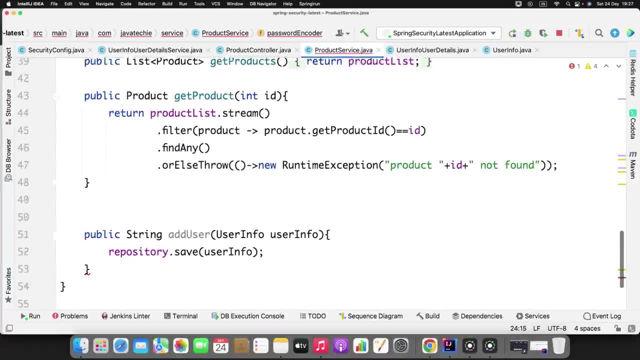 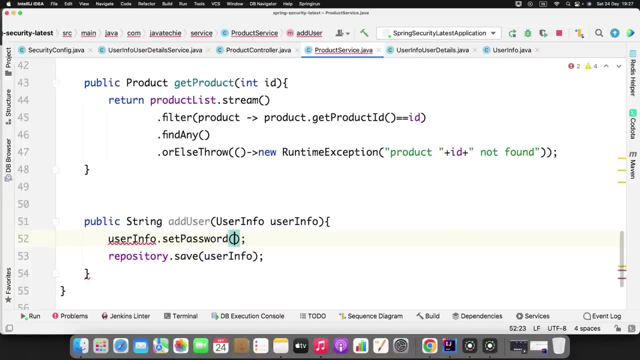 the private password encoder auto add it. so before i store the user info, i just need to set the value: set password. i will use password encoder- dot encode get the password and just encrypt it. user info dot get password. okay, then the value will be modified and store in the dv. 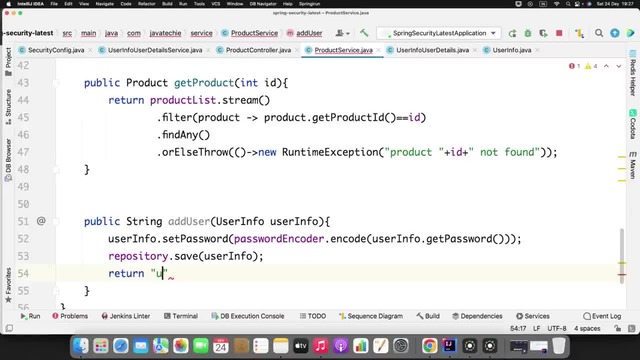 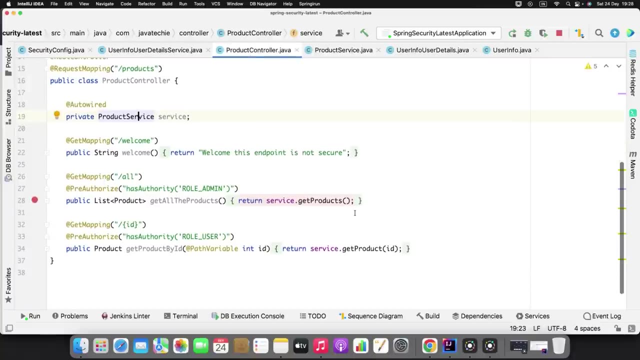 so i can simply return something. user added to system. that's it. okay, then i will call this method from the product controller. i mean you can create a separate user service and user controller but add it here only. okay, it's fine. it's just the enhancement we are learning as part of the 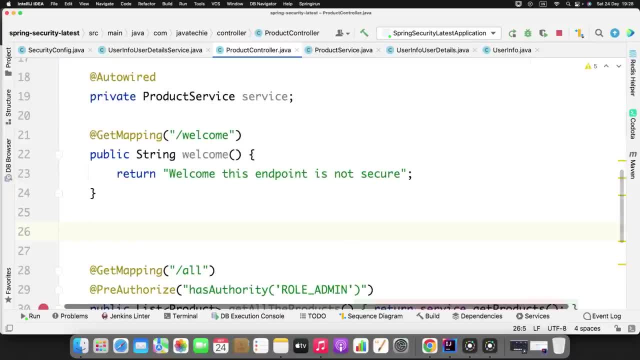 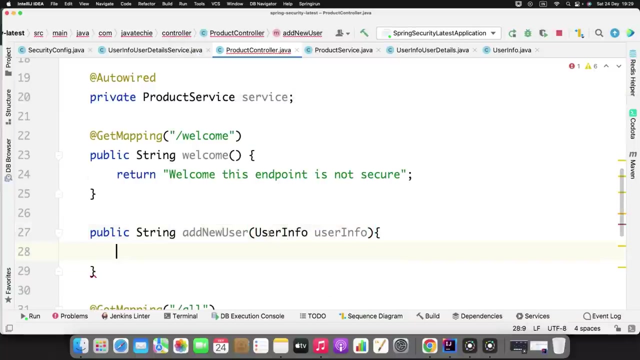 springboard 3.0, so let me zoom this. i will just define here public um string: add new user. i'll just change it to the new user info: user info. then i need to request body. i need to annotate here- this should be the post mapping right, because i need to pass from the postman- 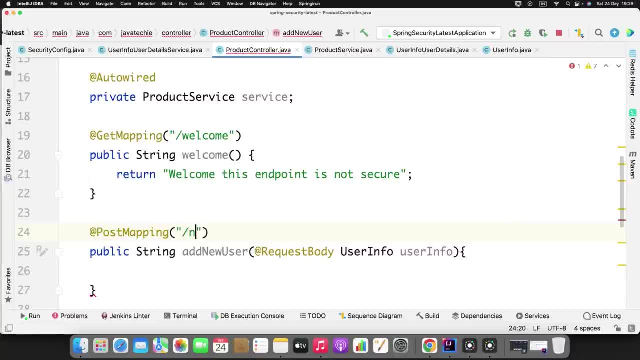 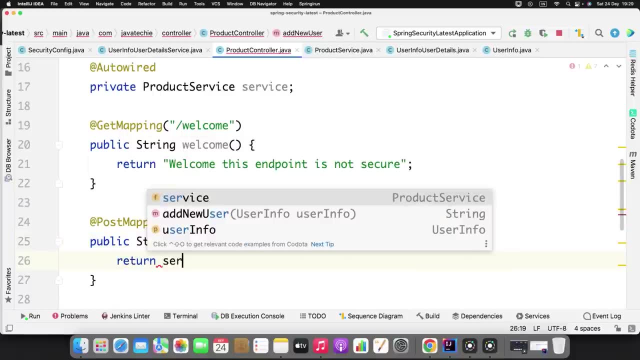 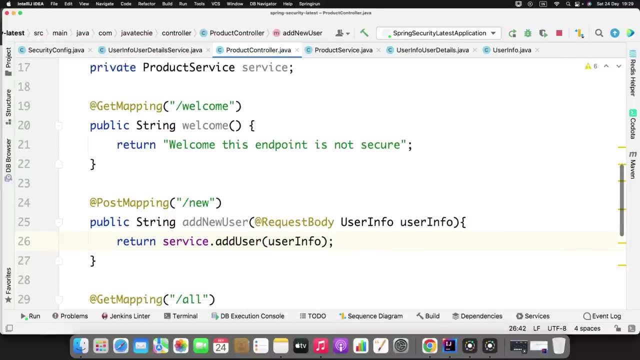 and i'll give the url, let's say new, okay, and i will just call the return service: dot. add user. give the user info, okay, but i want anyone can add a user. so that is the reason i need to bypass the authentication for this method and we already know how, where we can configure the authorization. 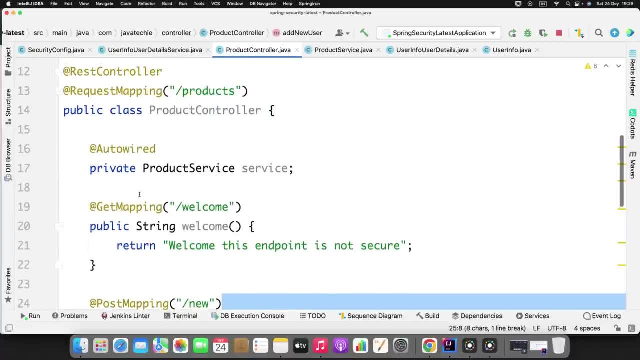 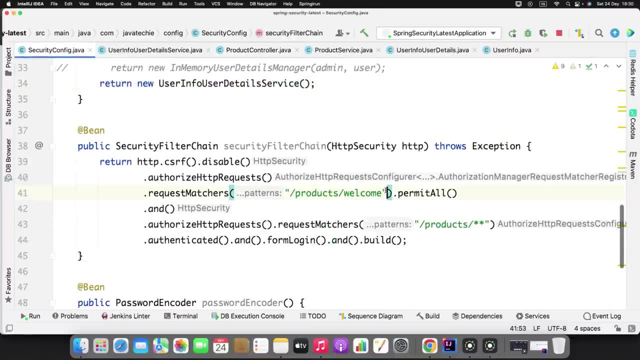 related stop. so i want: if request is coming with slash product, slash new, then bypass it, so i can configure here right. so just define here: if request is coming slash products, slash new, then ignore it. don't apply any security so that user can configure their user details. 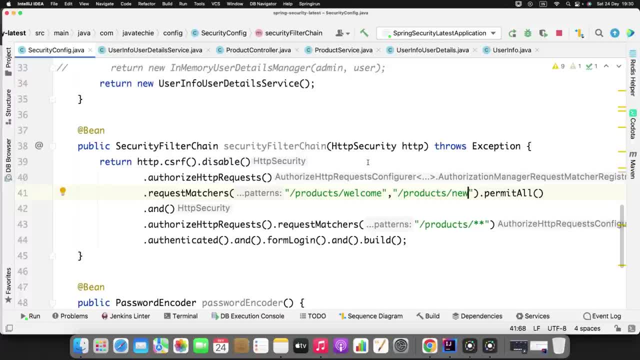 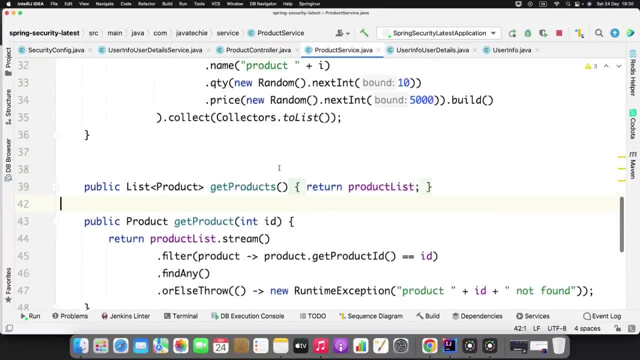 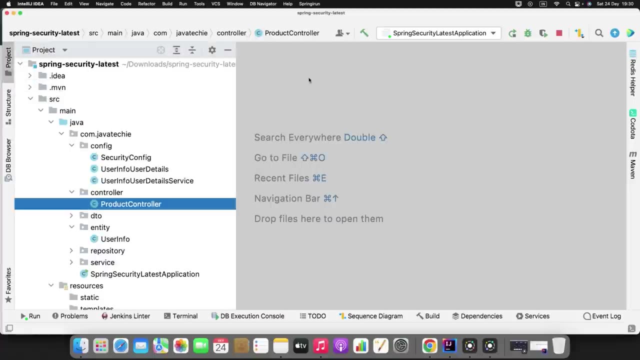 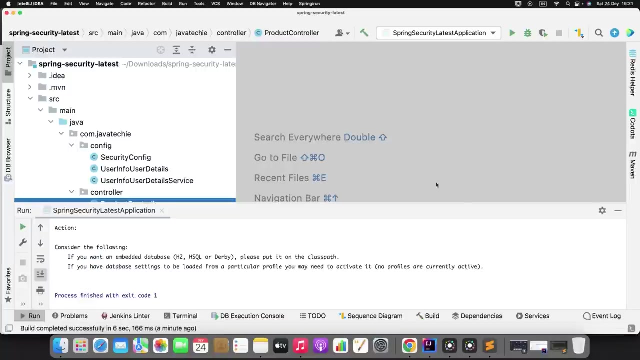 then we'll verify how the authentication and authorization works. okay, so we are good. now go to the product service. all good, okay, let me minimize this. let me close everything. we'll start the application. yeah, so somehow we got the error. what is there here? fail to configure data source? yeah, so we need. 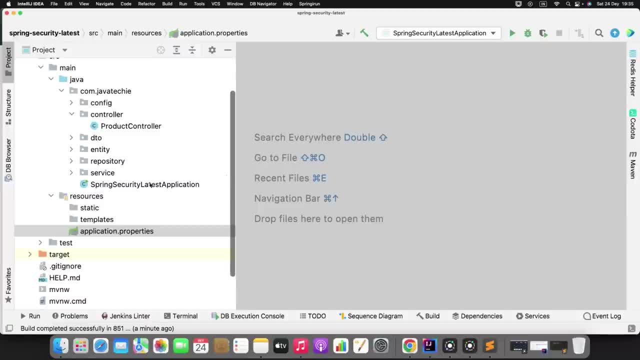 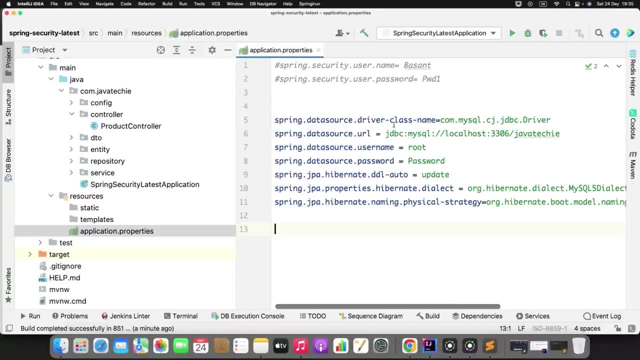 to configure the database or data source related properties in our application or properties or yml file. you need to define driver class, url, username and password, and also you need to add the mysql driver. right? so what you can do, go to the pomxml and add the mysql driver. 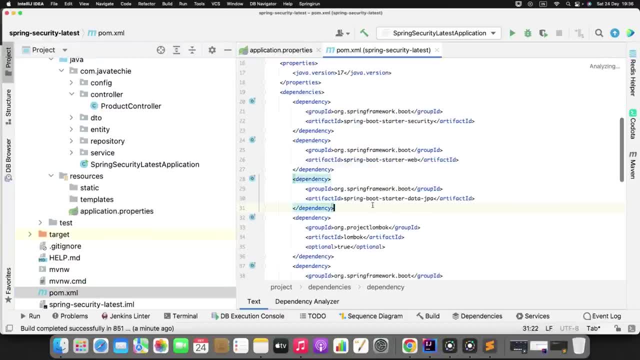 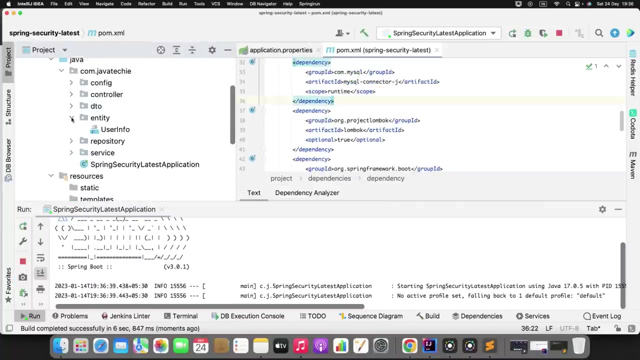 so you can see that the application is not working. so we need to add the mysql driver. okay, now just update it. okay, all looks good. now let's restart the app. first, we need to add couple of new user. for that what we can do, let's build the request. 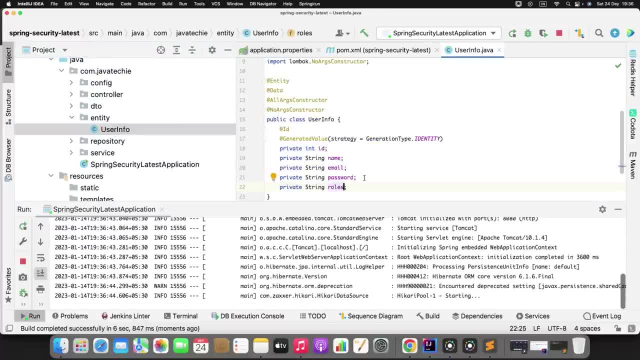 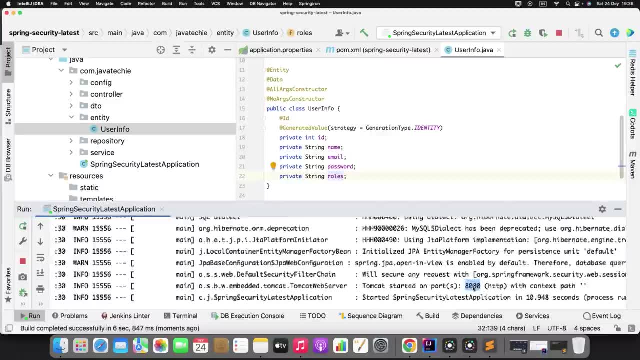 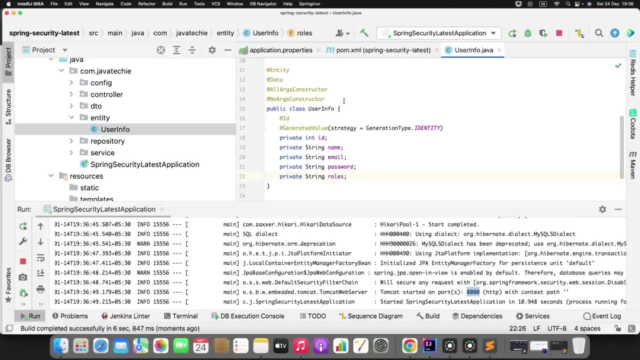 in the postman id will be auto generated: name, email, password and roles. okay, so let's wait it to start. yeah, it started on port 8080. now we need to add few user objects, so i'll add the same basant and john, so same what we have hardcoded we'll store in the dv and we'll verify. so just open the postman. 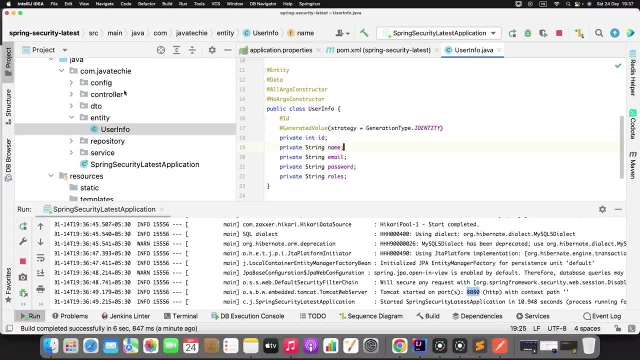 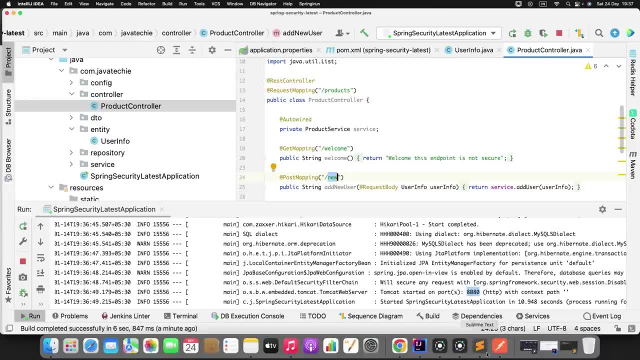 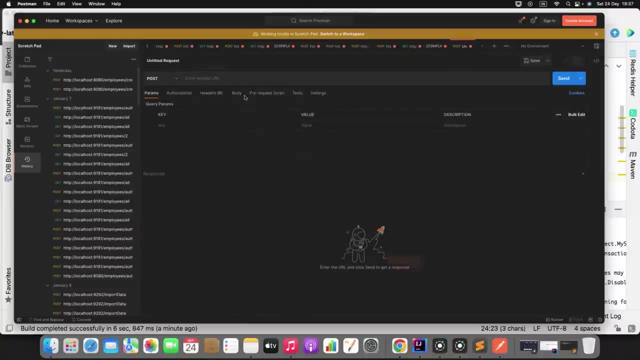 i will just copy the url. i mean go to the controller class new. right, let me copy this slash product slash new, new request, which will be the post. i will just add the url: http: 8080 products slash new. i mean, again, we need to define a separate controller, but it's fine, we just added. 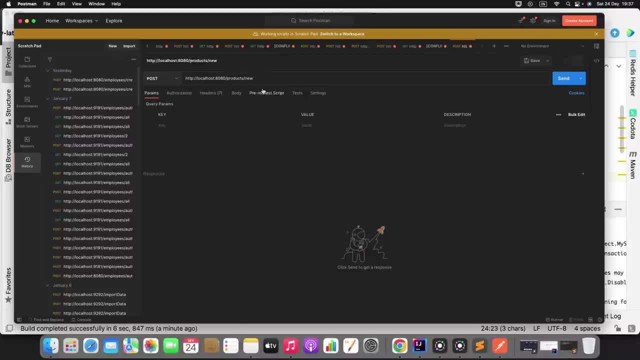 in the same controller. okay, in slash product, slash new, we should not add any user. this url is meaning less, completely right, but try to consider this for demo purpose. okay, don't ask me in the comment whether this is the correct practice to design the code or not. now i will just add the user object in. 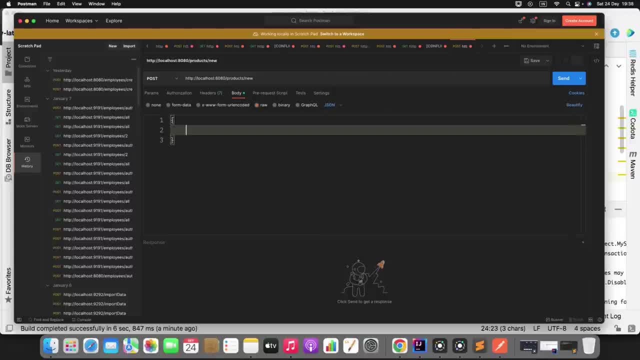 the form of json. so what is the user? i need to add name, let's say basant, then i will add password, let's say pwd1. email i'll give, let's say basant at the rate, emailcom or gmailcom. fine, what else field we have? 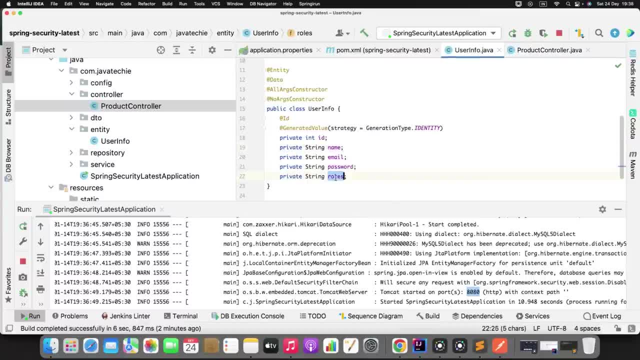 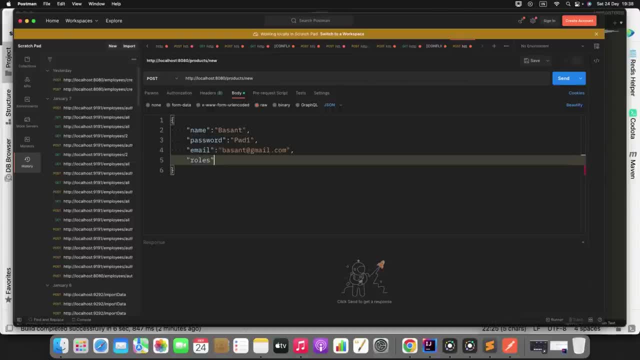 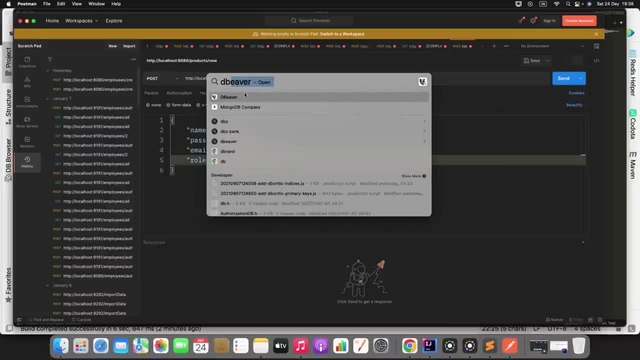 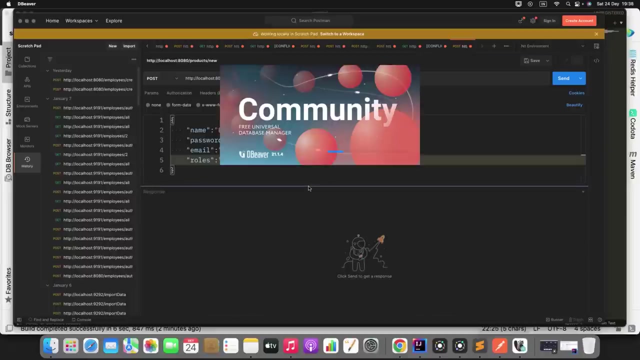 roles, right, roles i need to define. so let's say, my role is i'm a admin. okay, so this is what. so let me know, let me open the dv here for this slash new. it should not force me to authenticate because i bypass it, so let me send. 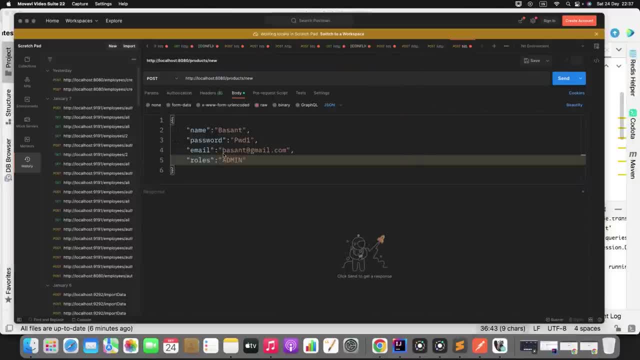 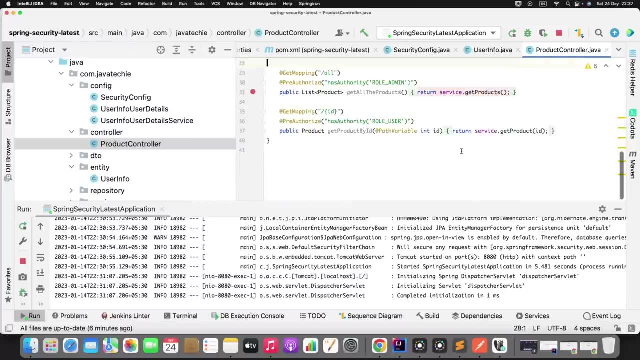 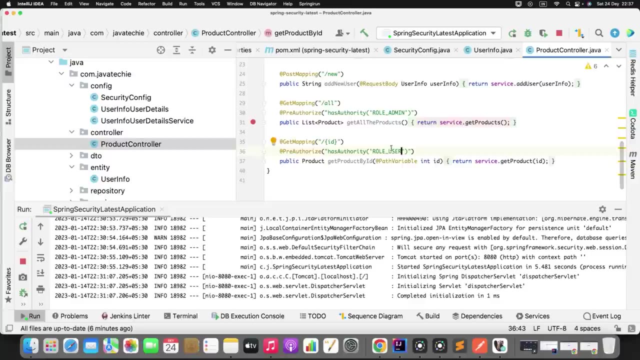 the request. before i send the request, let me change the roles to prefix. role underscore admin. okay, because that is what, if you observe, in the controller class we have specified here authority role underscore user. so i need to add the prefix because at the end, if you will check the 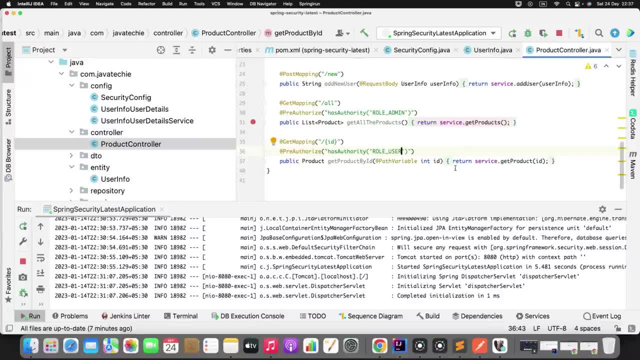 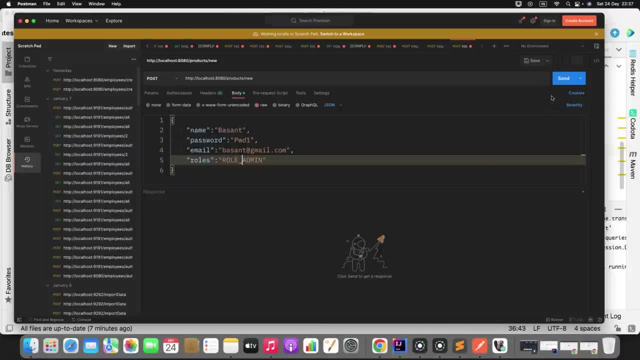 or if you will debug the internal code of authentication provider, it append the prefix as a role underscore. okay, so i'm good now i will send the request. just hit the send, so user added to the system. let me add another user, john, whose password is pwd1. 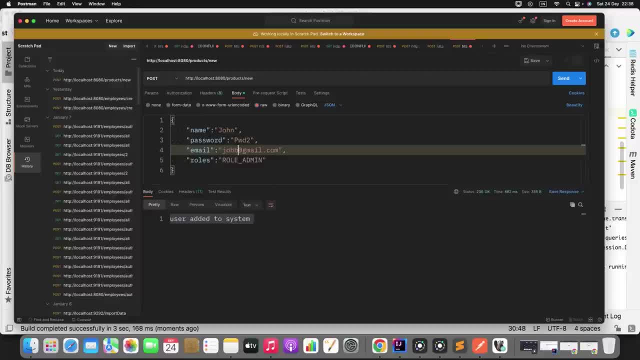 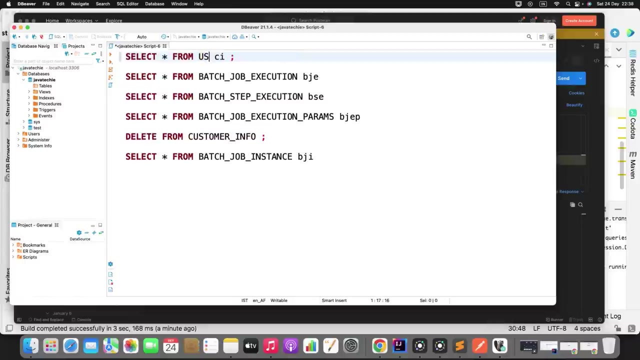 admlid is john at the gmailcom and roles is user. okay, now let me send the request. now we added two user: basant as a admin, john as a user. now let me verify in the db what is the table name user. first let me refresh. 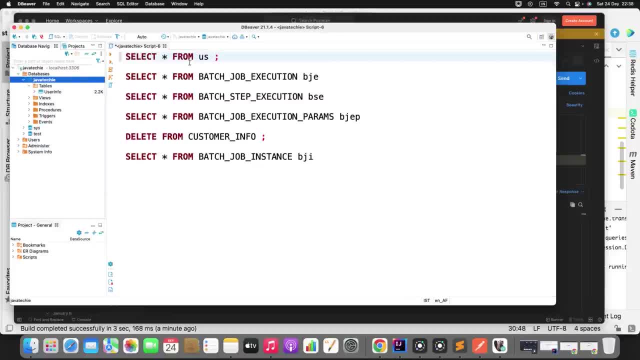 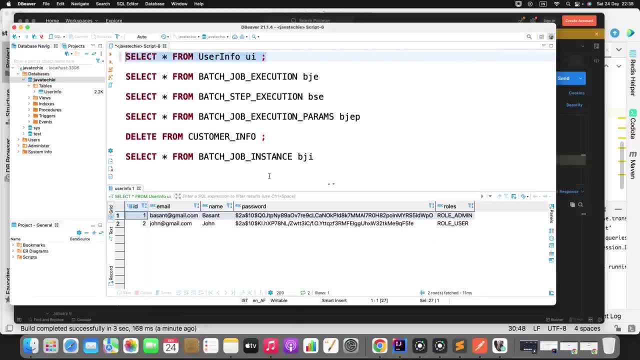 the schema. okay, user info: is there, right? user info. let me run this. can you see? here we have two user, basant and john. password is encrypted. basant role is admin and john role is user. now, all good, we have the record in our dv. now let's try accessing with these two user, okay. 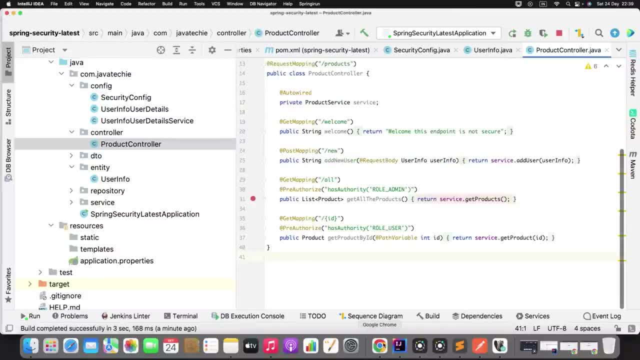 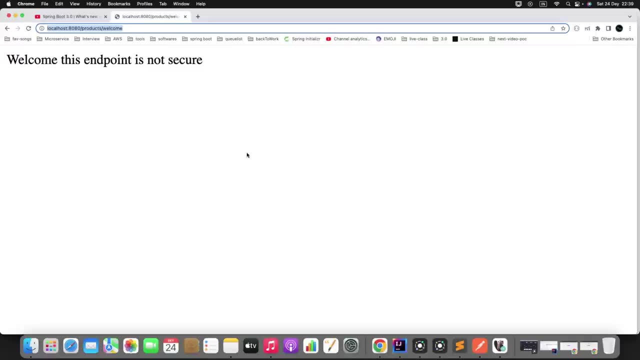 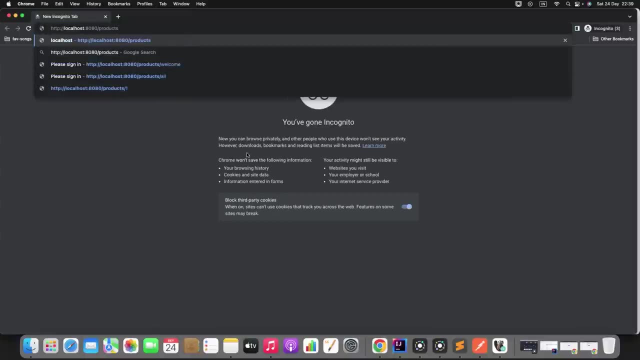 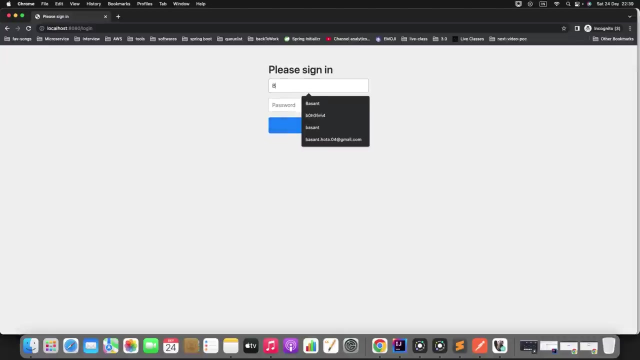 so first i will go to the browser, i will copy this so i will try to access the slash all product. okay, so only admin can view slash all product. so i will open a new terminal, all. so first let me try with the john, okay. or let me try with the basant. basant is the admin. so 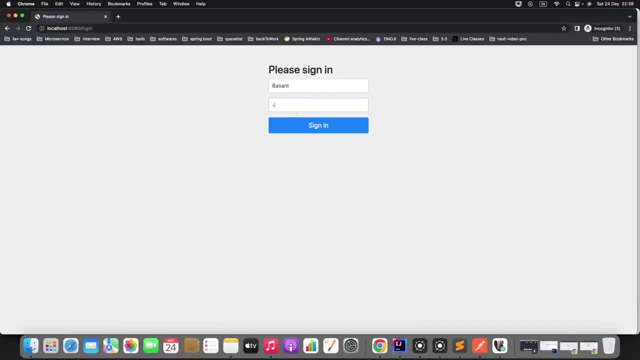 he should able to access this endpoint, pwd one. but before i hit this, we'll get one exception. okay, by seeing that exception we'll understand what is the need of that particular exception or how we can resolve that. click on sign in. can you see? here we are getting the option. i mean the exception, no authentication. 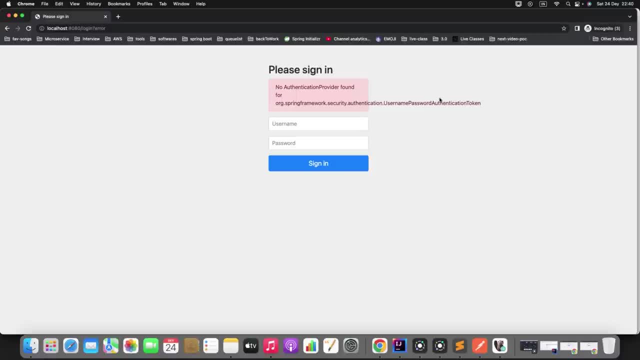 provider found for this username password authentication token. okay, so we have defined the user details service, who will talk to the dv and validate the user, but we also need one authentication provider. right, only the authentication provider will talk to the user detail service, so we need an instance of authentication provider in our code. so let me copy this: go to your config file. 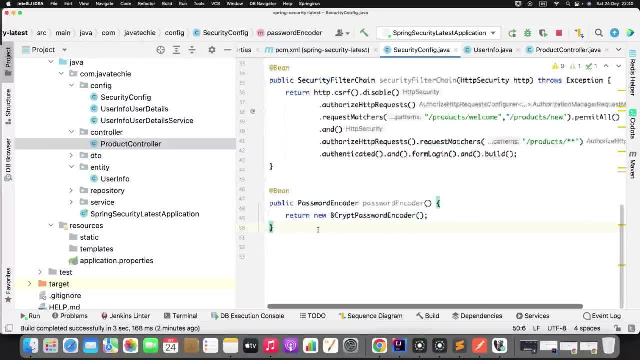 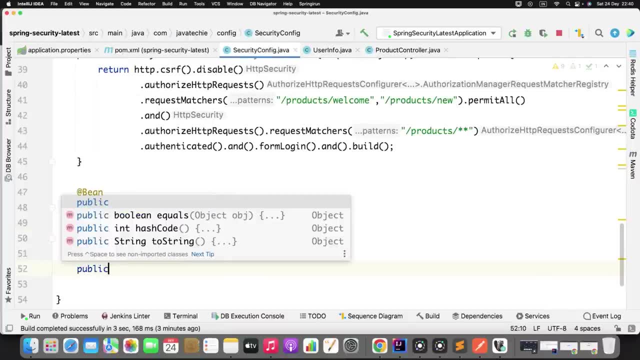 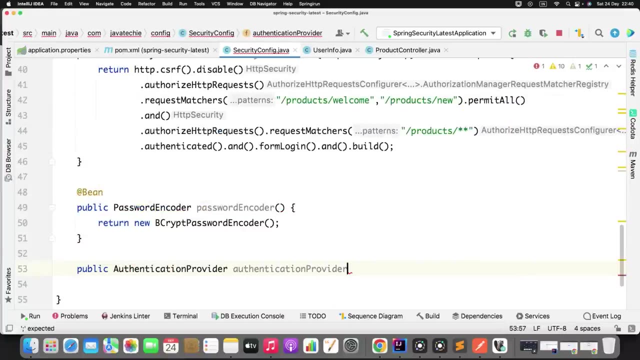 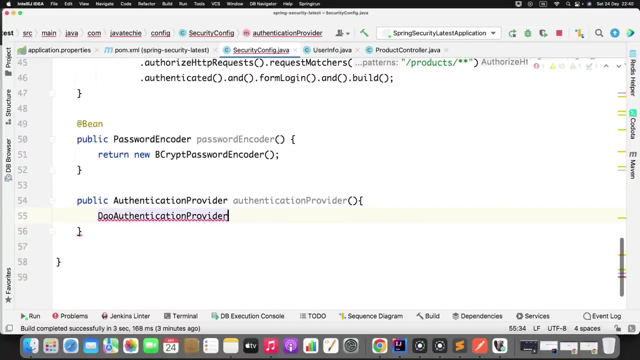 security config. let me zoom this for you then what i will do here. i will just create as spHello where we are loading the application. there you can see that i have called the slash authentication provider in manual connection. now there you can see that basically the authentication provider is in manual chicken, so you can check click. 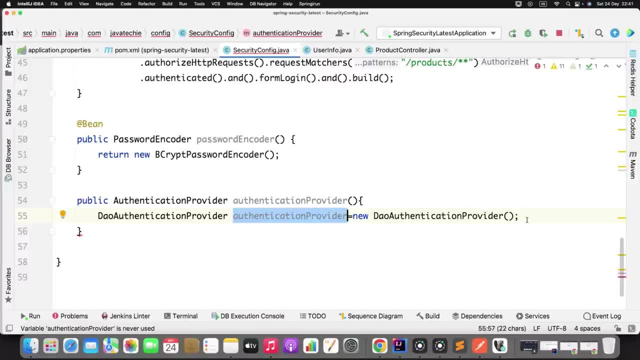 there's a warning. blue dot is our addressing data there you can like that. it will salty like this. you will get a notification is gone later. this is before that indicated's. here you have zip file. has to be чис file picking. here we will provide theShell folder calledacles oforercom and definitely there is an authentication provider which is being 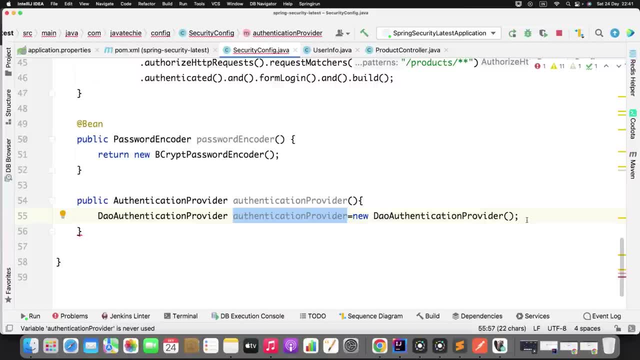 we can give to the authentication provider. authentication provider will talk to the user details and generate the user details object and it will set to the authentication object. that is what the internal flow. okay, so do let me know in a comment if you guys want to know about the. 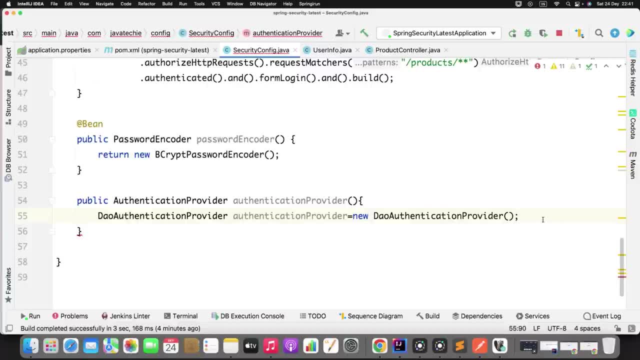 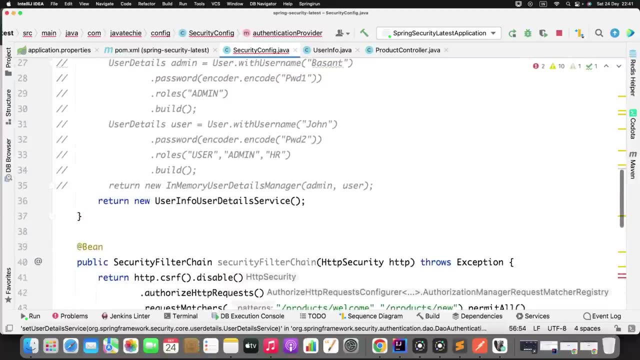 internal flow. already i uploaded one video about the spring security internal, but it seems the classes has been changed. okay, so let's do that. authentication provider: i need to set the user detail service. who is my user detail service? already i created, been a fit, right. this is what. 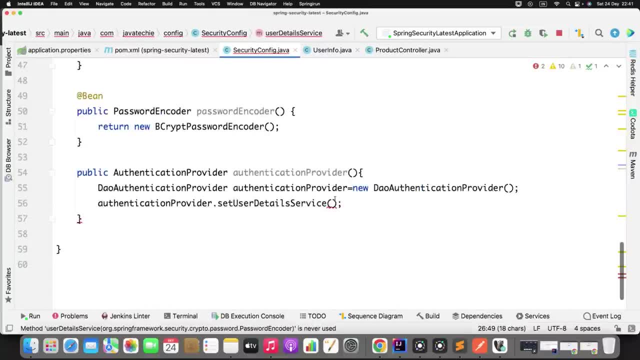 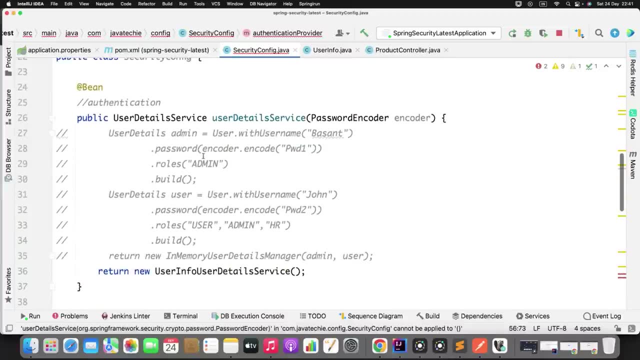 my user detail service been, so i will simply call that. it is asking password encoder as a argument, which is not required for now, because anyway, we comment out this code right, we are encoding the password in service layer so i can remove it, so i will just pass it now. now, next authentication. 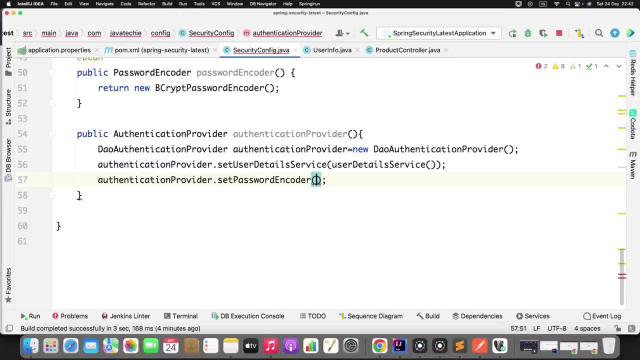 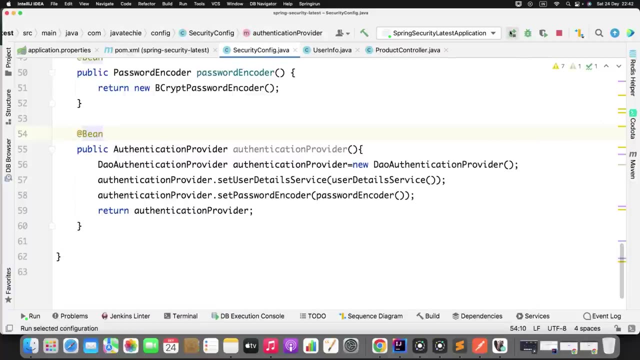 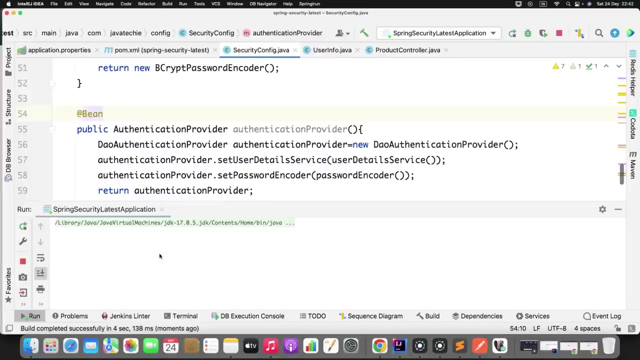 provider dot. set password encoder. give the password encoder, that's it. then just return the authentication provider. okay, and i need to annotate here at the red bin: that's it now. let's quickly restart. so this kind of configuration you no need to add if you are using the. 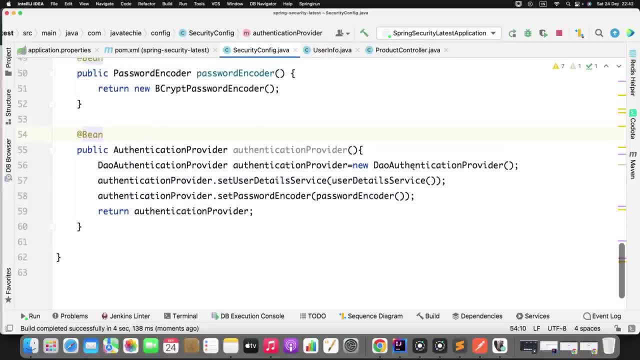 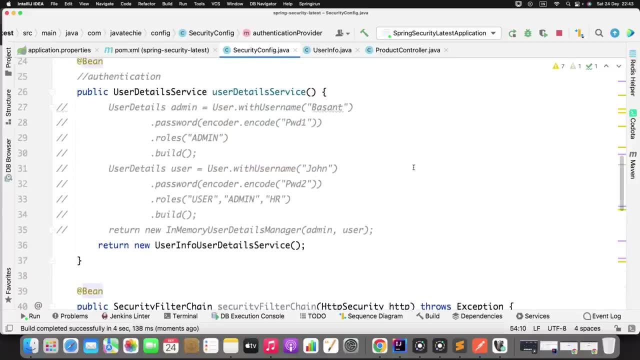 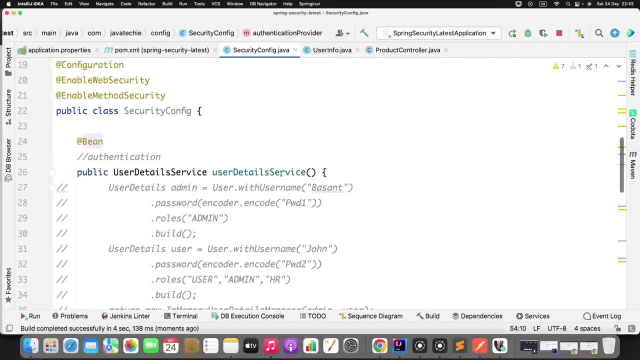 spring boot 2x version. still, you can play with the security configure adapter and you can over write the configure method which is overloaded method and you can directly play with that. but in spring boot 3.0, each component of this security flow, you need to create a bin of it user detail. 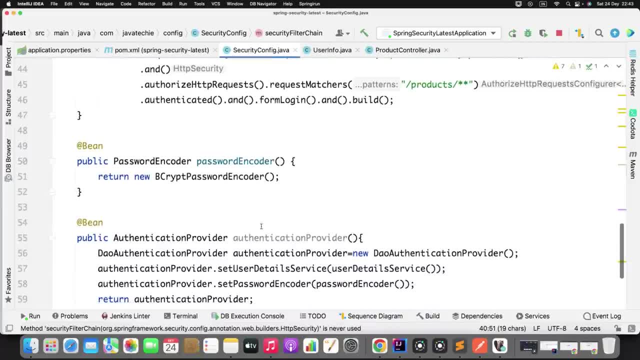 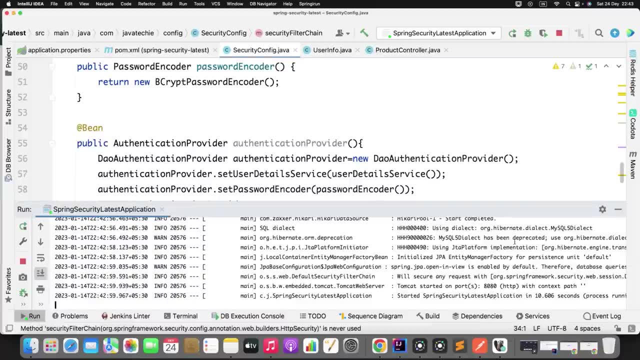 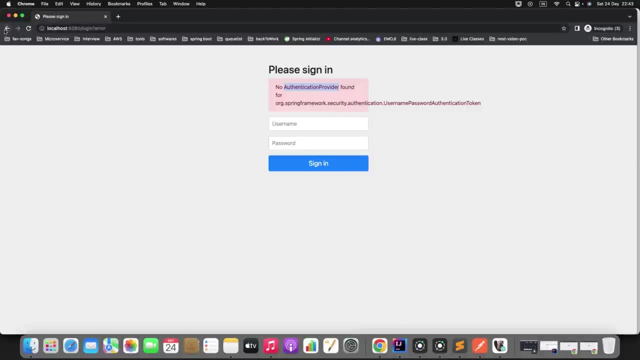 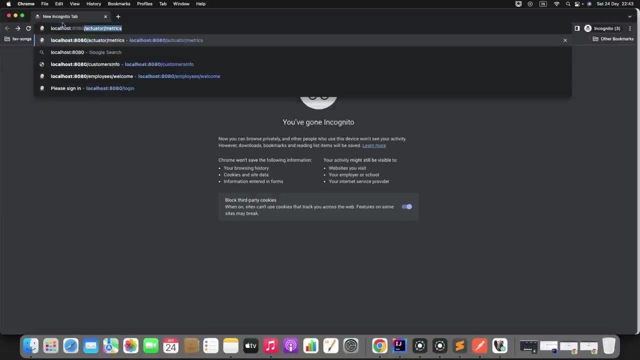 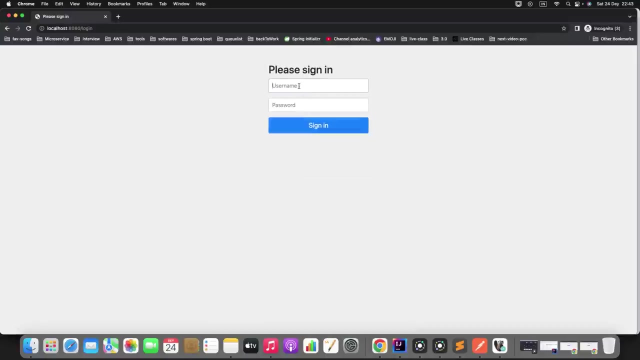 service filter, authentication provider, password encoder. in some case you also need the authentication manager all bin you need to create manually. okay, this is what the major difference. so it started. now i will just go and check the same url and i'll just go back here. um, localhost 8080, slash products, slash. all okay, enter the url now. first let me try with the john. 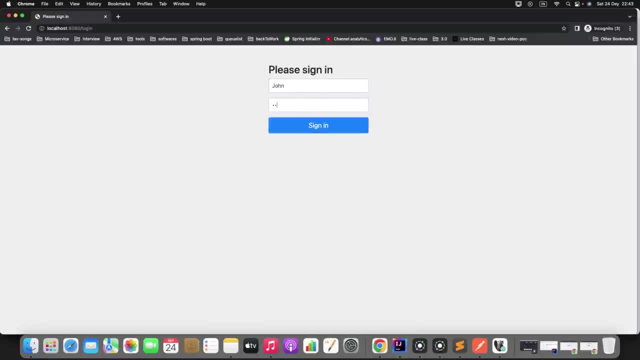 okay, john password is pwd. 2. i should get 403 error because john is not authorized to access slash. all endpoint because he is a user, is not admin, so that he can able to access it. let's see we are getting 403. this is the expected. now same endpoint I will try using. let me close this. I will. 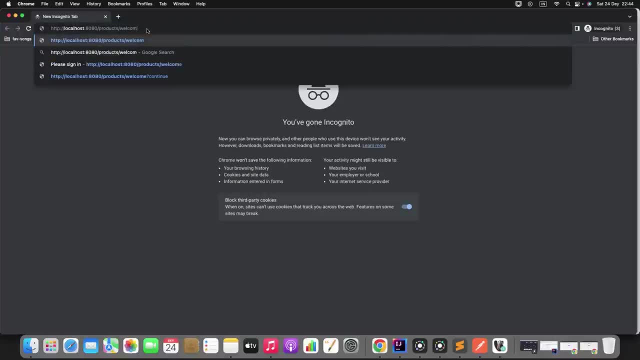 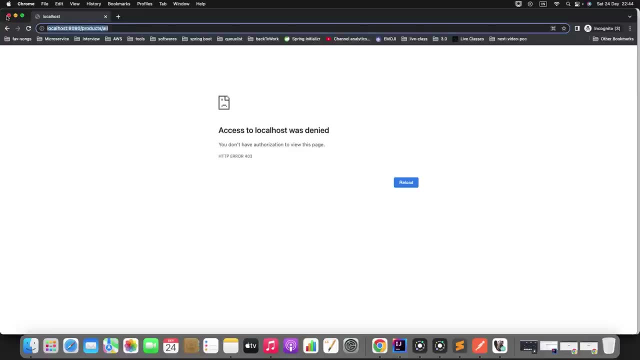 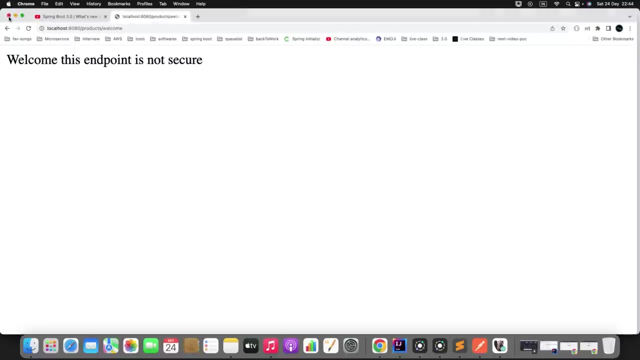 copy this. I will open a new in incognito mode. I will just pass all okay. oh, I need to close it again. command shift n. okay, it's already taking from my cookies what I will do. I will just quit this particular Chrome and I will just open. 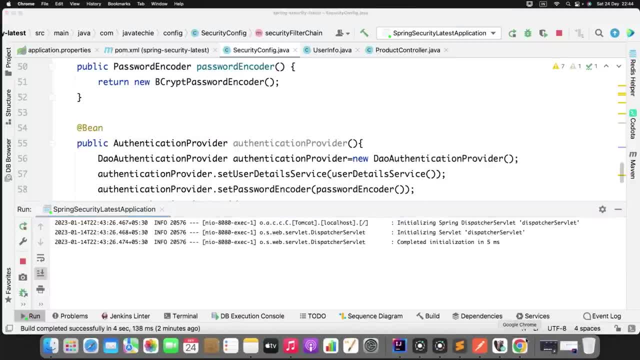 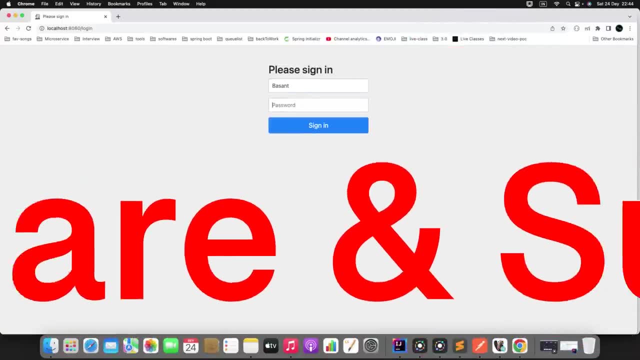 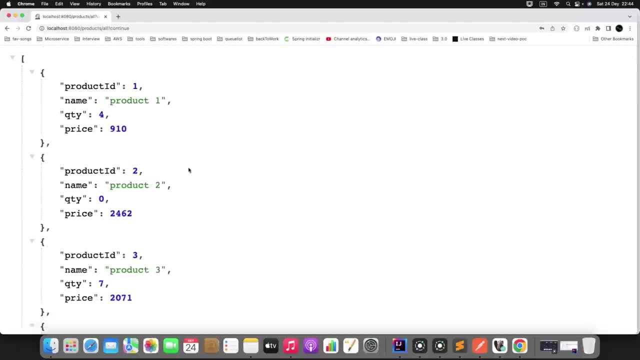 it even. you can try it out in your postman. okay, that's not an issue. it came now. I will give password. I will give PWD 1 sign in. okay, I can see the response here. right, because I am a admin, I have authorized to access this last all endpoint. okay, now John is try to access this last all. 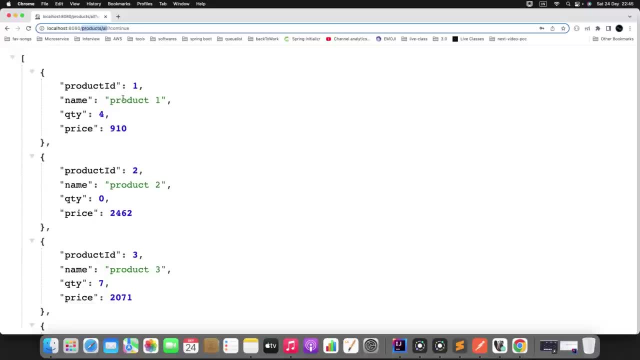 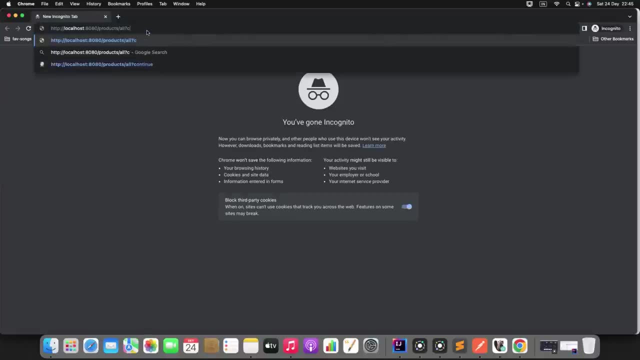 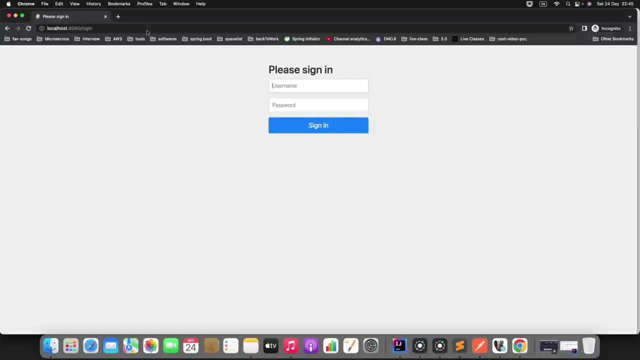 endpoint but he is unable to access because he is having the role user. now let me copy this. I will open a new. then I will try to fetch a single product by ID. this particular endpoint can be accessed by only a person or a user. when I enter, I can see a new endpoint of which I have to access. this particular endpoint can be accessed by only a person or a user. 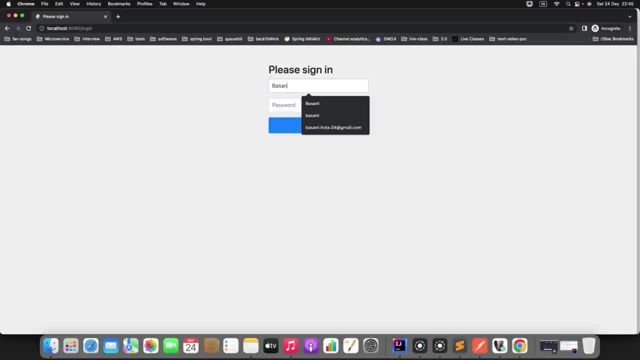 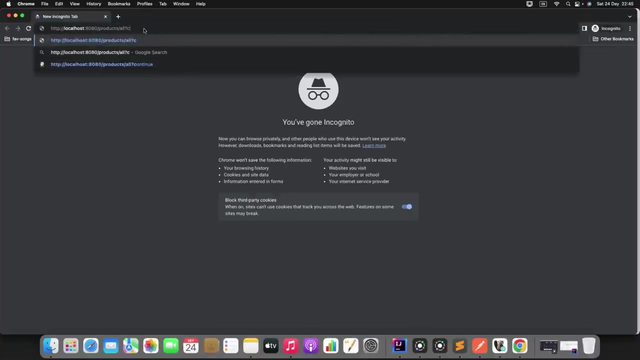 whose role is user. now i will try with the basant, because basant is admin, so it should not allow him to access right pwd1. i should get 403. that is the expected now. same. if i will try with, let me close this. i will copy this endpoint. i will open a new tab. i will just. i will just try. 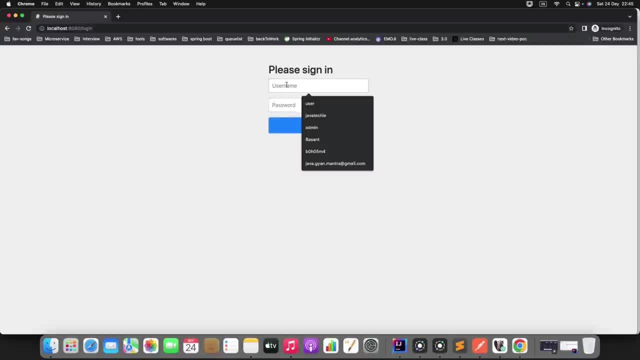 for the one. now it's asking me the credential. now i will give john, because he is the user he is having permission to access this endpoint. pwd1- sign in. okay, i okay. its password is pwd2, right, john. pwd2- sign in. john is able to get the response okay. so this is what we have specified.